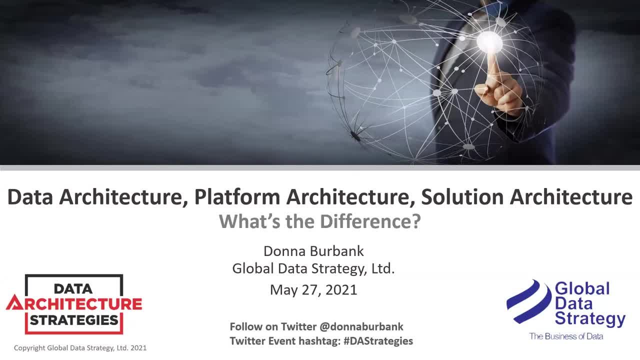 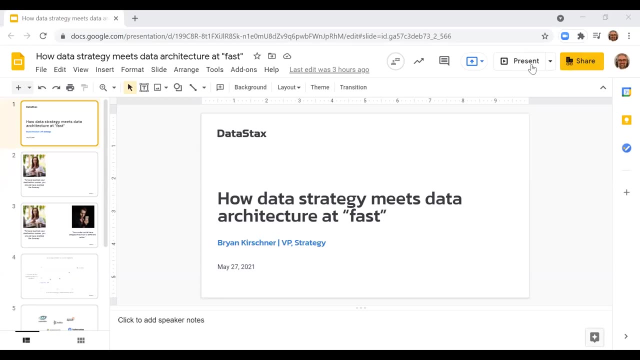 Monday is a holiday in the United States, so this will go out by end of day, Tuesday. So now let me turn it over to Brian for a word from our sponsor, DataStax. Brian, hello and welcome. Thank you, Shannon. I'm glad to be here to introduce this session and to share a point of view about 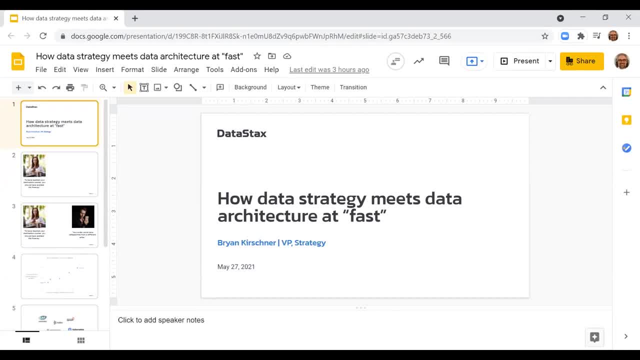 how we see data strategy meeting data architecture at quote-unquote fast. So without further ado, let me dive right in. You know architecture is an incredibly high-leverage discipline. Great technical architecture choices mean dozens, hundreds or even thousands of developers will be happier and more productive. But those choices 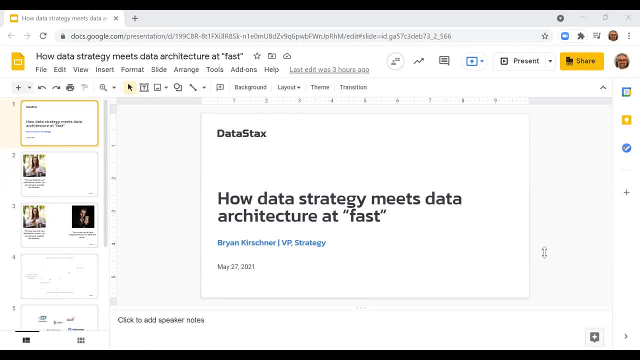 have got to be made in the context of business strategy because, at the end of the day, it's happy customers that are how organizations stay competitive and grow. So I want to spend this few minutes talking about what do we see a winning architecture needs to include: to make 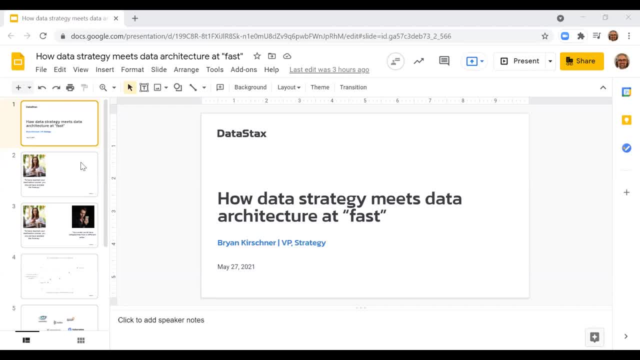 developers happy and productive at creating high-level data. So let's get started. So I'm going to start a little tongue-in-cheek. Imagine it. Oh Brian, sorry to interrupt, I don't see your slides in present mode. Oh sorry, It clicked out of present mode. That is odd. 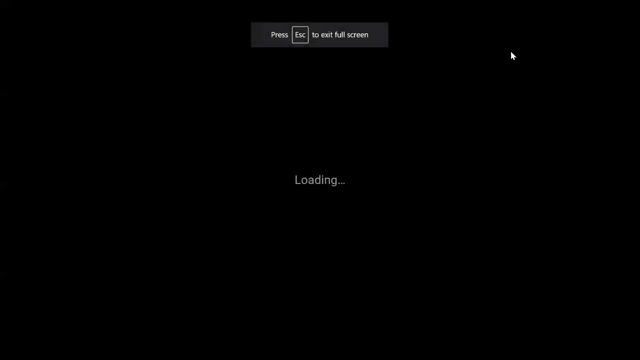 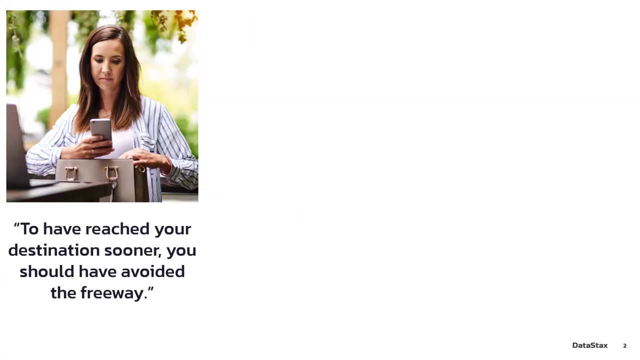 There we go. Okay, There we go. Sorry, It keeps All right. Thanks, Zoom. I think I got in the hang of it after the last four or two minutes. So imagine an app that says to reach your destination sooner. you should have avoided. 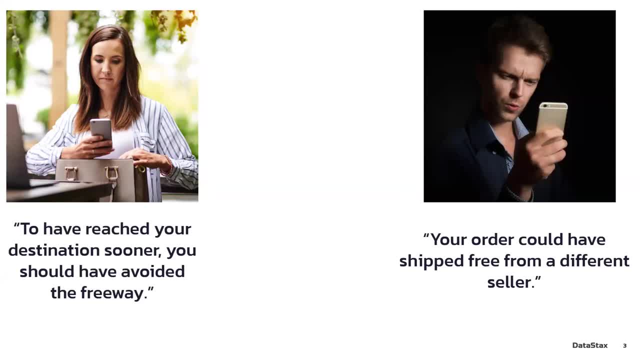 the freeway, Or after the fact, you should have avoided the freeway. So imagine an app that says to your destination: sooner you should have avoided the freeway, Or, after the fact, your order could have shipped free from a different seller. I'm being a little tongue-in-cheek here. 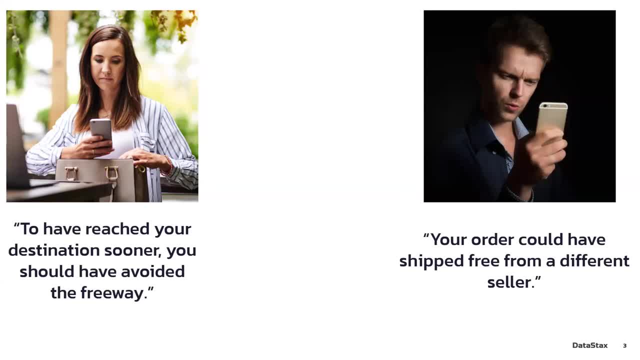 and we can all laugh Ha-ha. Who would ever ship such a broken, frustrating app? But the serious point is to satisfy customers. increasingly we need to ship apps that are smart in the moment, that do something useful with data to help us out. prevent a mistake. delight us. 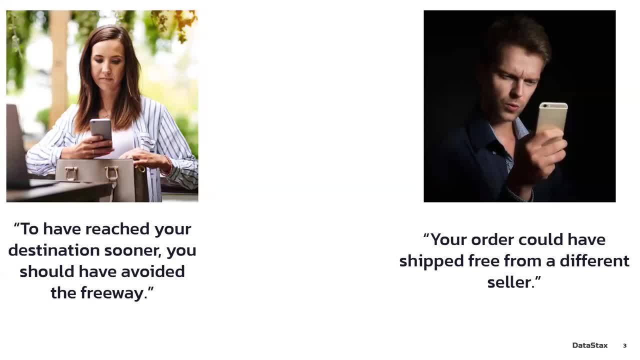 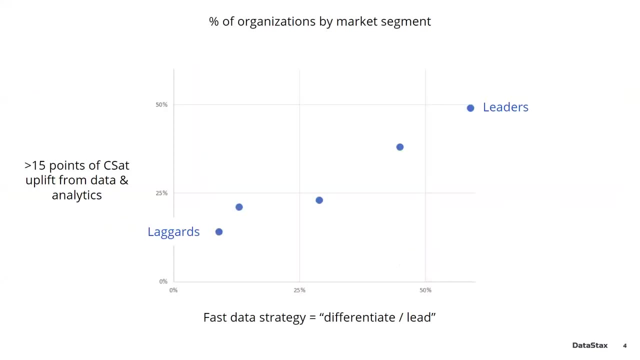 at the time it matters most, And that means latency for data. that's maybe in the milliseconds, maybe in the seconds, Maybe not in minutes and definitely not in hours and days. That's what developers need to be happy and productive doing shipping those smart, fast data apps applications. So we see the stakes. 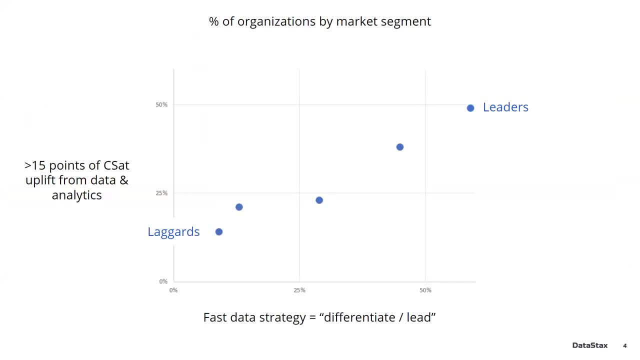 being really high. So we do a lot of benchmarking, not just to help us make decisions, but to help our customers make decisions, both business and technical, And this is data from a survey we just completed of over 500 organizations, And one thing we do with this data is we 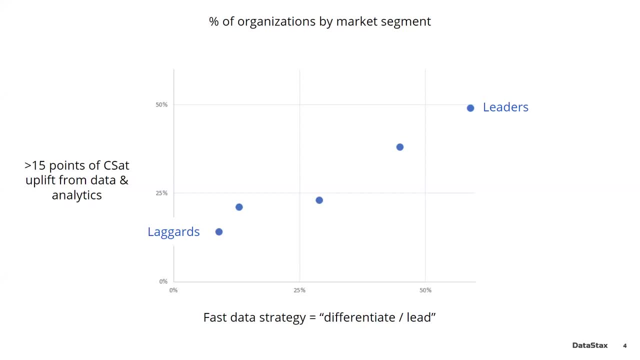 segment the market based on how the degree to which companies are leaning into change- not just changing technologies, but also changing their business, changing the culture and so on. And then we find roughly five segments with the top 10% or so we call the leaders. 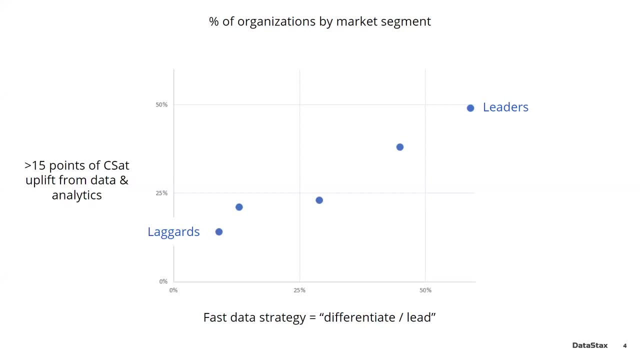 because they're the ones leaning furthest into change, And when you map out the behaviors and the outcomes, you see something pretty clear: The leaders are much more likely than the other segments to describe their fast data, And so what we're trying to do with this data strategy is differentiate and lead. 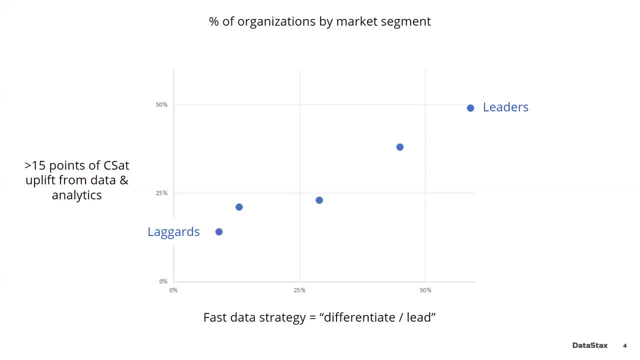 And they're also pulling ahead at driving customer satisfaction up by double digits using data and analytics. This should all seem pretty intuitive, because at the current moment, I think we can think about delightful fast data experiences going beyond Netflix and Spotify into great curbside pickup, into bang on delivery time prediction and so on, particularly over the last year or so. 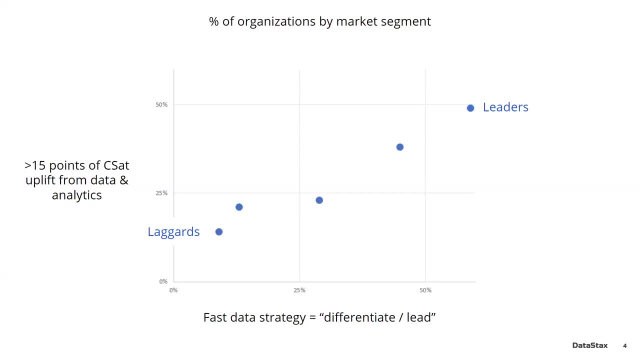 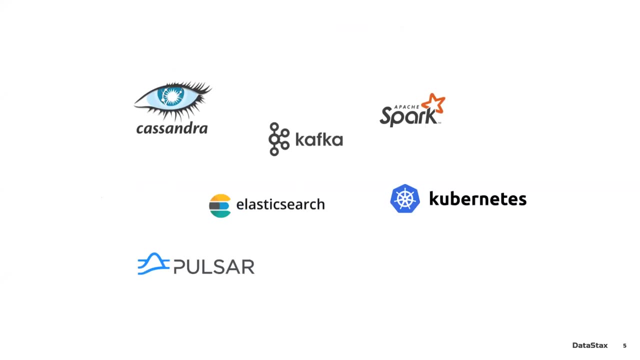 But we think this is a generalized and important pattern. So what are the implications? Well, again, in our data, we see the leaders much more likely to be using these technologies in combination, And you can read great technical blogs by folks at Intuit, Condé Nast, Walmart about how and why they 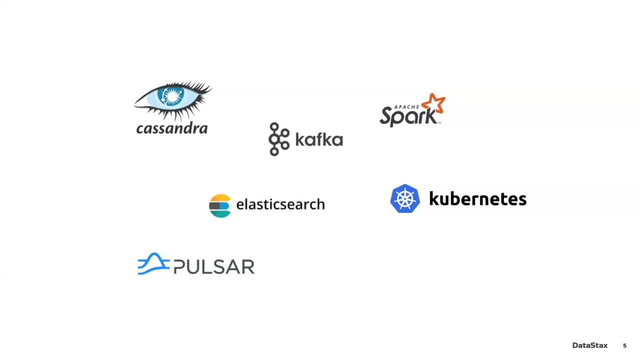 chose some of these technologies in concert to deliver these great, fast data experiences. Now, the key point here is that this shouldn't be a random grab bag of tools. if we're talking about architecture and we're talking about platforms, So the meat of the matter is: we'll get to. how do we think this coheres as part of an architecture and part of a deliberate approach to making developers happy and productive? 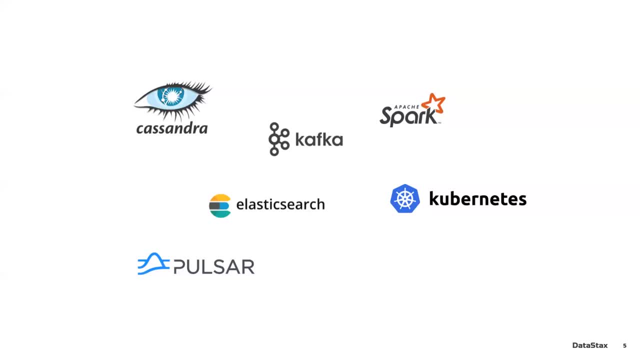 I want to say I'm sure people are experiencing some pain now that I didn't present this in a logical architecture. I know everybody's probably saying why isn't Kubernetes at the bottom? But we'll get there. So here's our point of view. 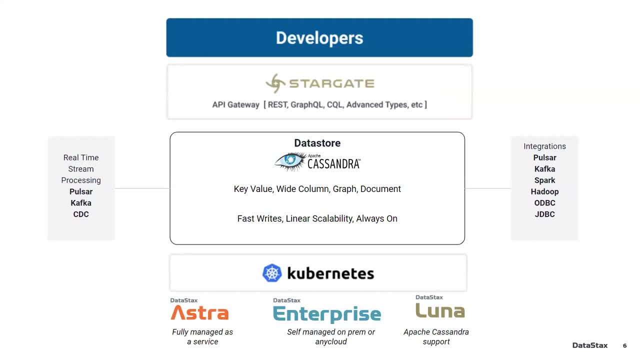 On the stack for fast data. I'll go right to the middle, And we love Apache Cassandra as a fast data store. By its nature, it's awesome at fast writes, it scales linearly and it's highly resilient- always on, never loses data for applications that are critical to customer satisfaction. 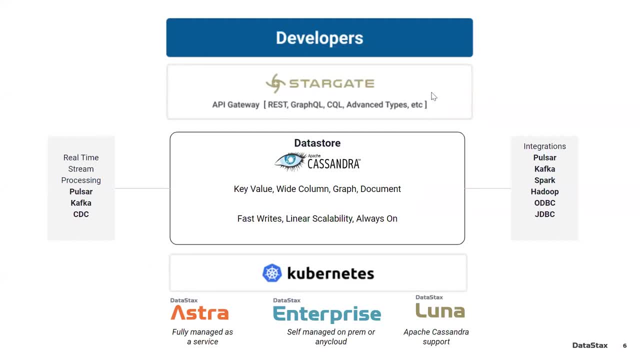 That's great. It's also multi-model, So when you need speed, it can function as a key value store. It can be used to build a graph database or a document database, And it works extremely well with streaming And if you look at design patterns for some fast data apps. once you're using streaming and stream processing, you essentially need a data store that can keep up. 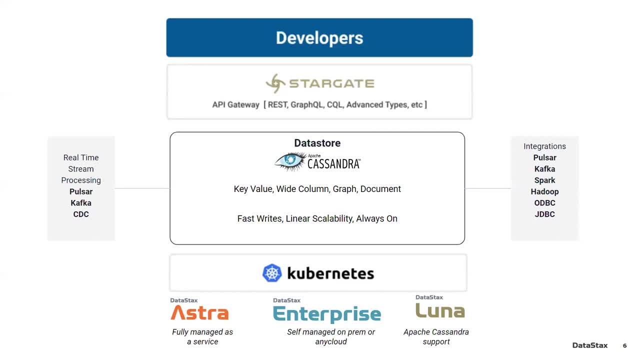 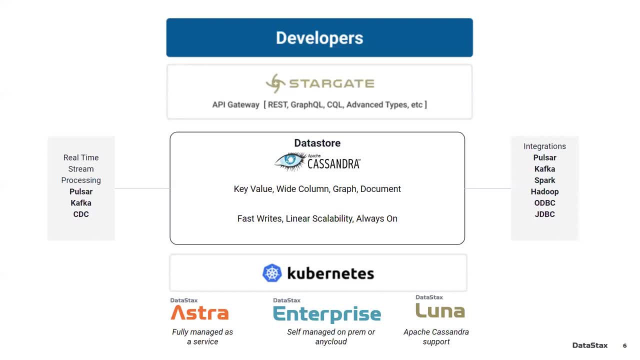 So that's the whole point. If you want to be happy and productive developers, don't just offer them a multi-model data store. Enable them to interact with that data store with familiar APIs. Abstract away the details of the database. So we've bundled up developer APIs into an open source project we call Stargate. 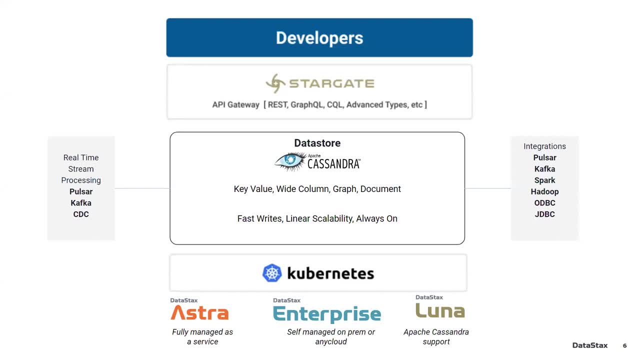 And so folks can interact. developers can interact with Cassandra through REST APIs, graph APIs or a document API, for example, Not having to know anything about the guts of the data store, Just using their familiar vernacular. And, of course, if we think about modern apps, particularly fast data apps, we think they should run on Kubernetes. 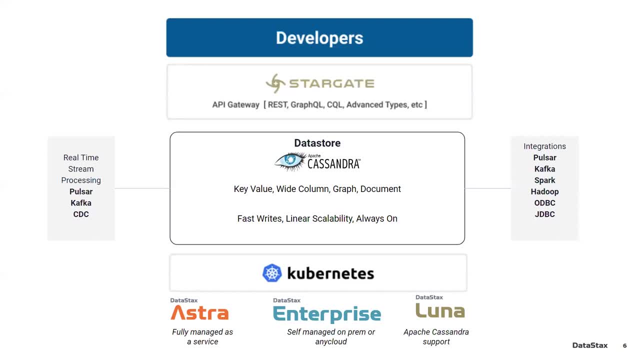 And this probably can make some intuitive sense- right, Marrying horizontal scalability for compute to linear scalability for data. So we think that's a very exciting and important approach and stack to have inside a data architecture And good platform, thinking about how you extend its relevance to make developers happier and more productive, delivering fast data apps. 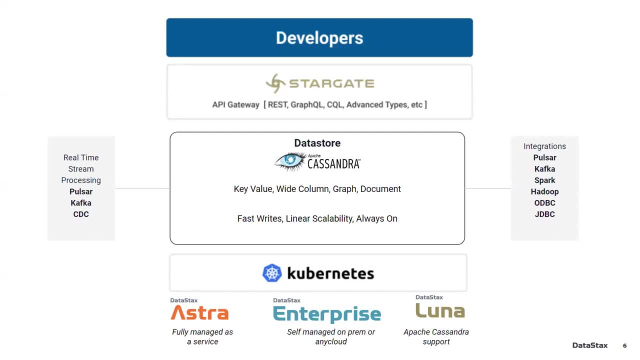 Finally, as a company, here's how we walk the talk and put our money where our mouth is. So, as a company, we operate Astra, which is Cassandra, as a fully managed service running on Kubernetes, And we've done the engineering work to also make it function in a serverless fashion. 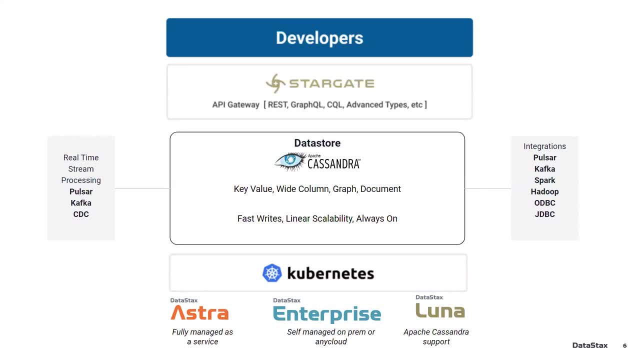 So Cassandra, by its nature, is always able to scale elastically up. Astra can scale elastically down as well, So you're not paying for overcapacity. We offer DataStax Enterprise, which is self-managed commercial version of Apache Cassandra on-prem or in any cloud. 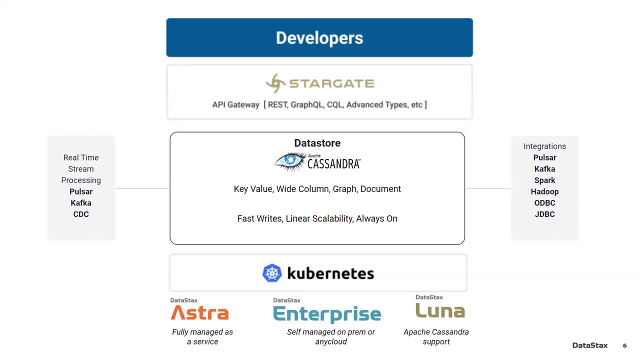 We think most companies, we know most companies who are excelling building fast data apps are also doing a hybrid cloud architecture and multi-cloud architecture. And finally, because you know, at the end of the day, great decisions about architecture and platforms are much more likely to happen if you have intimacy with the underlying technology. 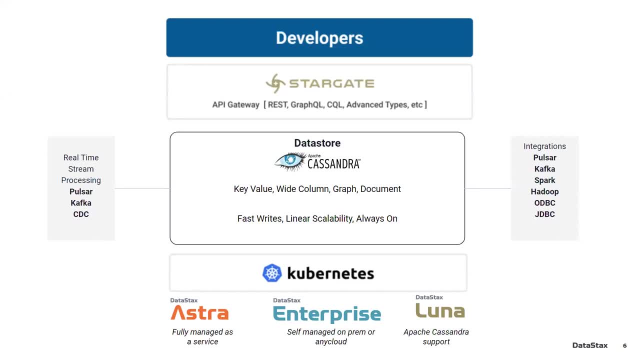 And with customer use cases. We also support Apache Cassandra- open source Apache Cassandra. So you know I'm glad to have these few minutes to share what we're excited about, where we think data strategy and architecture combine to have a great data store for fast data apps to make developers happier and more productive delivering those. 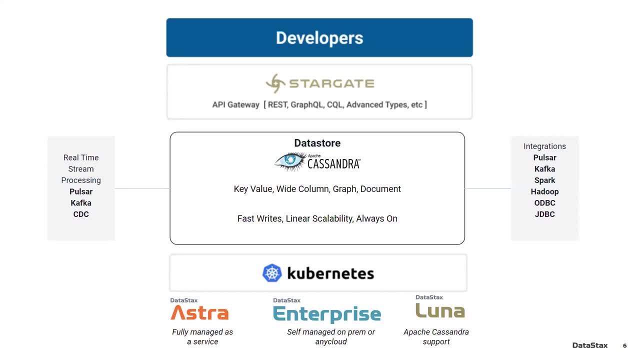 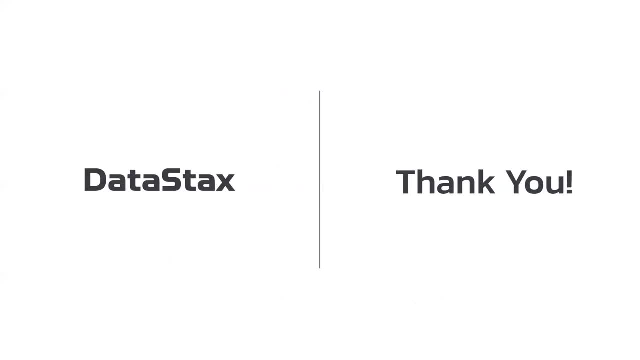 And we're hard at work. If you want to make this a reality in your organization, please let us know. We hope we can help So with that. thank you very much. Unfortunately, there is a very hard constraint on how leveraged I can be. 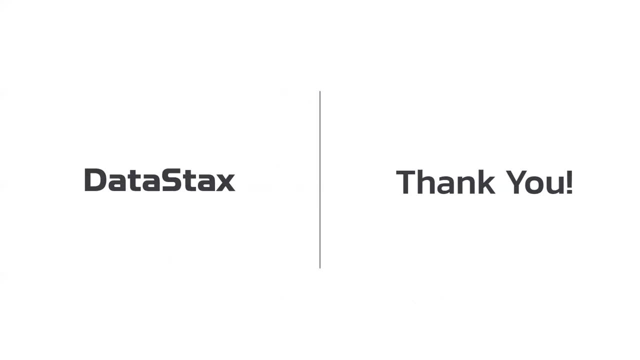 And I do have an obligation that's going to call me away at about the half hour. So if you do have questions, don't hold them to the end. Please plop them in the Q&A and I'll do my best. Thanks so much. 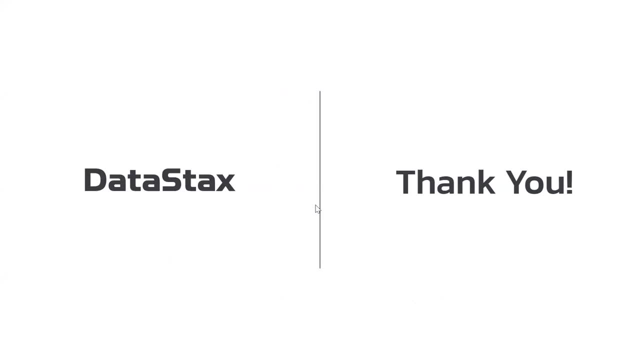 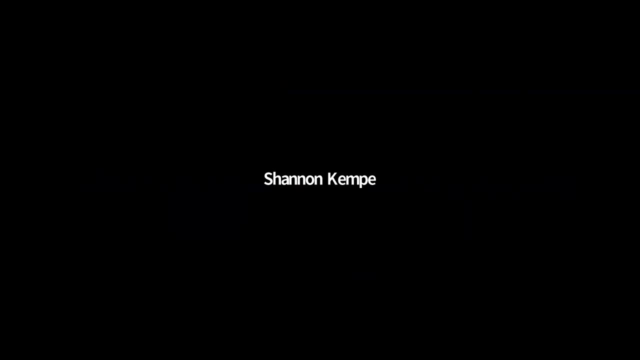 And I'll hand it back to you, Shannon. Brian, thank you so much for this great presentation And, as he mentioned, Brian will be hanging out a bit to answer questions in the Q&A panel. If you have questions for Brian Or about DataStax. 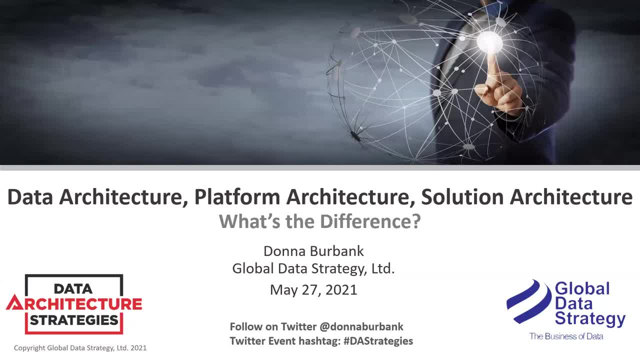 And thanks to DataStax for helping make these webinars happen. Now let me introduce our speaker for the monthly series, Donna Burbank. Donna is a recognized industry expert in information management with over 20 years of experience helping organizations enrich their business opportunities through data and information. 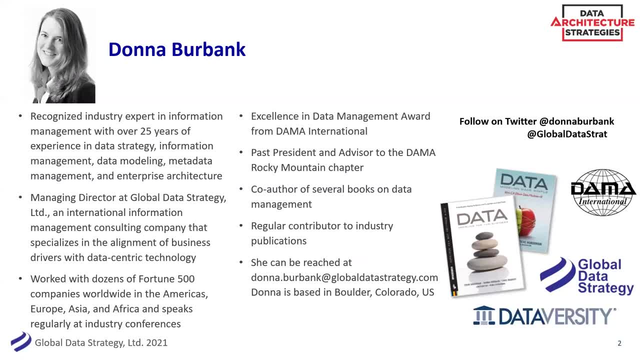 She is currently the managing director of Global Data Strategy Limited, where she assists organizations around the globe in driving value from their data. And with that, let me give the floor to Donna to begin her presentation. Hello and welcome. Hello, Shannon. Thank you. 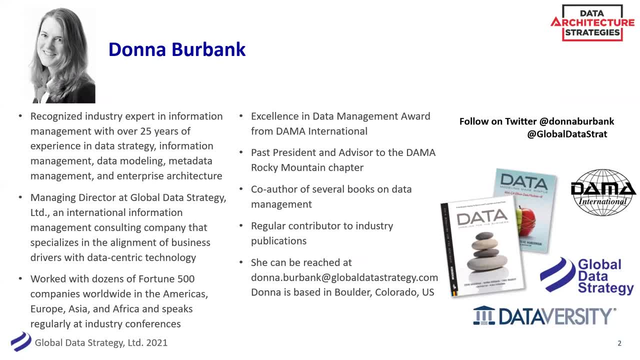 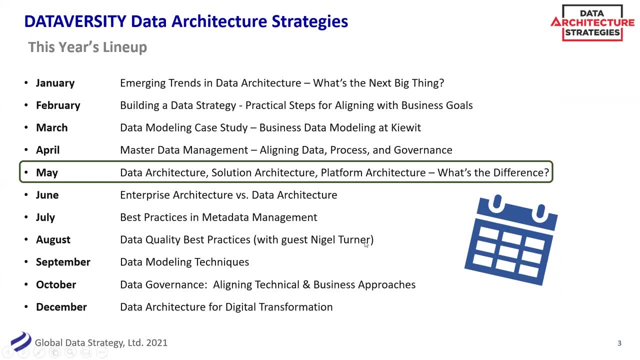 Always a pleasure to do these webinars and see some familiar names and faces on the attendee list. So thanks for those who- a lot of you I know- attend every month, So appreciate that. So, on that note, if this is your first time joining a Dataversity webinar or a webinar in this series, just a call out that if any of those previous topics that you see earlier in the year are of interest to you- there was an interest in case study, for example- 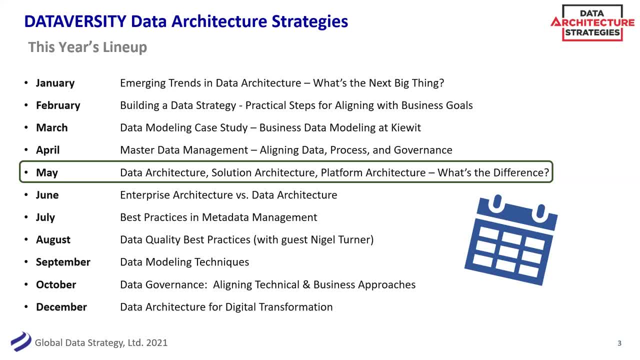 earlier in the year. These are all available on demand on the Dataversity website as well as ours, But Dataversity does all of these webinars Excuse me, And I hope you can join us for a few of the upcoming webinars. 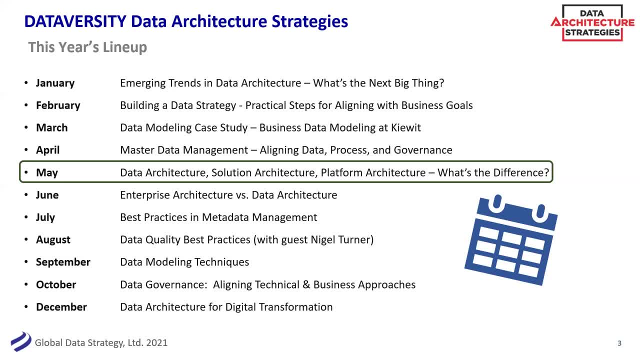 Next month is sort of a sister webinar to this. We'll talk about enterprise architecture versus data architecture. As Brian mentioned, there's a lot of different flavors of architecture and we like to be very specific as architects, So there's a little bit of a series within a series there. 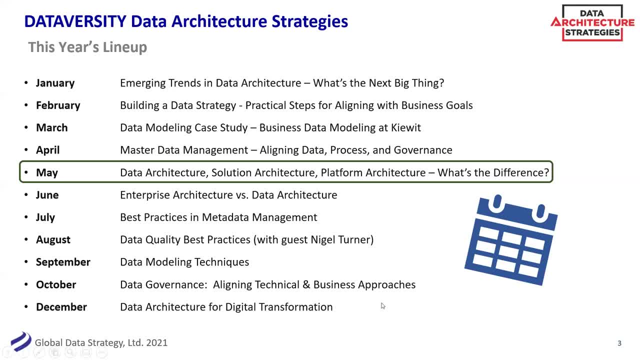 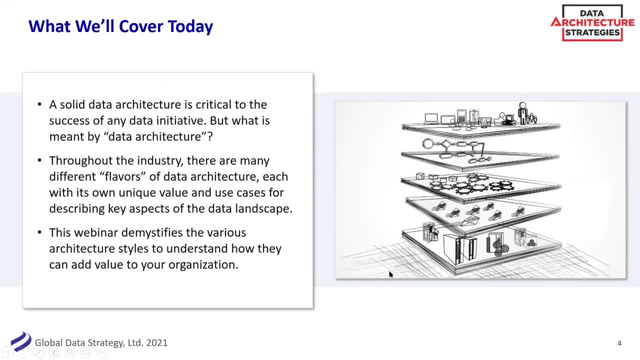 As well as some other topics throughout the year And, as always with Shannon's webinars, they are free and open to everyone, So pass them along. But today we are going to cover some of the flavors of architecture, And it can get confusing. 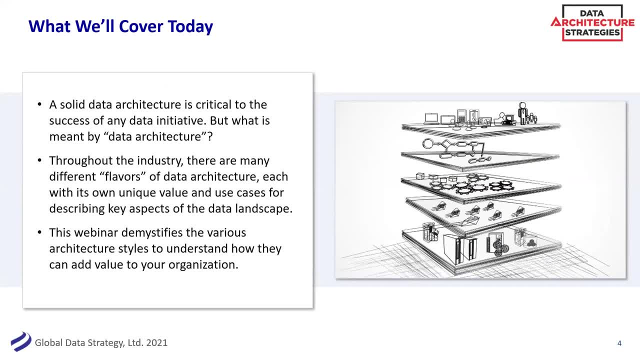 I mean, this series really focuses on data architecture And I will talk of the various architecture types in the title: platform and solution architecture. But just a caveat there that we will do it in the lens of data, Because this is sort of a data series. 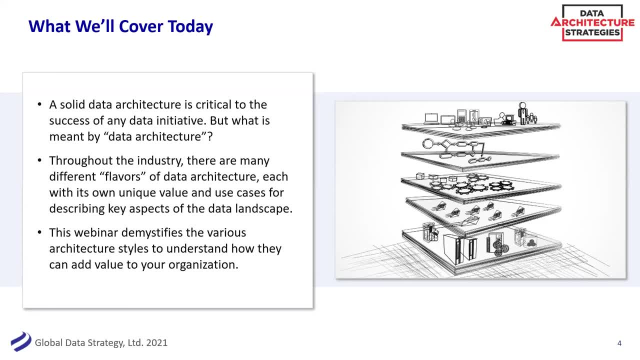 One could have a whole webinar series just on platform architecture or solution architecture, But we're going to kind of take it from the lens of a data architect, which I think is a lot of you guys on the call. And then, as always, what I try to promise and deliver here with this webinar series is that last bullet of kind of demystifying it. 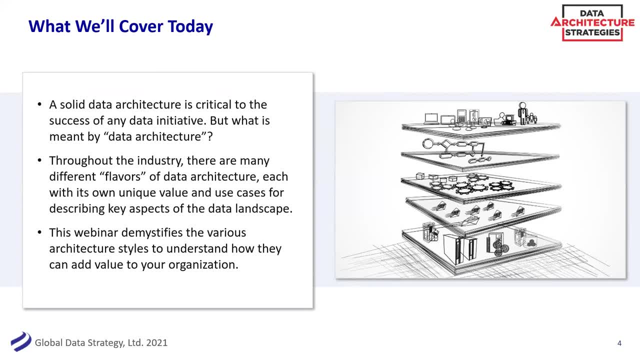 And we'll get a little into this. All of this can get very academic very quickly And I think it's important And I think what I try to do in life, and hopefully in this webinar, is to try to get down to the so what. 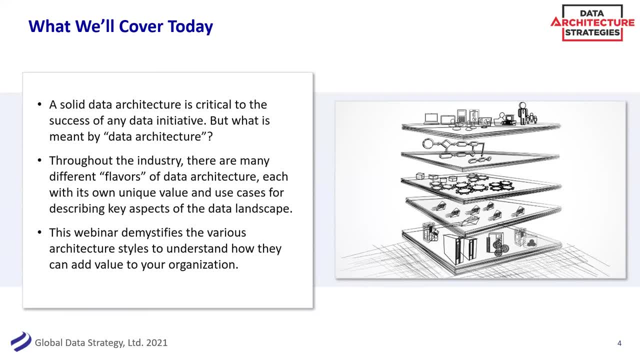 And I think Brian did a good job of that as well- of, yeah, there's a lot of cool architecture out there And a lot of us will learn out really quickly to get into it, But what's the so what at the end of the day? 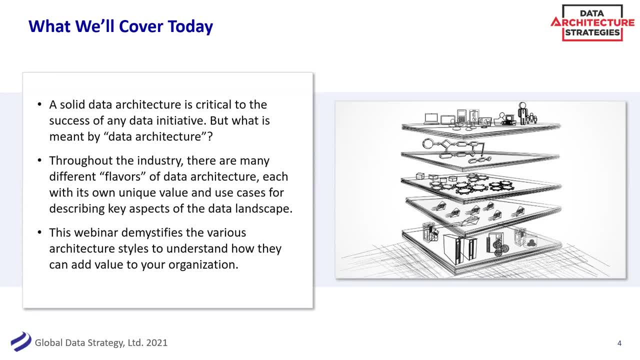 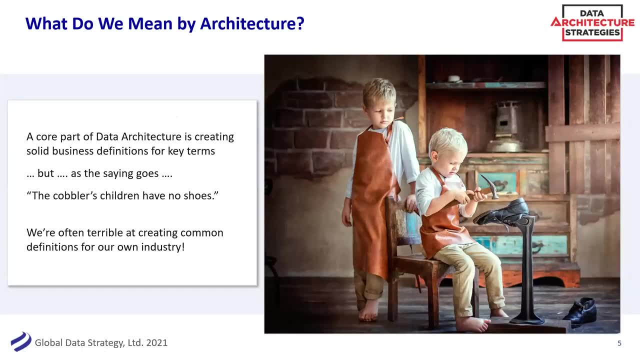 How is it going to help our customer, How is it going to help our organization? So I'll try to throw that lens on it as well, because there's just so much we can learn in this environment And on that topic. we in data architecture, especially more on the business side of data architecture- 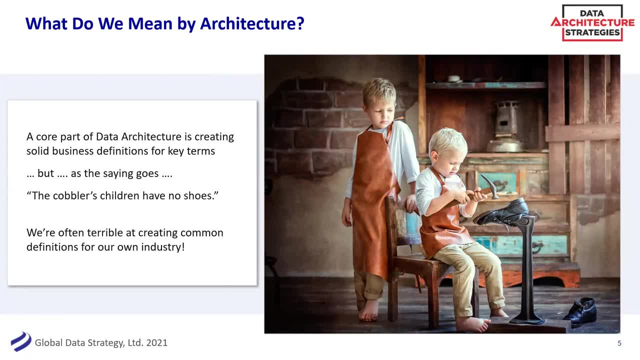 love our definitions. In fact, that's what a lot of us do for a living. We create business glossaries and data models, But what's that saying? The cobbler's children have no shoes. And I am often just flabbergasted of how poor we are as an industry on what some of these core terms mean. 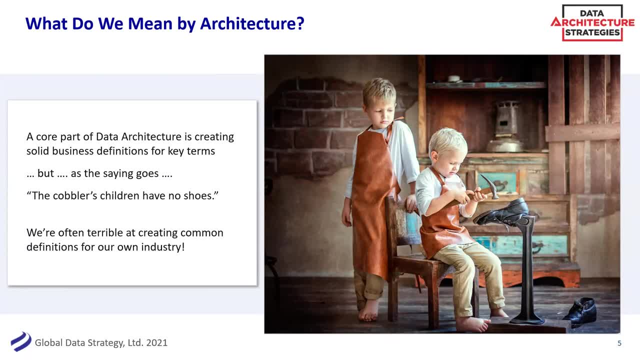 What do we mean by architecture? What is the difference between a platform and an architecture and a data architecture? We did a webinar last year on titles and it was similar. What's a data architect? How is that different from a data engineer? 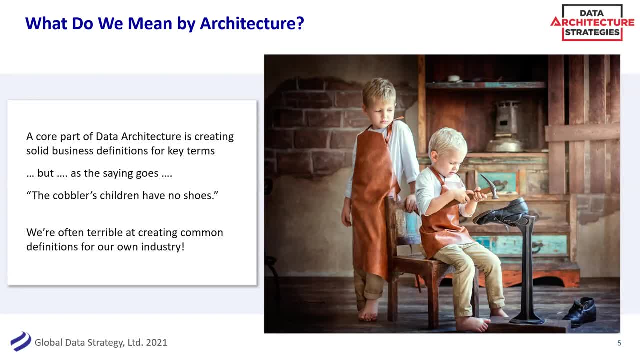 And there is a lot of overlap between these. But as architects I like to be sort of clear and kind of get down to the use cases and some definitions. So I will offer you some. I'll also offer you some of the different opinions that we see out there. 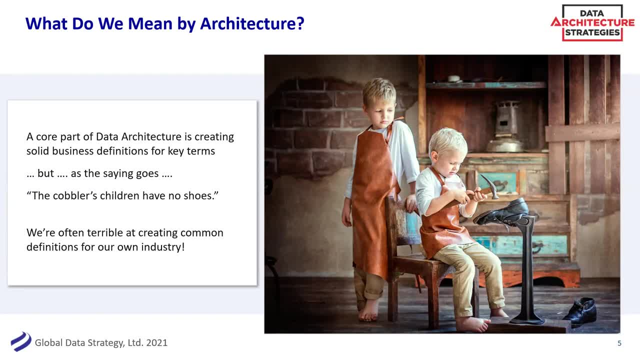 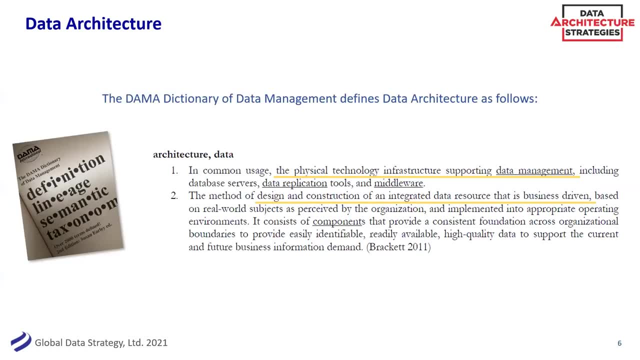 But hopefully we'll get better as an industry, but probably not, I think. we love to argue about some of this stuff sometimes, So just a little intro there. So here we go with our definitions. So I'm sure a lot of you are members of or are very aware of the DEMA, or DAMA, depending where you live in the world. 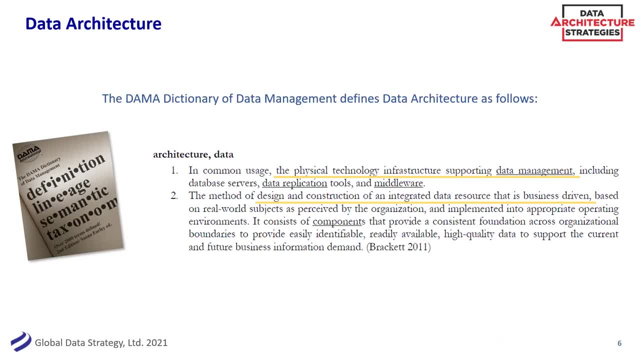 And there's a dictionary. There's a dictionary of data management that did attempt to put some shoes on the cobbler's children and go with some terms, So I would be remiss if I didn't use this for the data architecture definition. 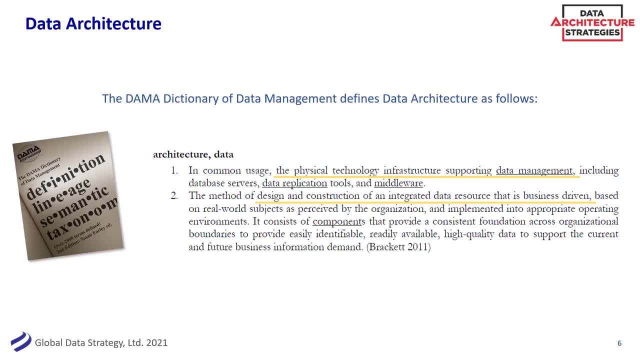 And what I do like about this definition. I could probably argue about each one of these for a whole webinar, but I will not. I'm learning to filter, So what I like about this one is it does separate out the physical data architecture, which is number one, the physical technology, and also heading towards data management as a wide area. 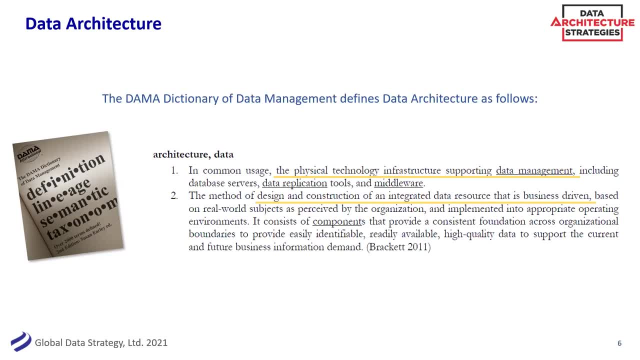 So I think that's a big part of the definition And I think that's why this definition is so important, because it's a big part of the definition of data management as a wider practice from the business data architecture, And I think they are separate and equal and related. 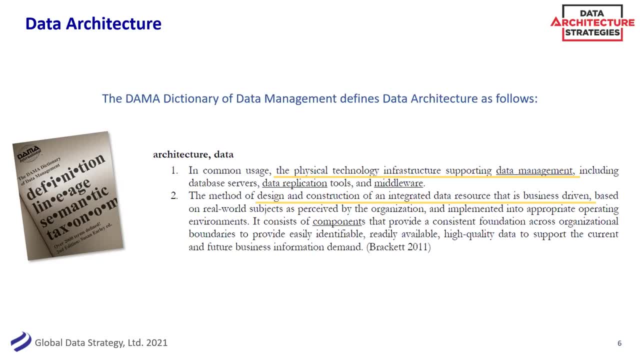 And we'll kind of go through that. But when you want to keep those separate and really understand that they are disciplines in and of themselves, So this one I'll go with. There's other definitions out there, But this is probably a solid one we can go with when we're talking about data architecture and the different flavors of that. 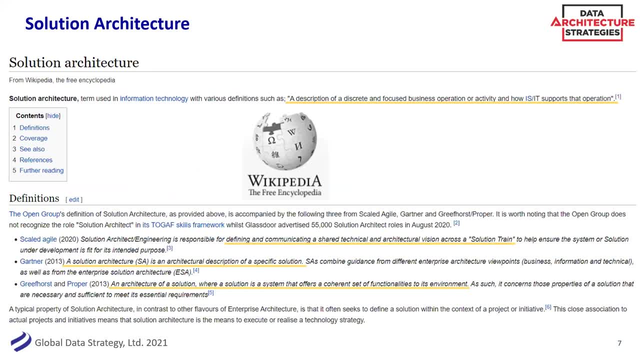 So I'll go with the data architecture. There was a whole bunch of those, So I went to the good old Wikipedia, which you know. there's pros and cons of that as well, But you'll see several from Gartner, from Open Group and TOGAF. 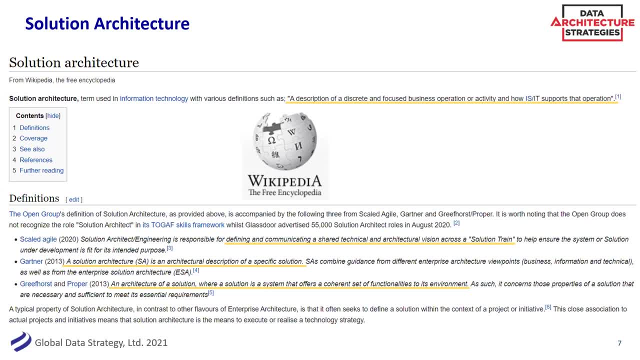 But when you really look at it- that's- I guess it's been in the name right- You're defining a solution or a particular application or an architecture. The one I sort of liked was Gartner's: the architectural description of a solution. 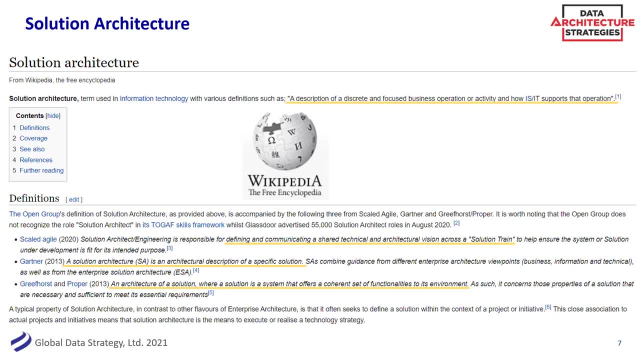 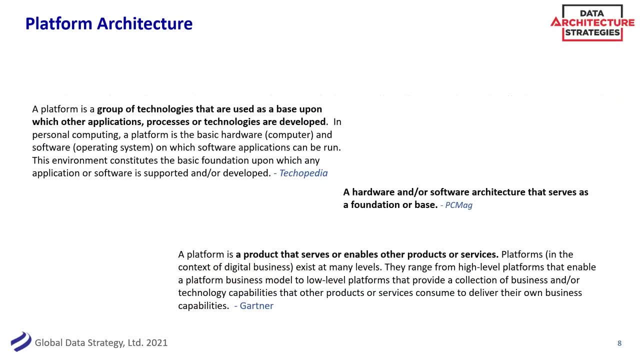 And really getting, excuse me, all of the areas around that. Right When we go into the platform- and that's sort of more what Brian was talking about, where we're getting into- how are we creating that core platform around the software, the hardware? 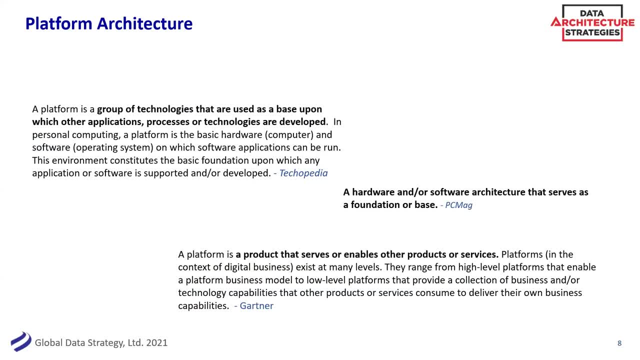 and more in the olden days with the hardware that really enables some of those other products or services. So here's some from Gartner, from Tickipedia, from a few, And then they sort of all were kind of starting to go around that similar idea of it's really that enabling foundation. 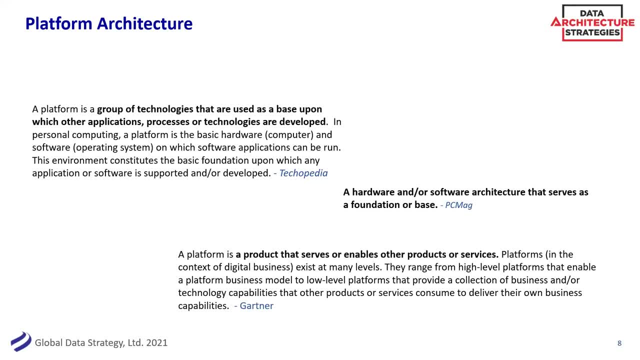 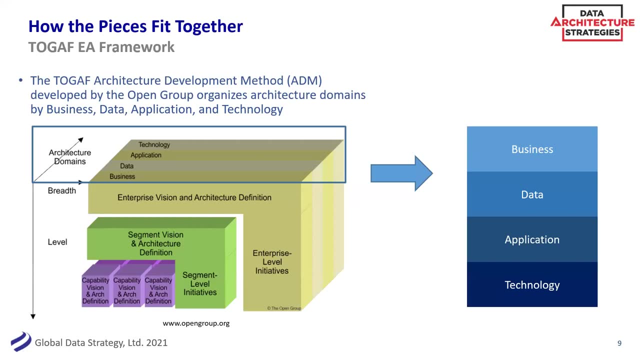 On which those other architectures sit upon, if that makes sense. So maybe this was helpful. Maybe this just made it all more confusing. There's a lot of words on these slides. When we talk about architecture, it's often good to think about enterprise architecture, which will lead into next month's webinar, which is a whole topic on that. 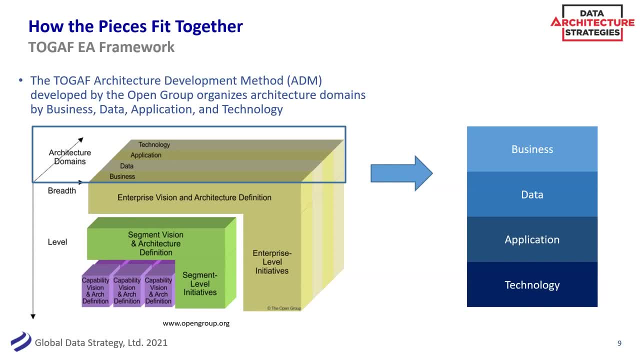 So I won't get too detailed into all of the broad areas of enterprise architecture. But TOGAF is a very common framework around enterprise architecture And when they that sort of top part that's in the box, I sort of like how they broke it out. 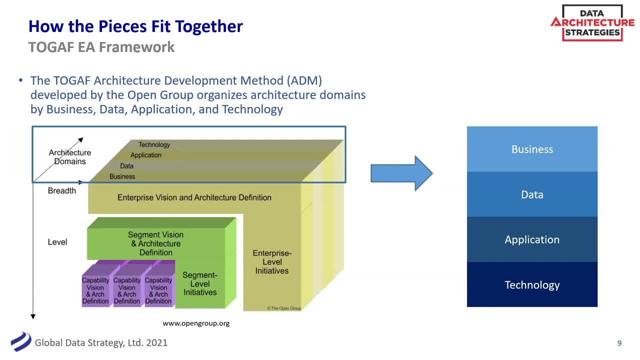 And a lot of areas do this, but this is a common one I thought I would touch upon That really breaks out these various architecture domains that are in the title And their way of looking at it was sort of business, data application and technology. 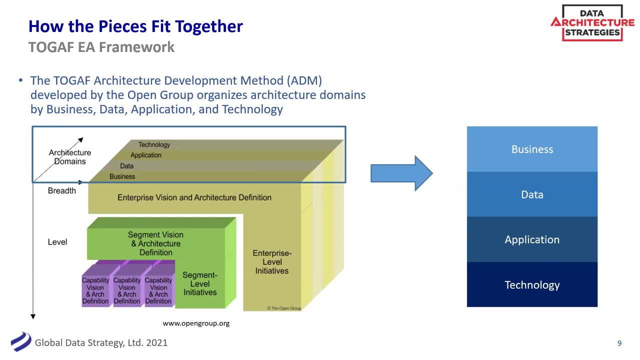 Maybe I flipped it on its head, But I kind of saw those in a similar way of. you know, the business is what's driving what, And that's why we're doing this. I might have put data on a different layer, but again we could argue. all of these 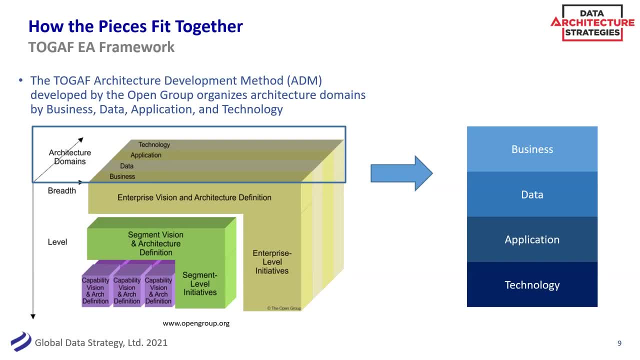 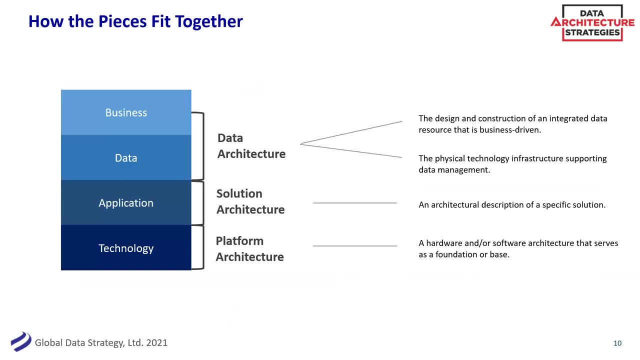 And then you have the applications that may use the data and then the technology that supports that. So, as kind of a framing mechanism, I thought that was a good and helpful one to go with. So then, how do those pieces fit together? to use the words in the title of this webinar, how I see it is when we look at data architecture. 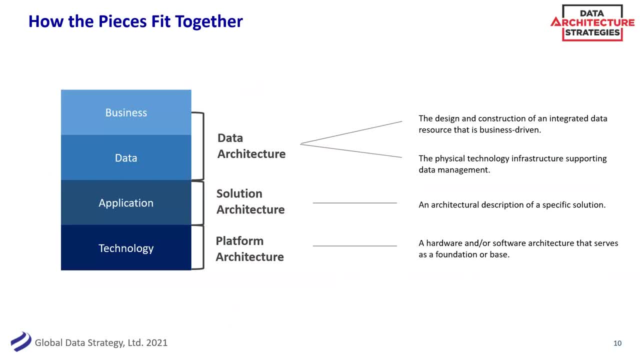 And again, you could probably say this With solution and platform as well. But I see data architecture in particular as that bridge between business and data. So if we go back to that DEMA definition, I think they correctly sort of said there's two types at least of data architecture. 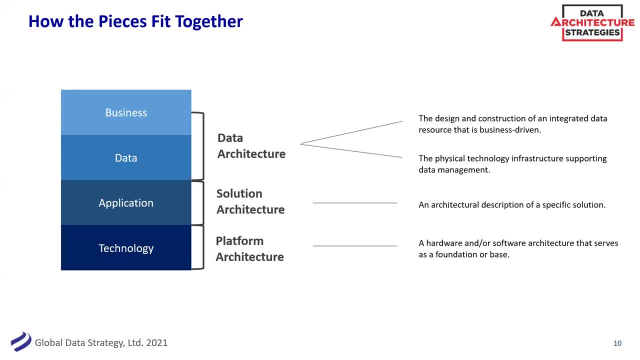 That business and I took these definitions from the previous slides and sort of mapped them onto this So that first, the business data architecture Is an integrated data resource that's more business driven, Which then ties into more of that physical data architecture that really talks about the infrastructure and the data management and the more technical sides of that. 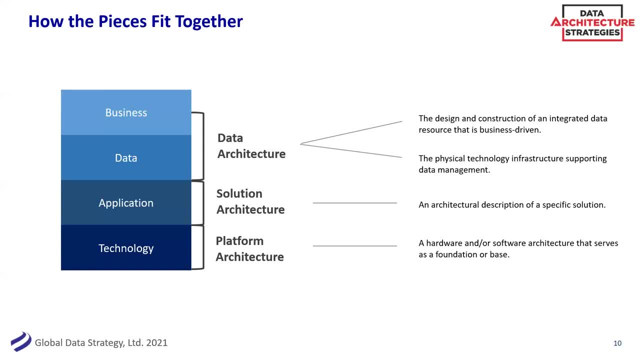 But of course they should kind of link together And then the solution architecture is describing, probably by definition, a particular solution, And then the platform is more of that foundation or software architecture or architectures and sort of how they fit together. Is it on-prem? 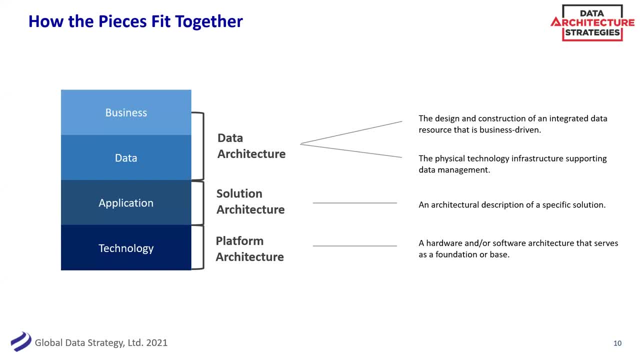 Is it in the cloud All of those types of decisions? So hopefully that was helpful to kind of take those different layers that were shown in the previous slides and kind of map them a little bit to the different applications. So what do we build from this? 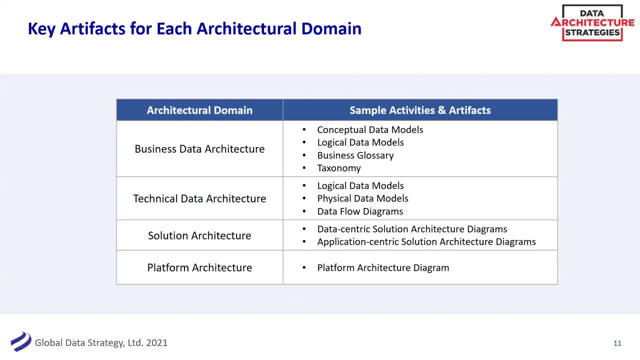 And this is only a subset. I'm sure there will be comments and thoughts that I'm missing something. I probably am. But just to kind of box some of the things that we do on a daily basis, especially the architects on the call and kind of which domain they would sit in. 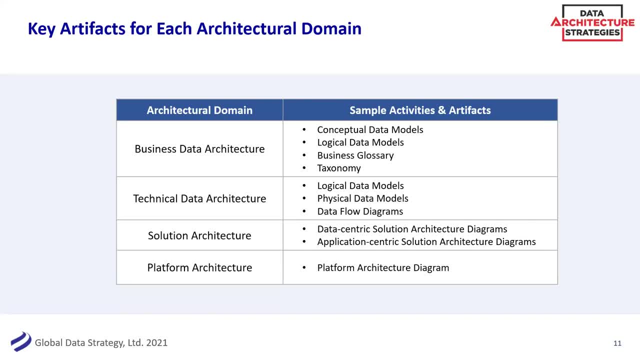 So business data architecture. Maybe I went a little heavy on those compared to the others, But I think that may be one that I see maybe is neglected and shouldn't be in some organizations. So I'm sure a lot of folks on the call are familiar with data models. 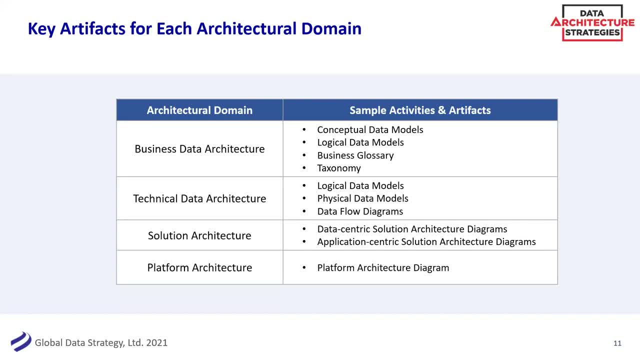 So I would put in the business data architecture things like conceptual data models, logical data models- Some people go a little higher than conceptual and maybe call that an enterprise or a subject area or different names for that- But that sort of business-centric data model. 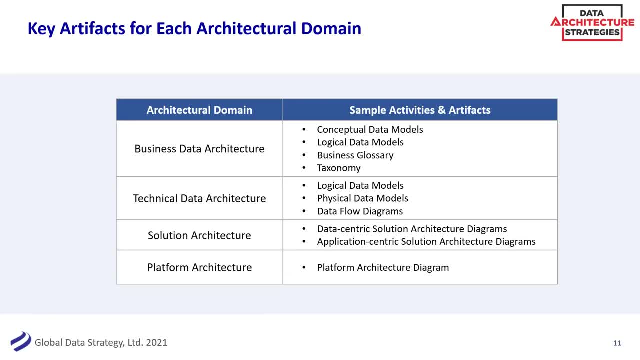 I think a business glossary. you could argue: is that really an architecture piece of architecture? I think so, because you're architecting the definitions of the business. A lot of those glossary terms come from data models And I think again kind of a related technology or architecture is a taxonomy. 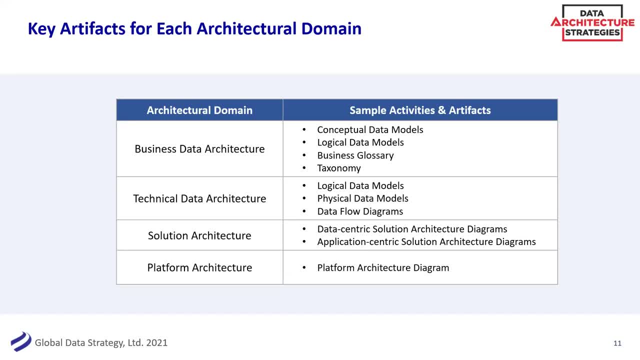 And I find- and we all have our different camps in the organization- sometimes there will be a whole taxonomy group that's separate from the data architecture group or separate from the modeling group. And when you think of a taxonomy, that's really a modeling of words and terms and concepts that maybe it's not in a what we might call a data model or an architecture diagram. 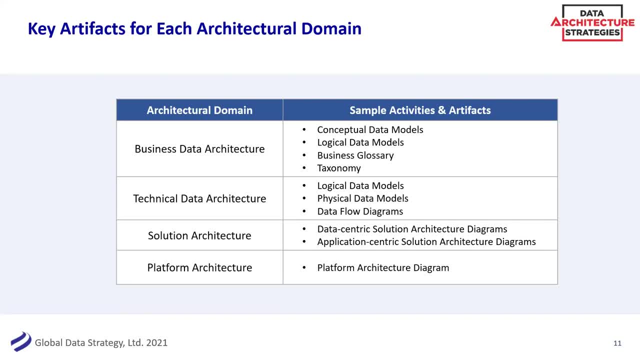 But there's certainly an architecture and a hierarchy within those. So I kind of threw out some ones that maybe wouldn't come top of mind. Some probably very much are, But I think those are in the business data architecture because they're architecting the business, the data around the organization. 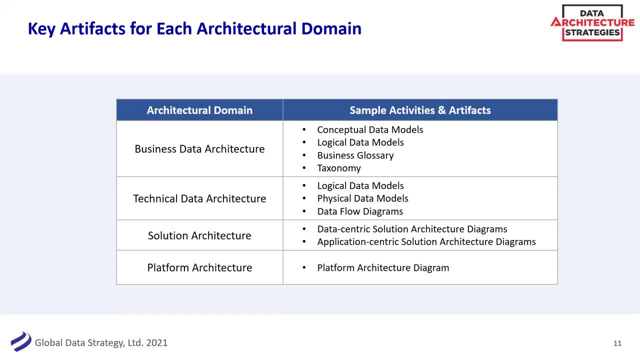 I didn't want to go too far. We'll talk about it again at the end. But when we do talk about enterprise architecture, there's a whole business architecture on top of this. How do you model the business, the capabilities, the business drivers, the- so what, around the business itself? 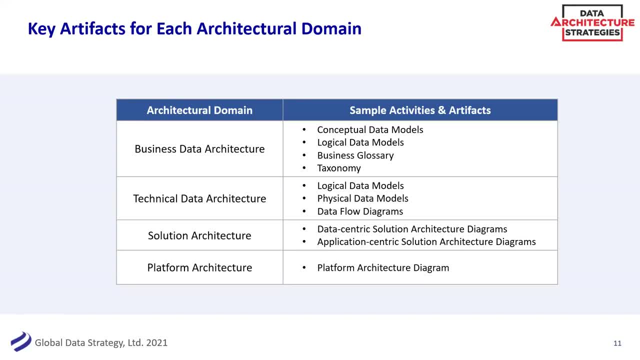 But again, that's the whole webinar in and of itself, As we go into the technical data architecture. that's where you get into things like your physical data models, your data flow diagrams. I put the logical data model in both categories, the business and the technical, because I think that's to me the handshake. 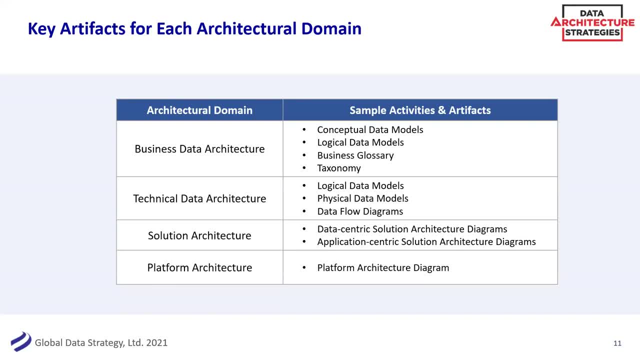 Between the business conceptual- sorry. a logical data model should have business rules in it. It should use terminology that's fairly business centric And you're also getting towards some architectural decisions. How do we group the entities? What attributes, what data types might we have on that model? 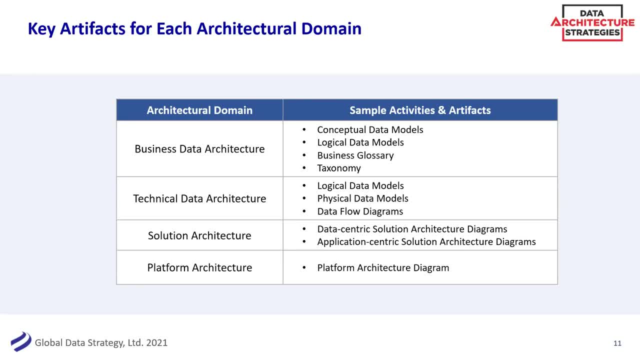 So that one to me lives in both camps. As you get into more solution and platform architectures, they sort of have their own diagram. As Brian said at the beginning, they're all architecture diagrams And one of the reasons I kind of hosted this webinar is I know, when I go into a consulting engagement- full disclosure, that's what I do for a living. I see a lot of different organizations. 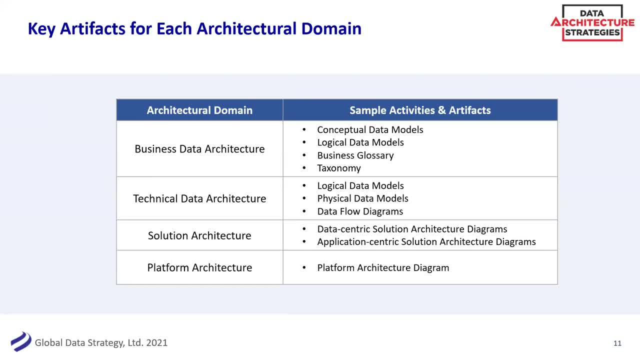 Often there's this whole little, I don't know, awkward piece in the beginning. when we're again back to that cobbler's children have no shoes. We're trying to describe the type of diagram we're looking for. Is there a solution, architecture for this? 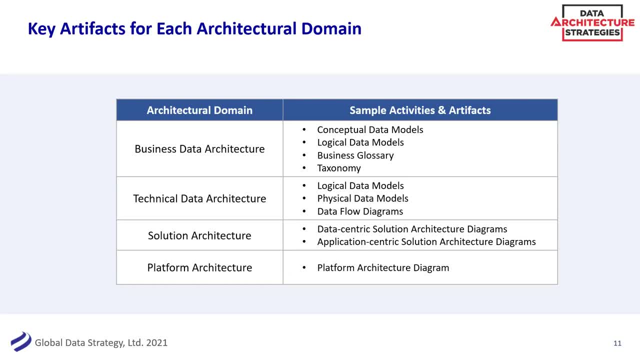 Do you have a data model? What do we mean by that? What do we mean by a data model? Is that a data flow or is that a solution? architecture, And again just trying to get at some core definitions of: there are a lot of architecture diagrams that have boxes and lines on them, but they all have a slightly different purpose. 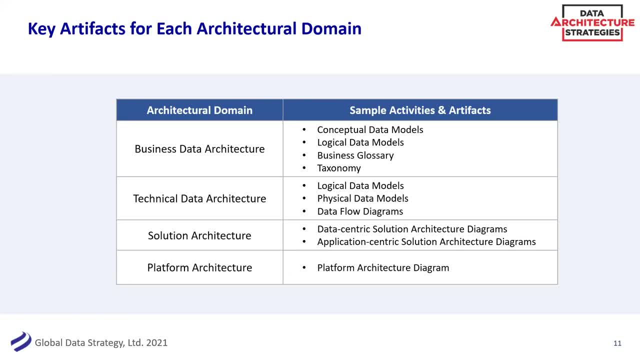 And some of the weird design decisions- maybe that might have happened in certain use cases- is sometimes when we're mixing them, we're using them for the wrong application. So within a solution architecture, you might be talking about an application like your CRM system, your customer relationship management system. 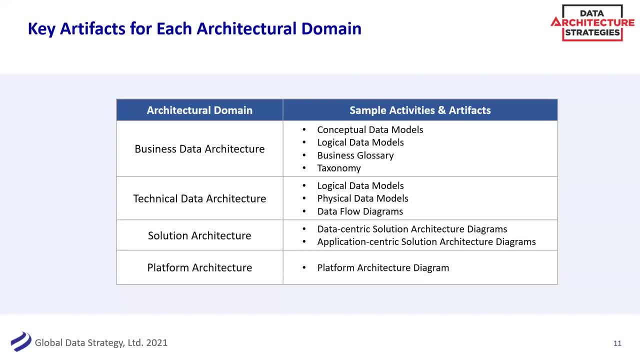 Or maybe you're designing the data solution architecture itself, the reporting and the analytics and things, and really understanding which one you're talking about. or is it a high-level solution that talks about how those solutions fit together, But really that's more of the application type level. 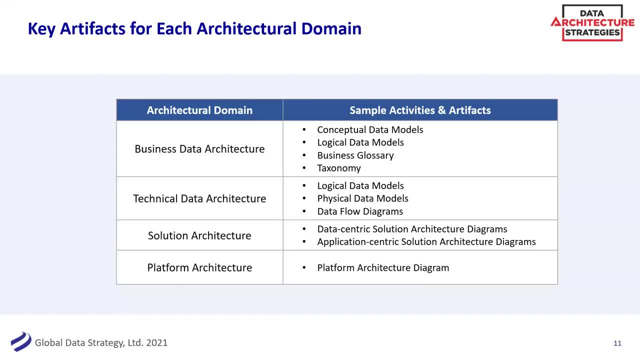 And then the platform, to me was more what Brian was showing. Do we have a multicloud architecture? Is it on-prem, Is it both? Are we migrating from one to the other, Which is super important to align with what your business is trying to do? 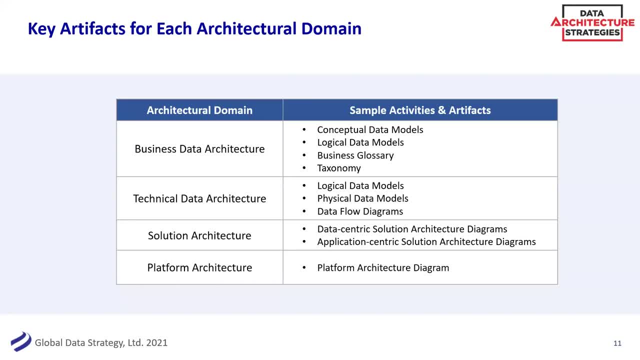 And are we trying to be fast to market and really get to that speed that Brian was talking about? Or I mean, I'm working with a couple of clients now that they're thinking things are going too fast when we're talking about something like a financial report. 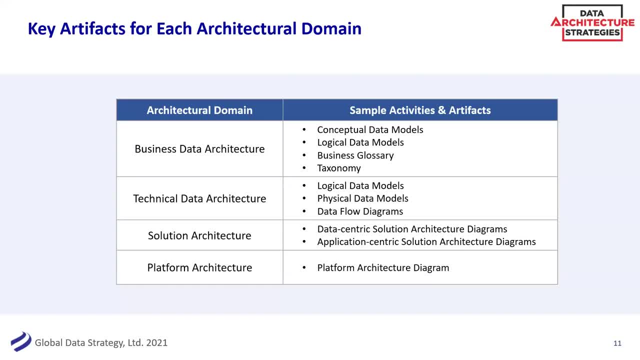 I really don't want that real time. I want someone to vet it before you send it to me, And those are two absolutely different use cases. Both are valuable, but you don't want to have the wrong architecture. You're not going to use Kafka necessarily for your financial reports, or maybe you do. 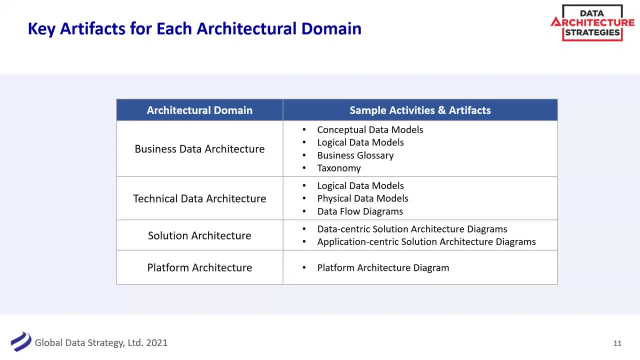 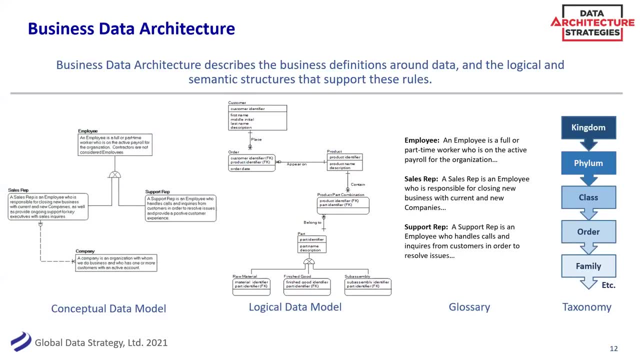 So, anyway, that's why this is awesome, That's why this is all integrated, and you really need to look at it holistically. Okay, So some examples of pictures worth a thousand words, And again, I'm sure there's some differences of opinion of how I showed these or what might be included. 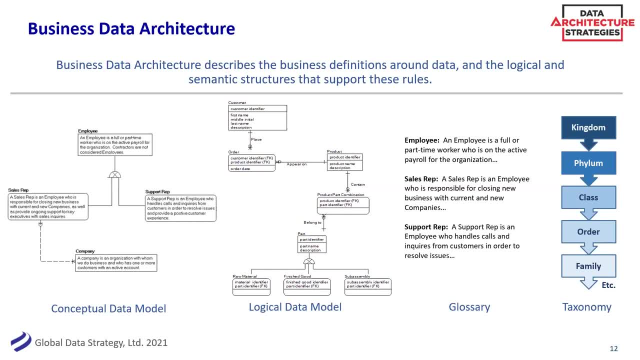 But I think as a general hand wave it's a fair, fair list. So your conceptual data model and there's different flavors of these and I kind of change my style depending on the use case. sometimes The one on the left I like and that particular tool I like because it shows the business. 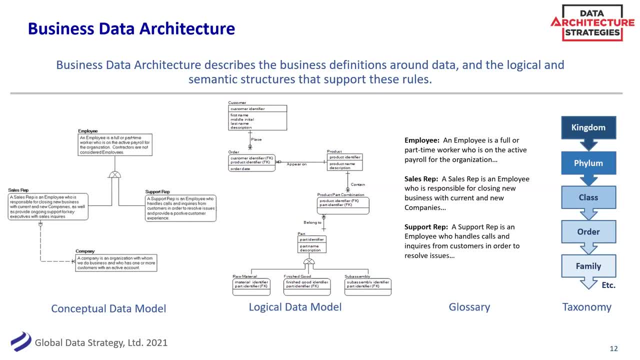 Shows the business definitions right on the model. So you know that classic what's a customer, What's an employee, What do we mean by a company? You can show it on the model and that's where you often get some feedback. 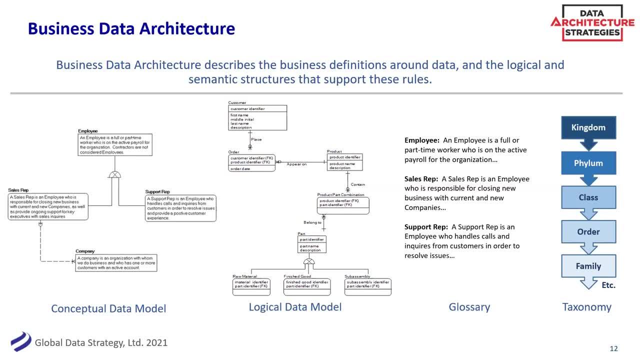 An employee is a full or part-time worker. Oh no, we don't call part-time workers employees. We're only talking about full-time. Well, there you go. You see it right on the model, and you don't have to kind of have a separate discussion around that. 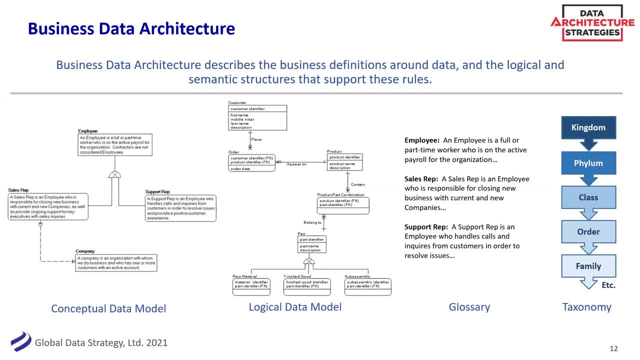 Obviously you can get busy as you get into bigger models, But for a conceptual data model they're kind of by definition should be a bit smaller. That's one example. The logical data model again is using business-centric words. Anyone can probably look at this and kind of understand what we're talking about: customers and orders and products and parts. 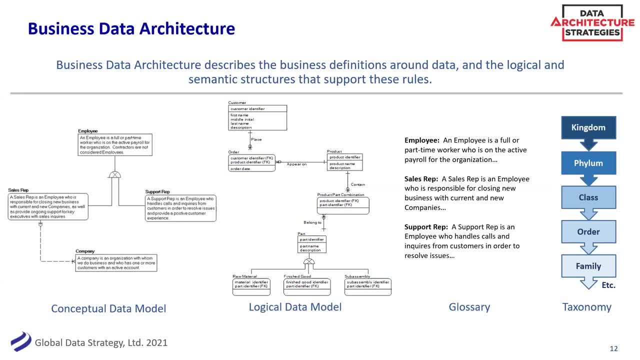 Is it a raw material or a finished good? And you start to see some of the attributes. Yes, you could put data types, You can have different flavors, But that is a good definition of. we're still very much at the business level. 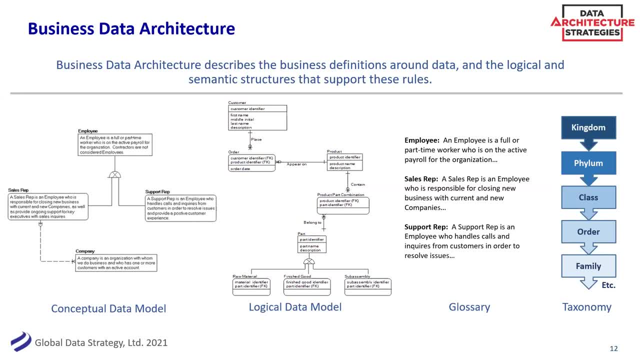 For example, I didn't know that we, as a product, would be considered a raw material- the parts I thought we were just selling full products. Right A business decision? right there Or no, we never sell raw materials. We're only going to sell finished goods. 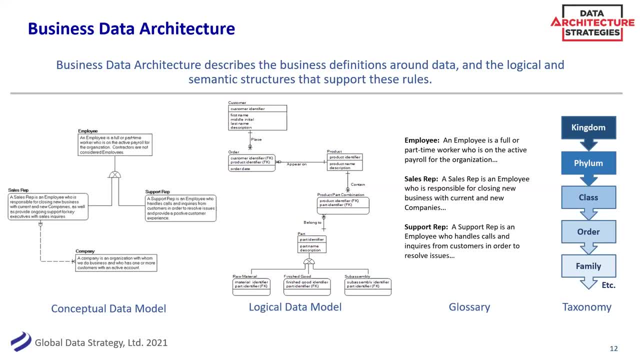 Please change the model. This database shouldn't include that, Right? So that's your logical data model. A glossary again. is that an architecture? I think so Because I listed a very simple one where basically it's look definitions on the left. 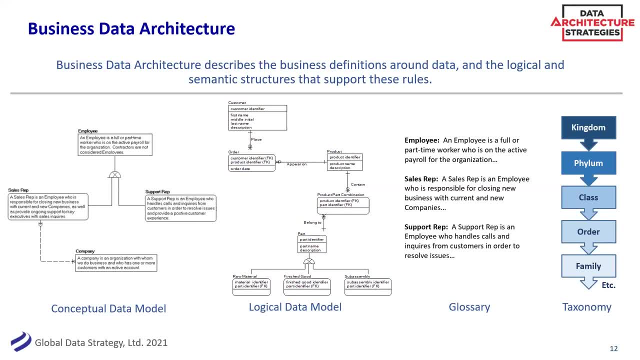 I think conceptual data models and glossaries go hand in hand. But you may have a hierarchy within your glossary Right, You may have linked terms, You may have versioning. I mean glossaries in themselves, A simple list. This is a list of terms. 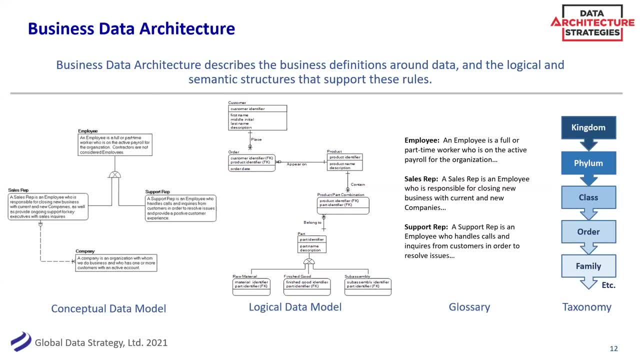 But there is a whole architecture often behind the glossary itself. So I do put that in the business architecture category. And then you know your good old taxonomy that I put, one we probably all learned in school. I think I memorized this eight years old. 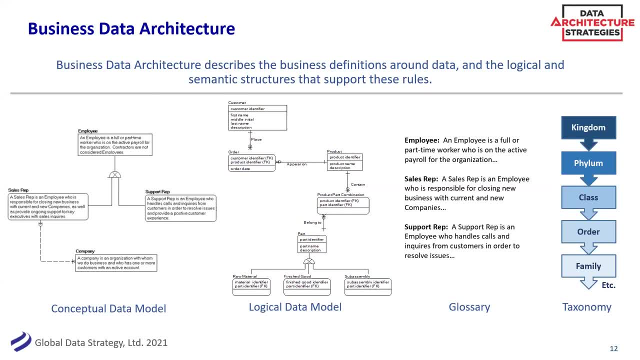 Kingdom, phylum, class order, family, genus, species. But there's taxonomies within the organization. It could be a part number, hierarchy, It could be product codes. There's a lot of taxonomies that do have their own intrinsic architecture. So again, I put those ones on the right because I think they're often sort of forgotten when we talk about data architecture, because we often think we want to model a thing with boxes and lines. 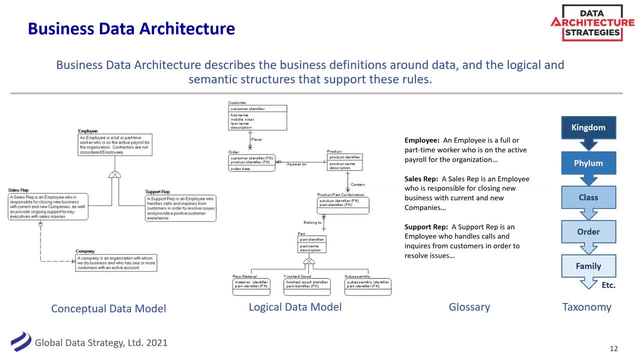 And I just don't want to forget those as well, because they should be architected, And I'm using them more and more in my engagements as well. So there's your business data architecture. This isn't a business architecture. That's a whole other webinar. 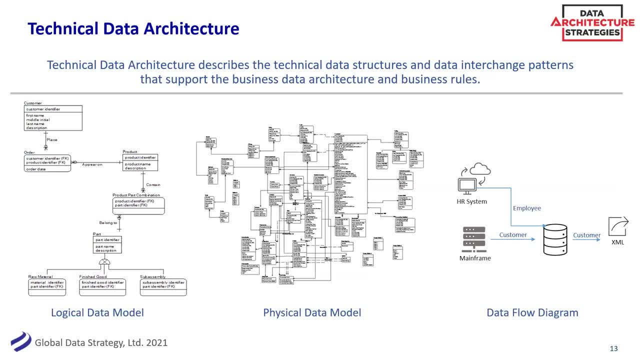 It's not related. When we get into the technical data architecture again, there's lots of diagrams we can use there some common ones Again. I put that logical data model there again because right now we're sort of assuming that sort of is starting to look like a relational database. 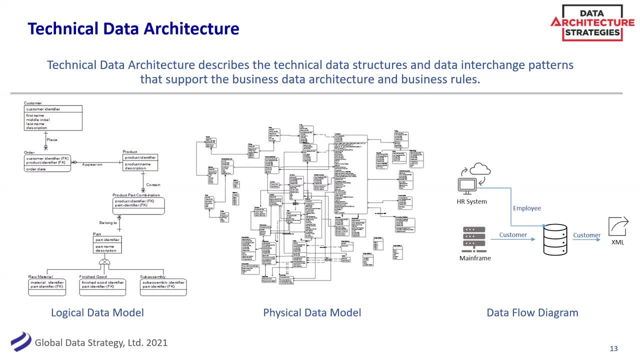 It's not a graph, It's not a key value pair. We can kind of get a sense of some attributes and maybe some. now there's some design decisions. Look at that subtype. Do we roll that up into a part? Do we roll it down into separate tables? 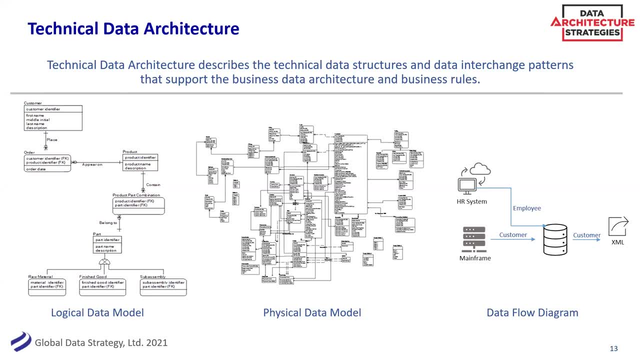 Right, So that you're really starting to build the thing on the right, which is more of your physical data model, where you're getting more into. how are we going to implement this on a database, or databases, or file systems, or however you're going to do it? 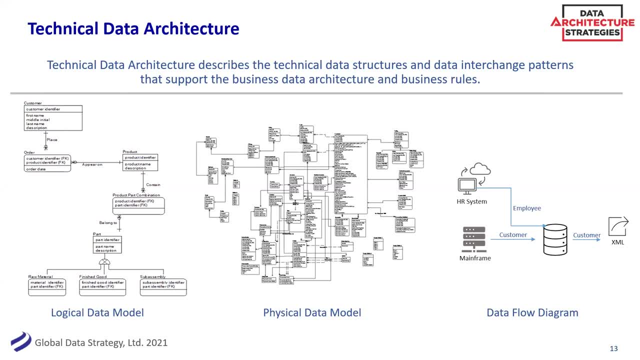 A data flow diagram. that's probably where I see the biggest difference in how they're shown. You know there are some standards. I think some of those standards are kind of old school. I tend to often use pictures to kind of show you know how things are: flowed, flowed, flowed, flowed. 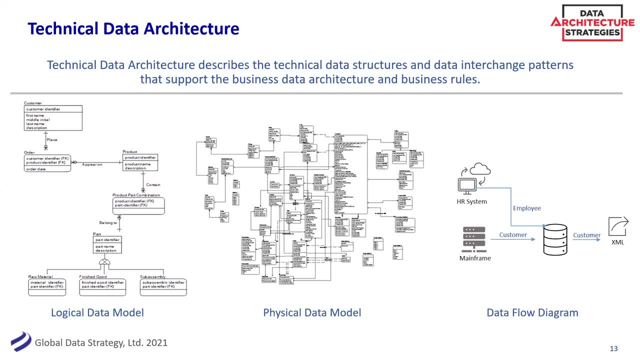 Between different systems, between databases? Are we sending things through XML or JSON or whatever? But to really get to that flow of information I often see physical data models are pretty common Dataversity and I we do a survey every year in terms of data architecture trends. 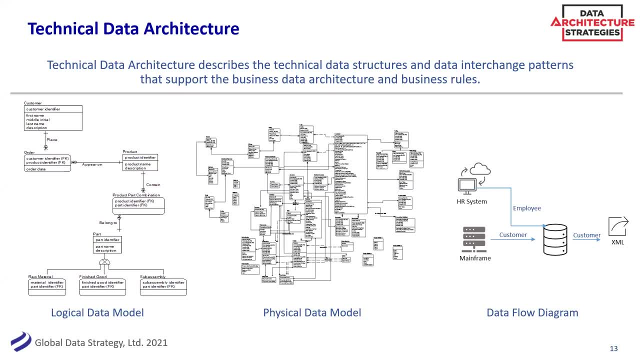 And we ask the survey of which organization is using data models. Logical and physical data models are almost everybody right. They should be the bread and butter of your organization. I think data flow diagrams should be used a bit more. I often don't see those. 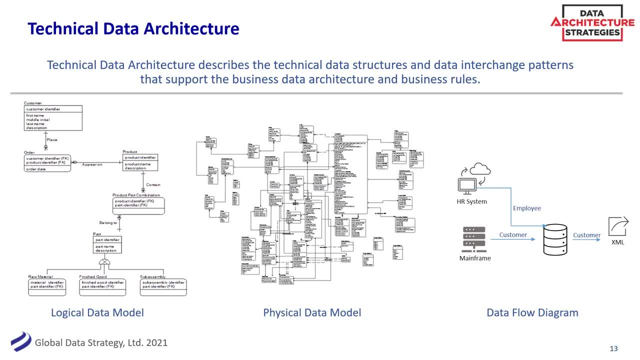 And I think often when we have a business issue or a master data issue related to data, it's often that flow of data. I think I've probably told this story 100 times because I'm still so happy about it. We did one engagement where we did kind of a data architecture agile sprint for a retail company because they had problems. 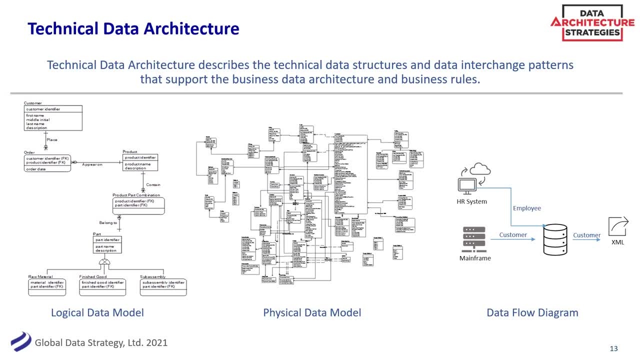 They did not want to do the big architecture, They wanted things fast. So we just did sort of mini versions of all of this architecture. We did a data flow diagram, brought it to the senior execs and the chief marketing officer said: you know, lady, I never thought I would use the word data flow diagram in my life. 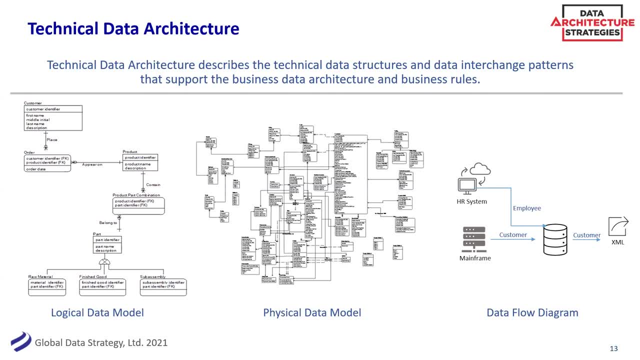 But you're the first one that explained why my marketing campaigns weren't working right, Because she had emails coming in from sales system And I think this company had three different master data management systems. if you can imagine the problems there, that inherent problem. 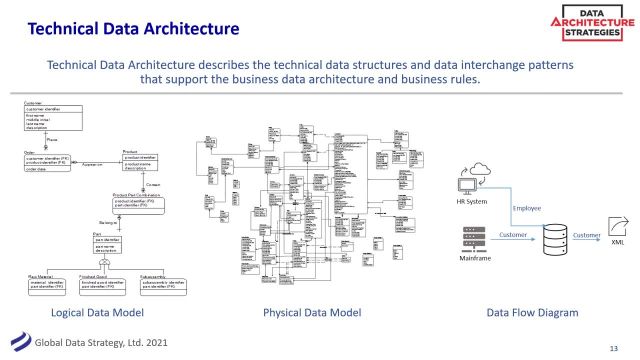 But it had never really been drawn out in a clear way. So that's why I think data flow often gets to some of those core business issues that maybe have been hidden in other diagrams. So there's your technical data architecture. I think a lot of folks are probably familiar with those or build those in their day job. 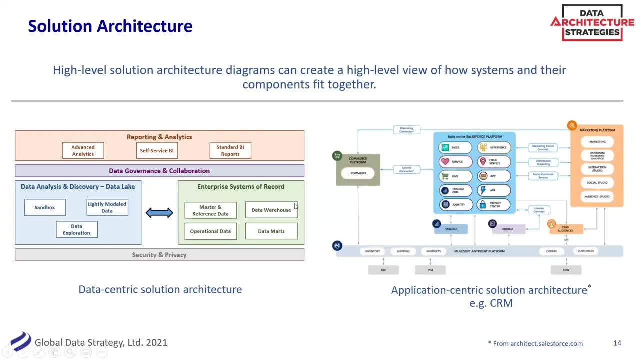 Now, solution architecture. a lot of different opinions here, But I think those are more your. how does a solution fit together? So the one on the right full disclosure stole from Salesforce. Part of the reason I picked this one. Part of the reason I picked that is because this is a CRM system. 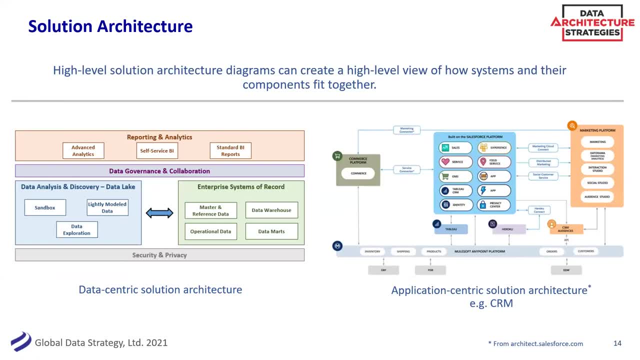 And this is showing how the various components of the CRM are fitting together. In some ways it's a data diagram. You'll see there's Tableau there. It's almost like a data flow diagram And you're seeing the different is integrating with an ERP. 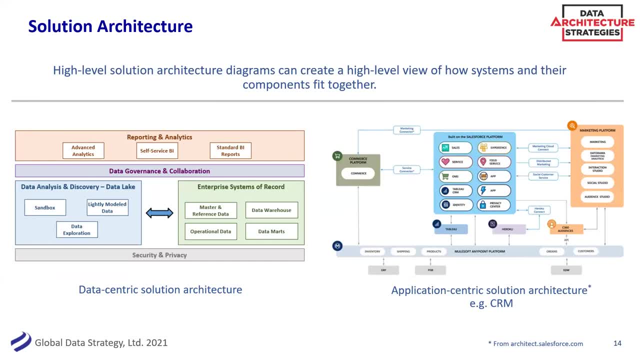 But this is about the solution And I won't do a full rant that a CRM is not master data. It is a customer relationship management system. It's a solution. It's a solution for customer relationship management. Yes, a lot of master data is in that system. 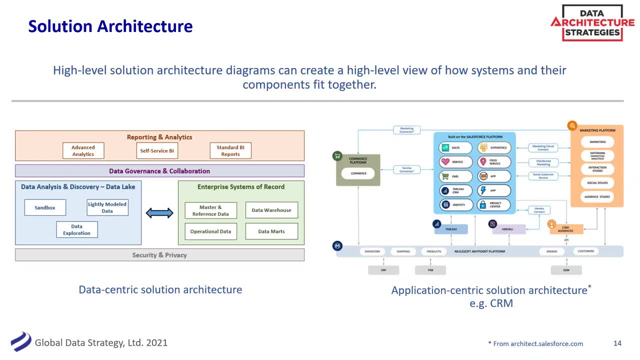 But one of the reasons I picked that is, if you're designing your CRM, you're designing that solution. that, yes, should fit into these other applications, But don't mix the two. And that's why I picked this one, because I can see it has boxes and lines. 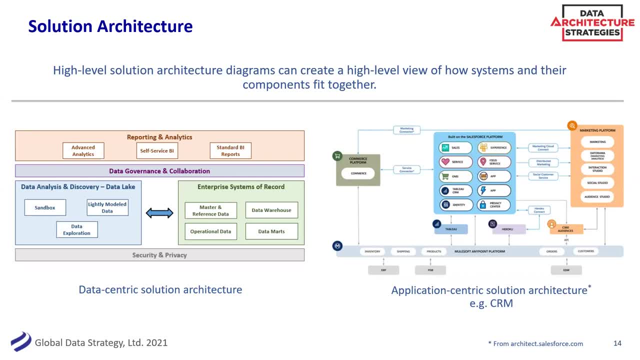 It has arrows, It has some data-related things, But this isn't a data flow diagram And this isn't a data diagram. It's a solution architecture about a CRM system. You can also have a solution architecture about your data. So this is a good example of- I'm kind of showing the reporting solution or the analytics ecosystem. you could say. 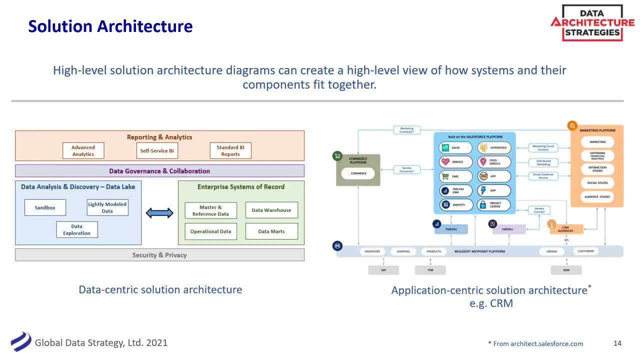 And that's where we kind of do have the lake and the analytics and the governance. I put governance in there, even though it's a solution, the best part of the solution. So again, these tend to be high level. It's more about how the various components of that solution fit together at sort of a high level. 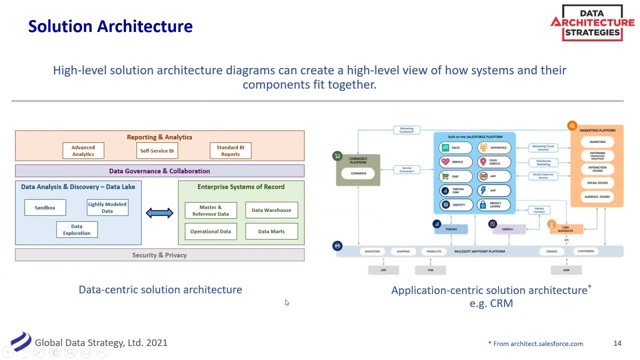 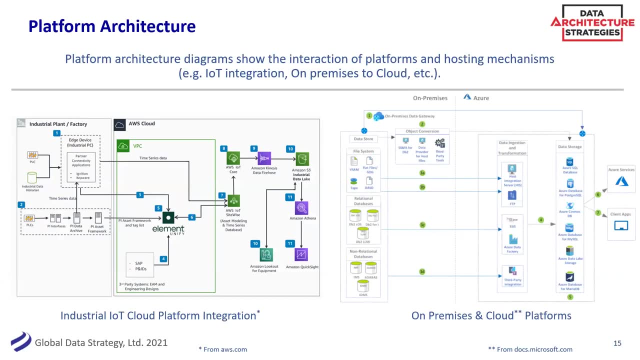 And again it can be more of an application or it could be the data. So when we get into the platform architecture, so many flavors of this. And again I stole two from popular vendors out there And actually you could nerd out for as long as you'd like on some of this. 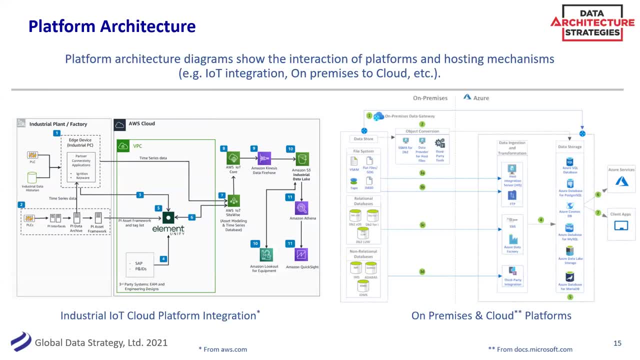 So there are so many- And Brian alluded to this at the beginning- There's so many different design patterns right now for your platform architecture. It isn't, you know, the old days of I don't know. just spin up the software. 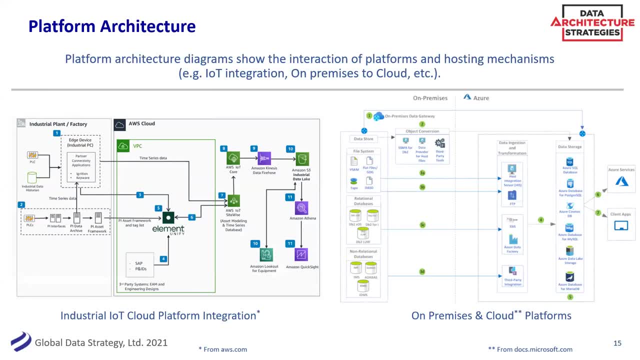 And put a database on it. You know really, firstly, aligning with that business purpose, And these two are very different. Am I doing an IoT integration for a factory, Am I doing a reporting solution Or are we doing a digital transformation? 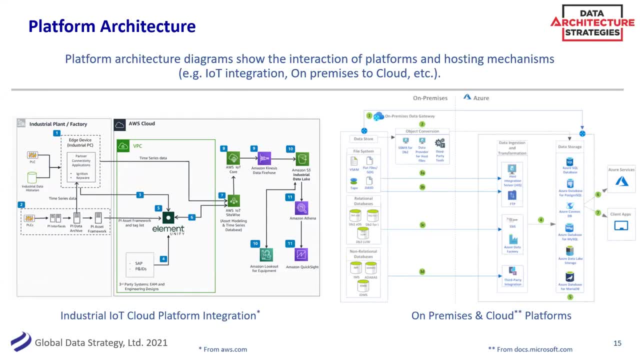 Maybe the one on the right is moving from on prem to the cloud. Are we doing a shipping system? Are we doing a? you know there's so many different patterns. Are we integrating healthcare records? So one of the reasons I stole these from the vendors is because it's fairly neutral. 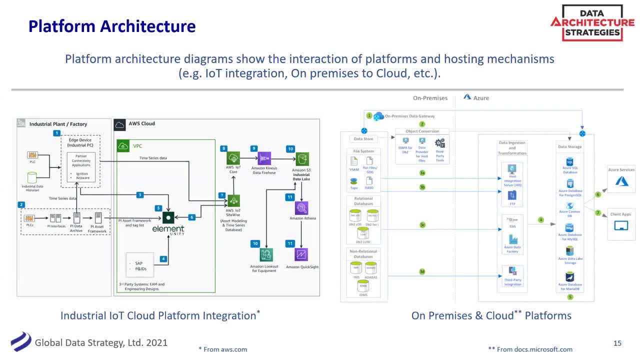 And they publish them. But if you look at some of these vendor sites, these are common cloud solutions And a lot of companies are now struggling with. do I do multicloud? Do I do a mix of? on prem and cloud? And the one thing, whether I agree with all their design decisions that are published out there, they're a good template. 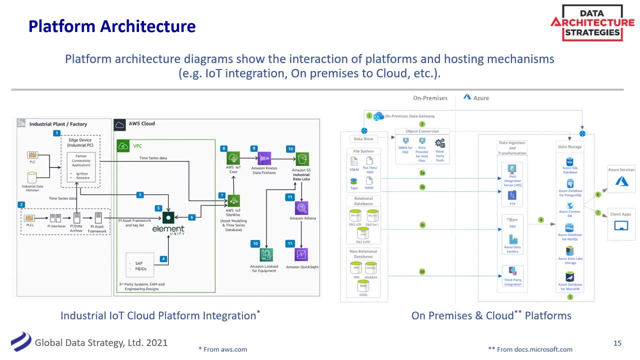 And if you sort of look, they have you know. here's an example of a cloud migration, Here's an example of a real-time data streaming for a web app, And you can kind of see these very different patterns, Because there's a lot. 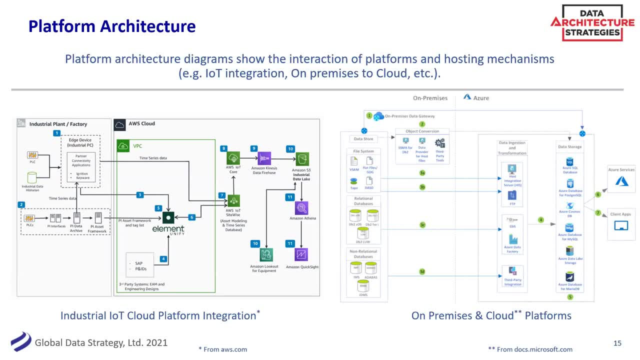 And this is again as Brian mentioned in the beginning, this can. I'm a huge fan of starting with a business and driving from that, But if this platform isn't supporting it, and you do have this cool new, sexy app and it's not fast enough and it's not performant, right. 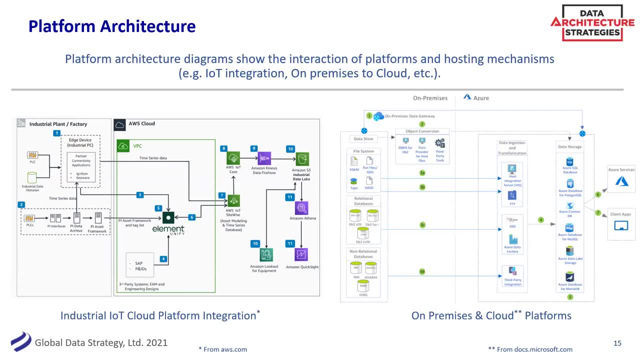 Or you're doing reporting and you don't have the right governance feeds that tie into it, it's not going to be successful. So, really, This is really the core and the foundation of everything. that seems like you know the nuts and bolts. 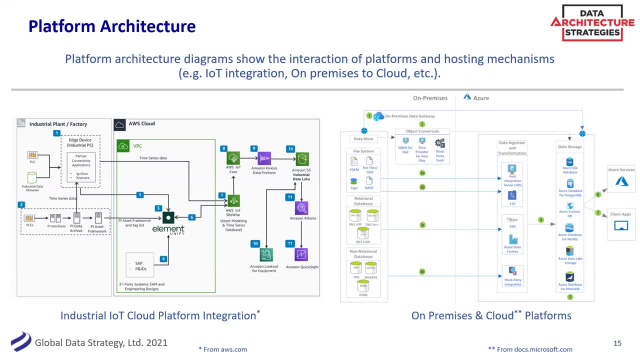 Maybe we don't need to worry about it, But if the nuts and bolts aren't secure, it's going to fall apart. So those are some different ways to kind of show them. There's a lot of different flavors of this, But these are kind of two from some of the leading vendors out there. 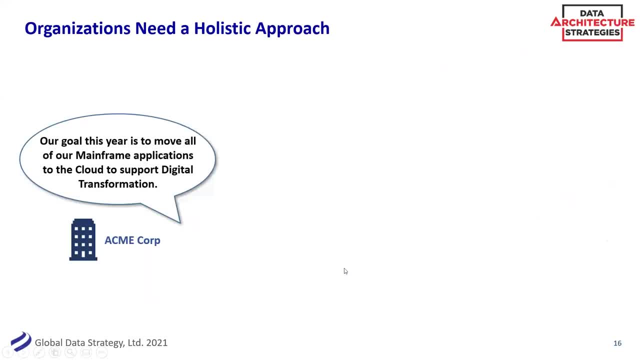 So hopefully that's interesting to you. Okay, So if you've heard me speak before, you know I like to look at that holistic approach And really look at the so what, And I think this- Obviously Hackamy Corp is sort of a fictitious example. 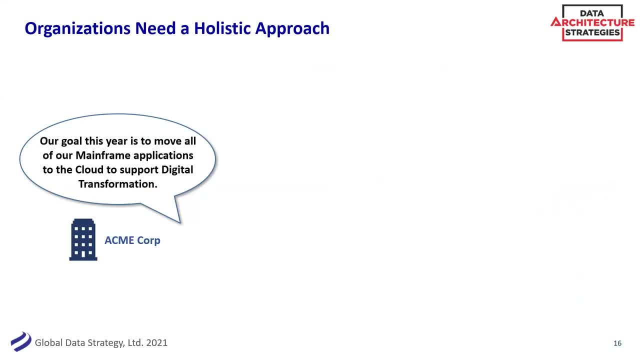 But this thought bubble could be so many organizations right now We're trying to do a digital transformation. We're trying to move all of our mainframe applications to the cloud. We really want to be faster, more digital, et cetera. 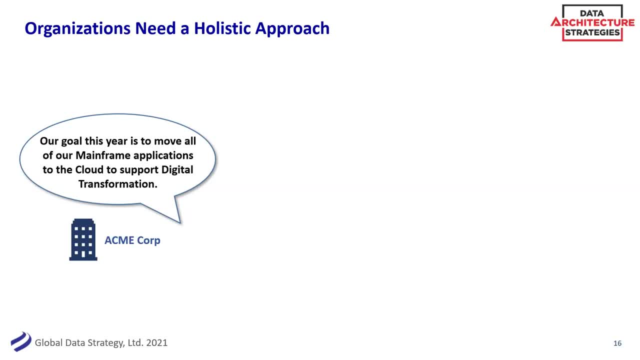 You might say: seriously, Donna, you put mainframe on there. Yep, You can pick on them, but they're still running And a lot of them still work. Are they the best solution for data integration? Do they have their issues? 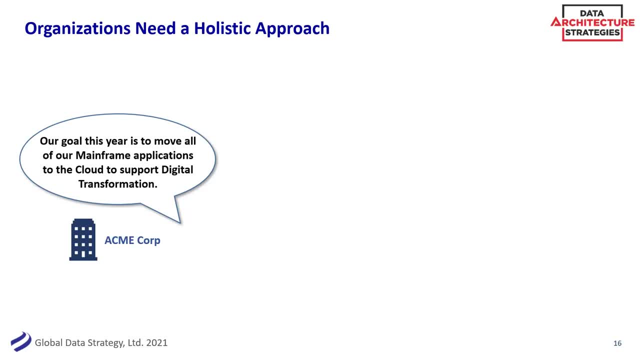 Absolutely. But yes, And often, when you are doing a digital transformation, and maybe we do want everything hosted on the cloud, you are going to have these legacy systems, whether it's a spreadsheet or a mainframe or relational on-prem database, et cetera, et cetera. 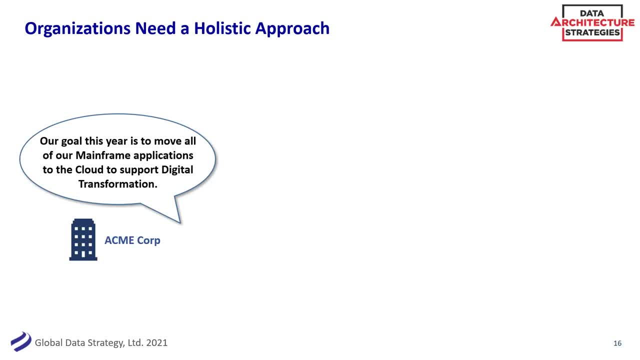 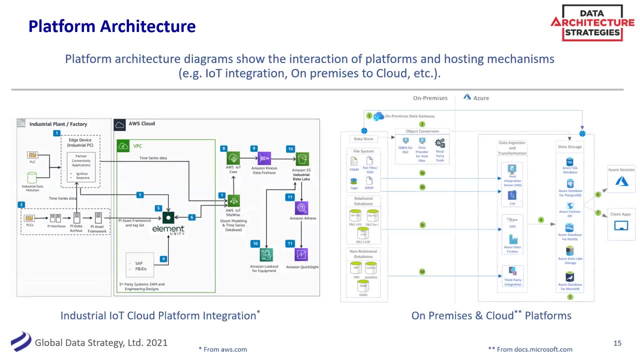 So where do we start with this? It's tempting to start with this Right We're going to. I need to move from. let's pick the one on the right. We have all these on-prem systems, from flat files to relational, to non-relational to. 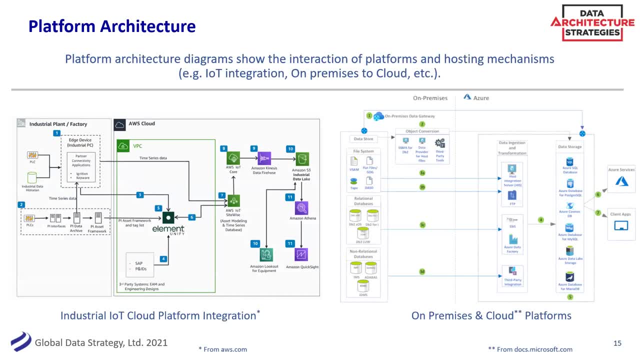 you know, there's some mainframe type things right there And now we want to move it to the faster cloud. That's absolutely important. We need to do that. I would be careful, just don't start there. It should be driven from the business question. 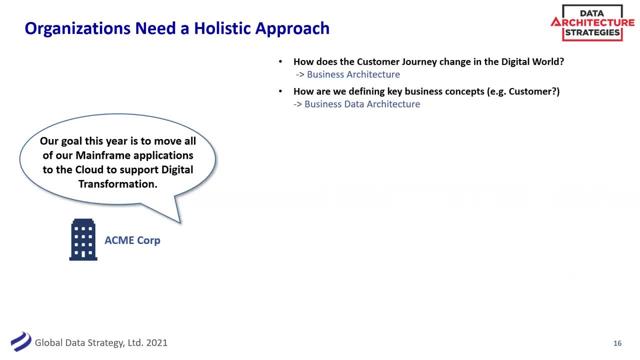 So, for example, this first one, I wish more companies did look at: How does the customer journey change now that we're in the digital world? What you don't want to do is just lift and shift all of your- you know, non-digital 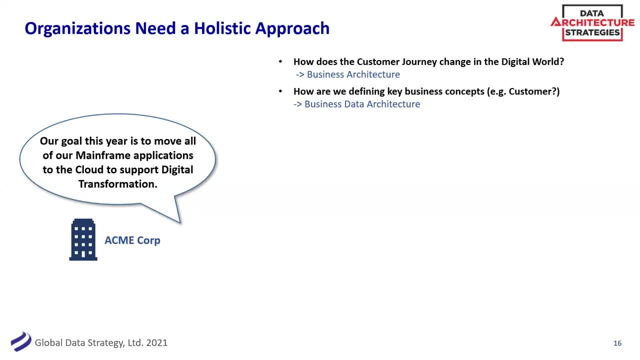 non-digital processes onto a digital world. I think we've all had some of those negative customer experiences where you know literally they're just doing kind of on. you know brick and mortar badly online And this is really a great opportunity to not just upgrade your technical architecture. 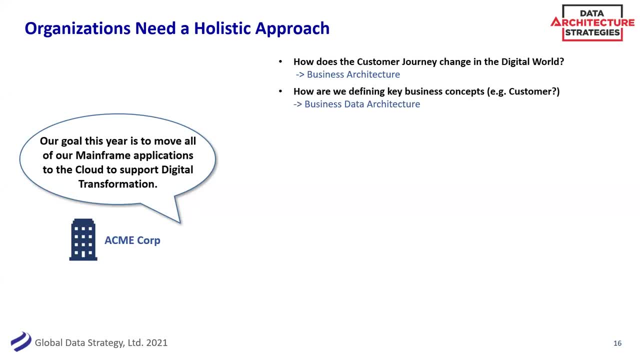 but upgrade your business. Let's step back. Let's do something like a customer journey map. How do we really change the way customers or patients, or whoever we're talking about- really interact with us as an organization? And some of the huge light bulb moments we've had with our customers are starting there. 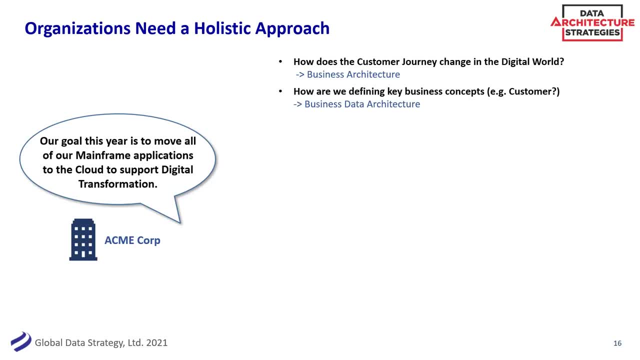 And we did a really great one with the university, where they just basically started with this. They called it the student journey map And they did a very high level data model with that, Did nothing else and just said, okay, if I'm a prospective student. 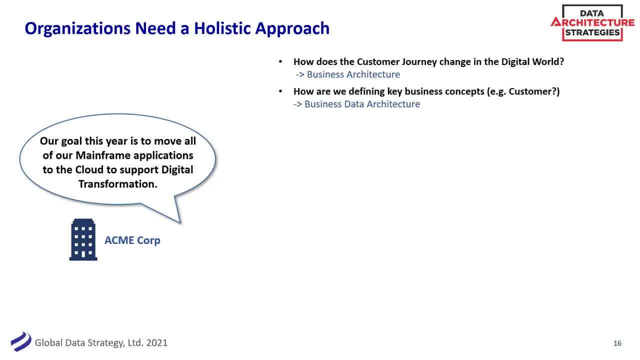 what's my best way to interact with us as a university. And they kind of started from scratch and they really had some night And they also had, you know, not to get totally off track from architecture- They had a good mix of people from the organization. 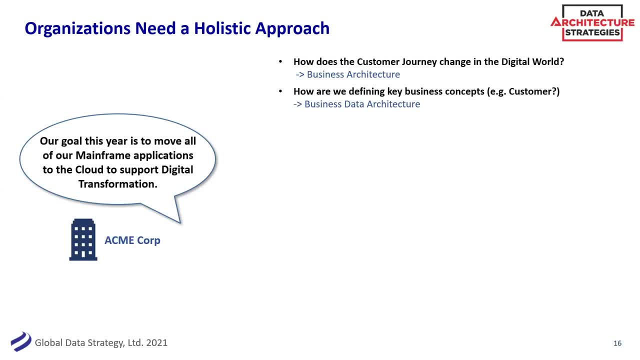 They had people from finance, They had people from enrollment, They had people who were teachers And they also had students. So it was a mix of generations, It was a mix of use cases And when you're really trying to do transformation, 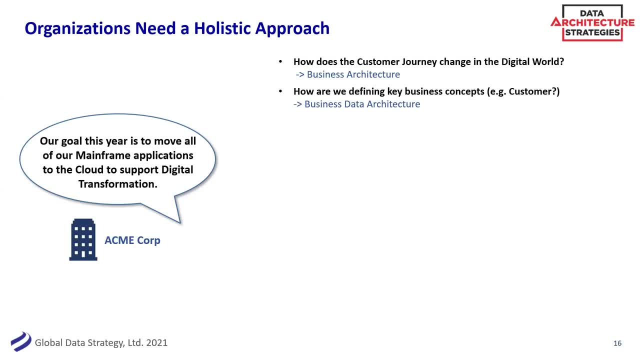 you really have to look at it from all the above. You know something is simple, And this would go to retail too, right? We're trying to change the business process, but how do we invoice? right? So you want finance in the room, or you know? 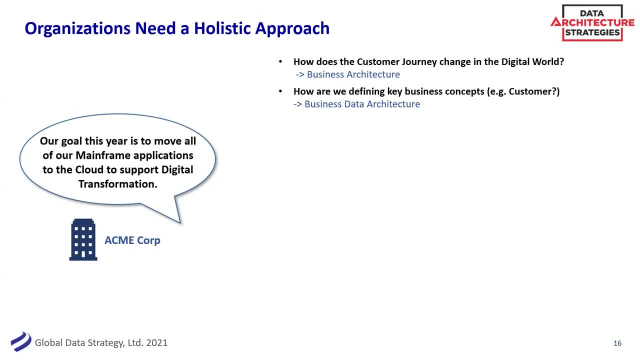 a younger generation is going to have a different perspective than maybe the older generation. So don't scrimp on that first phase and just terms of how we design the business that you're missing an opportunity if you only are thinking of the tech right. 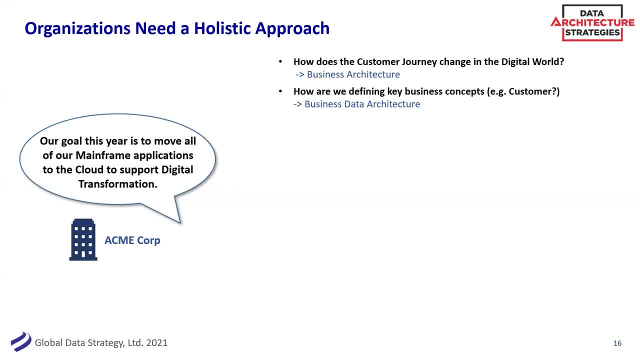 So then, as part of that, how are we defining things like customer? And this is where, yes, your friends and family, or maybe your colleagues, start to think you're crazy. Really, we need to do a whole cloud migration and you're going to sit us down and 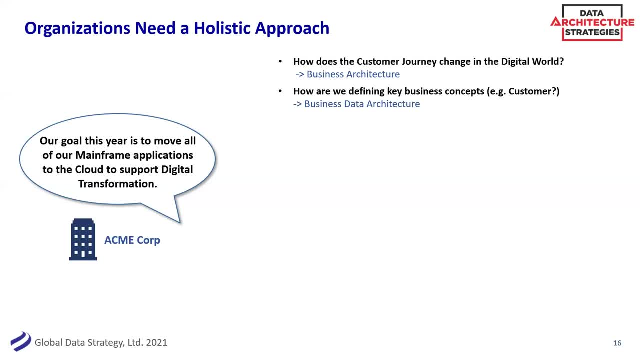 say: you know a very academic, what do I mean by a customer? But man, again I've had some of those light bulb moments. What do we mean by a customer? One of our customers has a. they were, they were very. 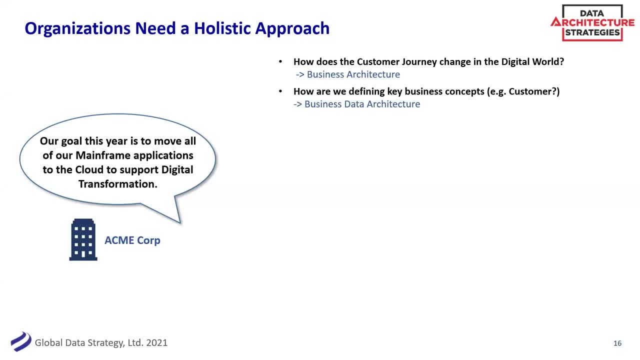 they were sort of focused on baby type products, And so of course, they were focused initially on on moms and pregnant moms, because they seem to buy the most. when they really looked at their customers, There was an equal amount of dads. Good to see how they were grandparents. 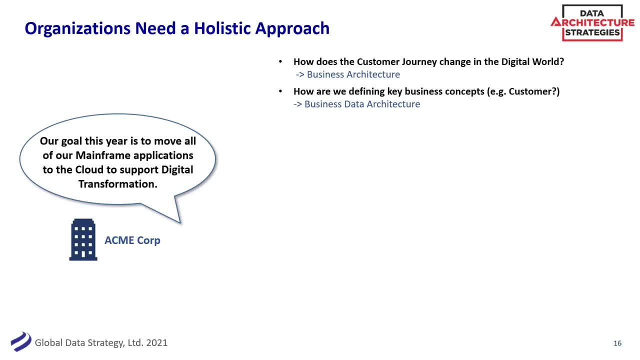 They were friends or family, So who they thought their customer wasn't. And then they were like: well, I'm going to give you a little bit of information. So they're like: well, I'm going to give you a little bit of information about the patient. 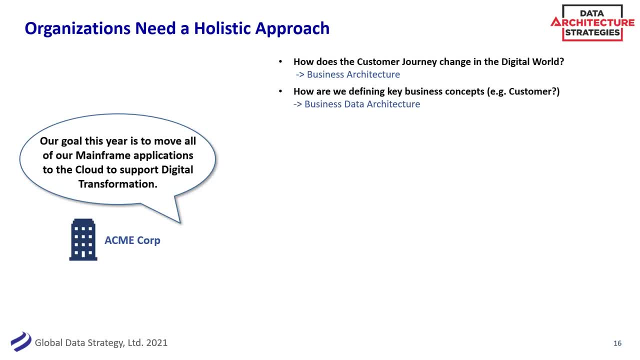 And then they're like: well, I'm going to give you a little bit of information about the customer Right. When we did the group with the university, It was not your typical 18 year old. It was returning veterans, It was parents. 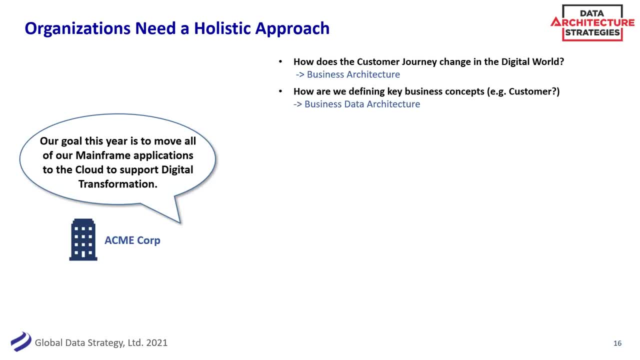 With babies on their laps. There was retired people. Who's a patient right? A lot of my kind of more Either nonprofit or medical customers are realizing the patient Isn't just the patient, That's the family right. So how would we maybe? 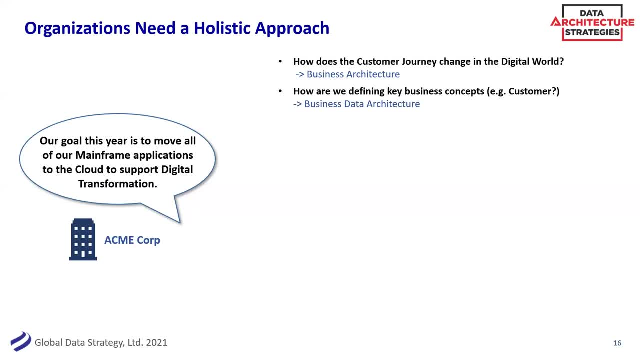 Give updates to the family and not just the patient. And so you know, I think that's a good question, I think that's a good question. I think that's a good question. I do do spend a lot and have those fairly academic, because they're 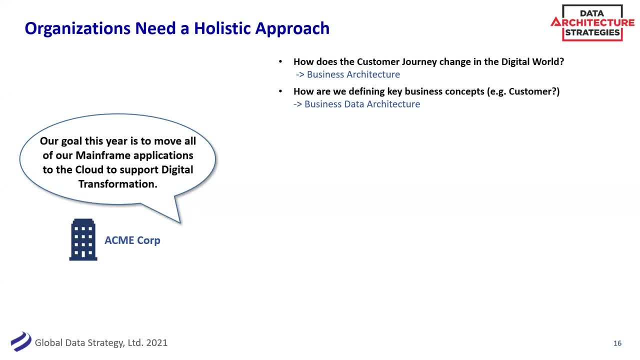 not. And the other thing- you've probably heard me in these, in these webinars- some of these architecture diagrams can seem overwhelming. You could say: that's great, Donna. You and your webinar can say: do all of this, I have a deadline and it needs to be done next month. 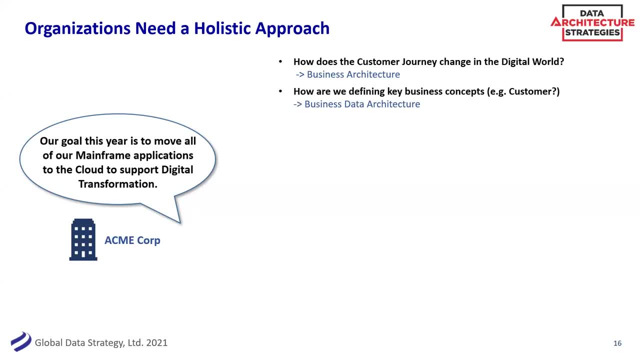 So that'd be nice, but you don't live my world. I don't live your world. But I would say, if you don't have the time, just do it in a in a whiteboard In an hour. Just sketch it out in the back of an envelope. 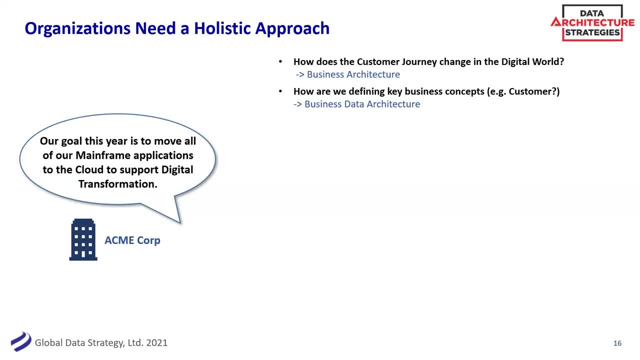 I've had some really and especially actually. And the other question is: how do we do this now? And things are opening up in different areas of the world, But most of what I'm doing is virtual. I've used a lot of 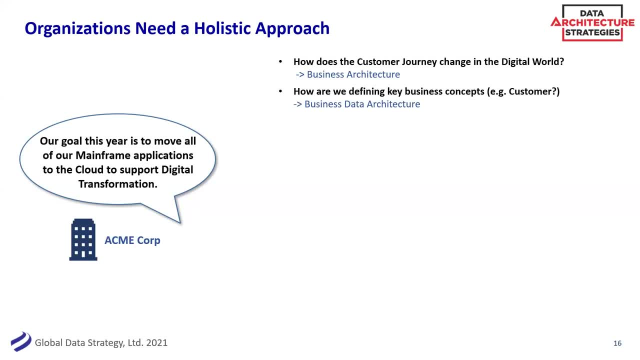 You know white boarding sessions, Miro boards, You know virtual sticky notes and we have said some huge aha moments by getting a lot of people together Just mapping out things like a customer journey and a high level conceptual data model In an hour. 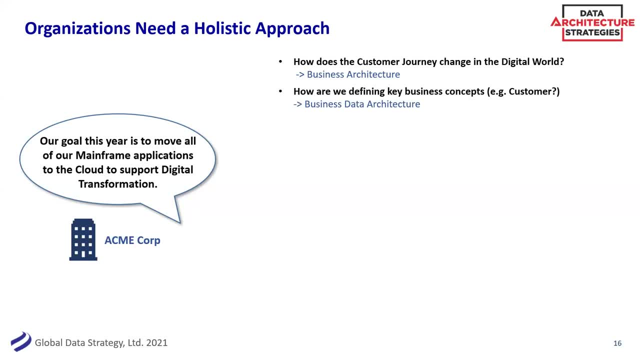 And I think in a way I'm getting slightly off track, but I don't, I think so It's actually. I've had, you know, I've been doing workshops for decades now with kind of white boarding sessions and sticky note sessions. Those are really valuable, valuable. 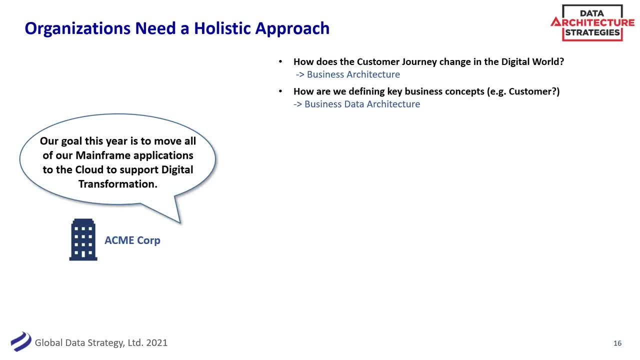 And I will get back to those when things open up. but there's something about this online almost gamification Of data modeling and architecture of. we had one really transformational moment of folks that we really were having issues Getting to And we did a data modeling session where they could be able to. 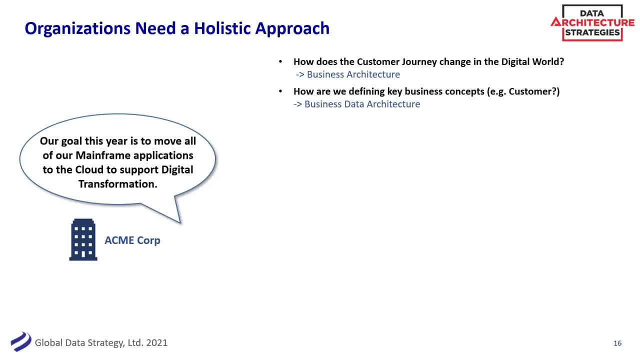 everyone could drop their own boxes and do their lines. Everybody participated And we really came to an aha moment at the end. I just think, cause it was kind of fun to drop the boxes, I'd like to think we're- we're more adult than that. 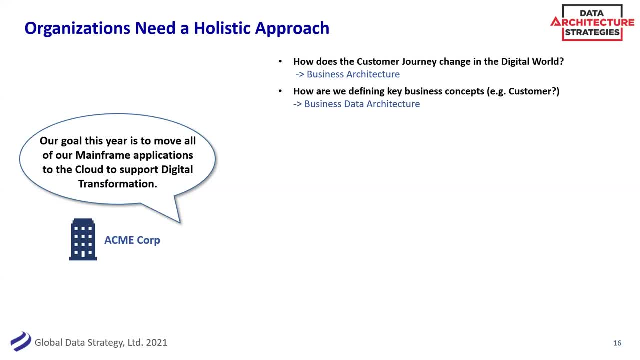 but I think some of the- it was a little more anonymous, perhaps two people, She could just drop their sticky note. We kind of did it in kind of 10 minute sprints. Okay, We're going to talk about customer, where all the boxes you would put 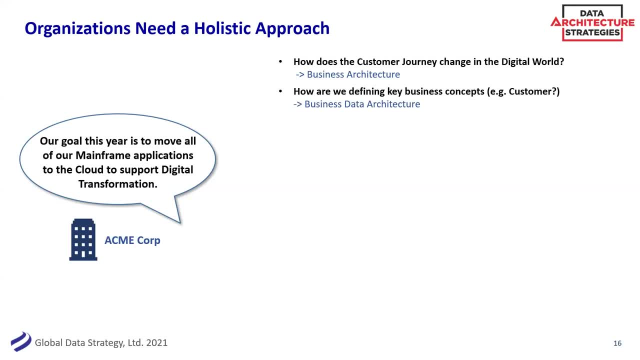 around customer in our group for a bit And some of the You know data architects in the call are going to say, great, you've got 90% of it In the hour, And then that last 10% is going to take you another three months. 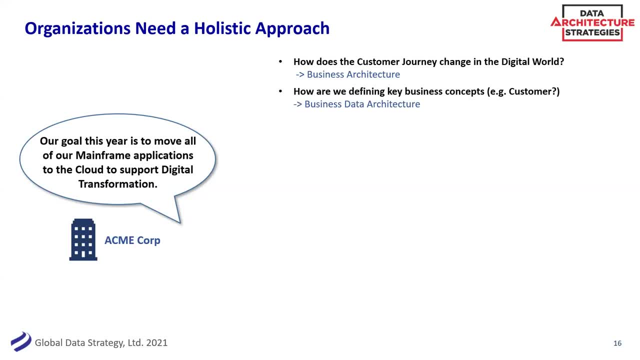 Maybe, Maybe those are your master data domains but you can go very far with especially. I'm now become a really big fan of some of these Digital technologies. You can do voting. You know on terms when you get those gnarly issues and things. 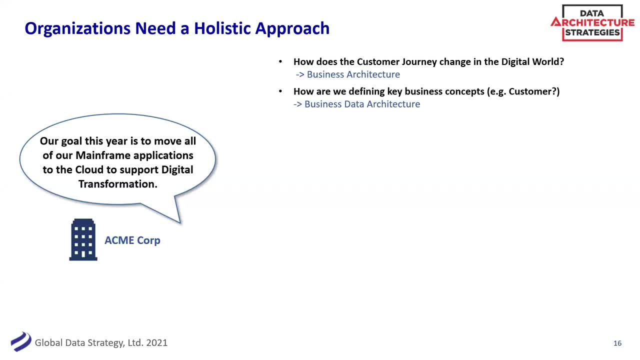 and I'll probably keep some of them even when we're in person. So Little Tent there, And then we when we get more into the technical data architecture. So these are only a few of the many questions. What data is being migrated? 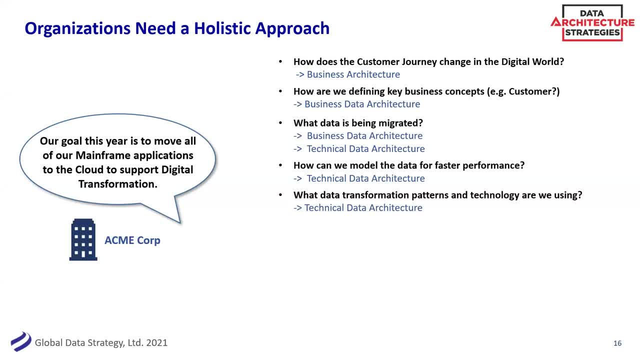 This is another one where I think there's an overlap between business and technical Again. so many of us, and myself included, Jump probably right to the tech. So okay, We're migrating to the cloud. What, what, what databases do we need to move? What technology is it? 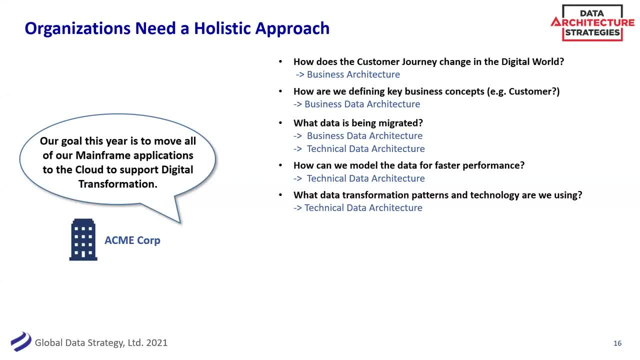 You know ELT or ETL or how do we? Absolutely important, But think about the. what do we need? Think about the. what do we need to migrate everything? What data? What is there security around it? What's the best business value? 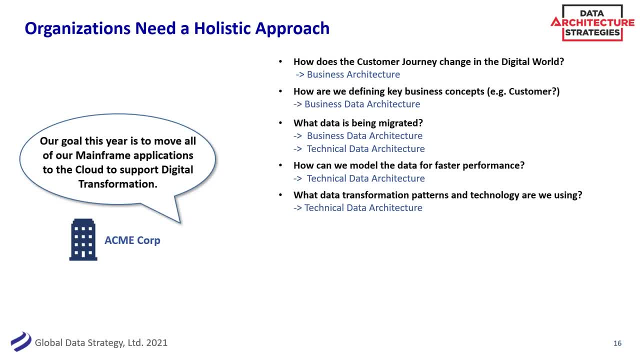 And can we pick just the high value data first? Maybe we don't move everything onto the cloud. Maybe some of the data we've been managing for years doesn't need to be managed right. So you're missing again. you're missing a big opportunity if you don't start with the why. 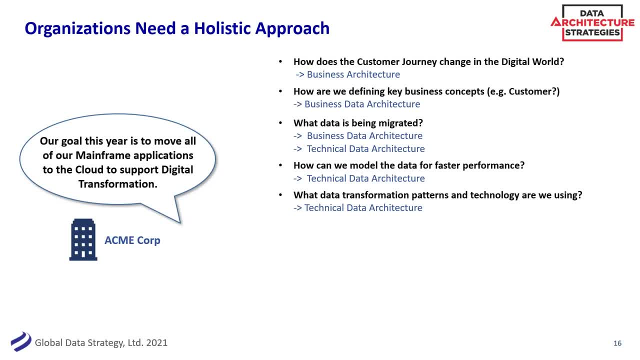 And I have seen that makes me cringe A few companies that in the rust Of, we don't have a lot of time, We just have to move digital and absolutely just Here We're going to have to do this, We're going to have to do this and do this. 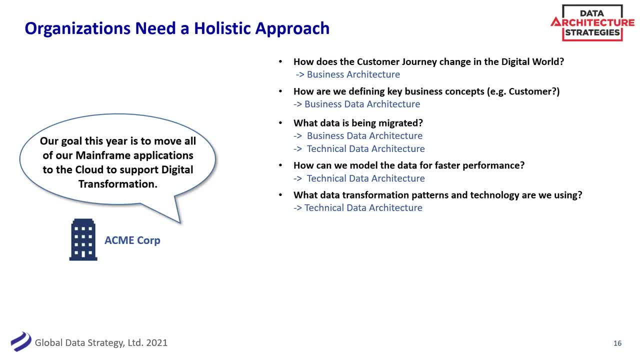 And- and we've been in the Excitement in my voice- I've literally just done a lift and shift- I can do not- from something like a mainframe To the cloud and literally kept all the data structures, all the same things. spent millions of dollars to do that. 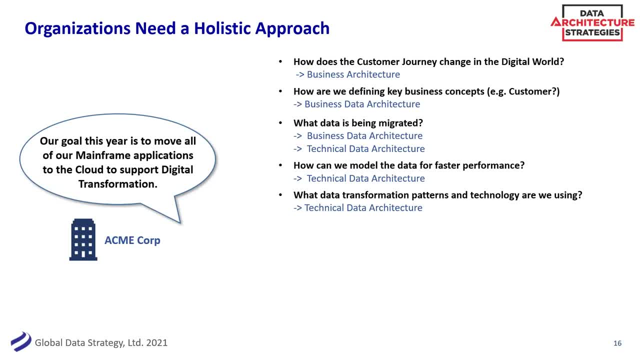 They got there faster, But what did you get in the end? You've got a mainframe on the cloud That really you're again. you're missing that opportunity to truly transform your business And really think: can we be more real time? 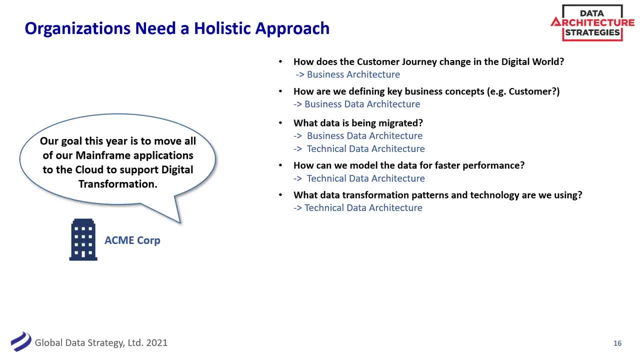 Can we be a? So don't do that. You may do that if that's the right business decision, but think it through before you just rush to have everything- quote- digital. What does that mean? We talked about this in the beginning. 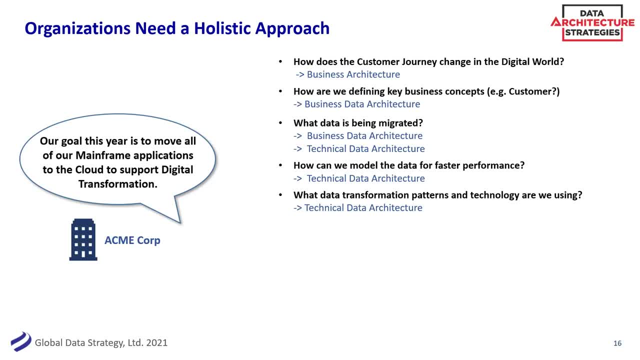 How do we model the data for faster performance Is moving to the cloud enough, Do we? just, you know? do we model it in a different way? Do we? is it key value pair for a web application, or do we want to do a relational database? 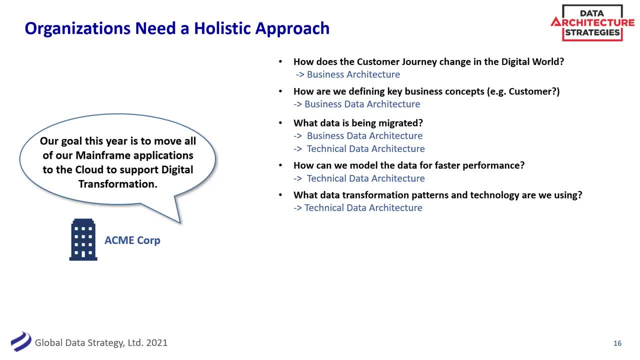 for a data warehouse, et cetera, et cetera. So a lot of new technology out there to make it faster. How do we have different data transformation patterns technology, I mean? all of those are very important and should be modeled out ahead of time. 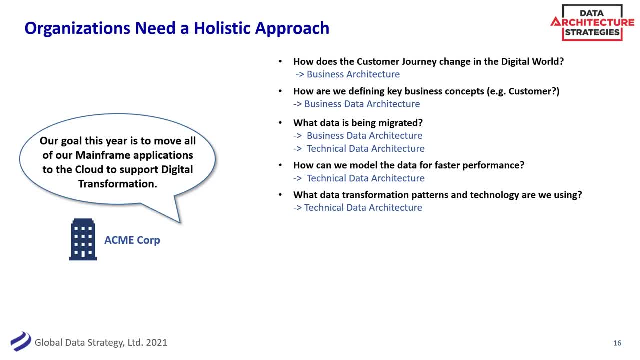 That should be a healthy discussion between your architecture team. I've had a few, I think, my team's on the call and I'm probably nodding their head that I can be very vocal in these meetings, but that's the time to do it before you build. 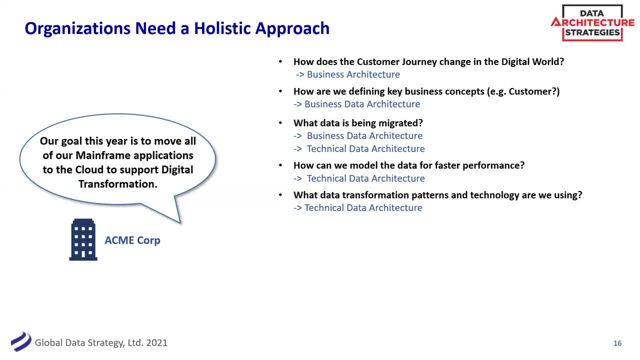 because it's hard to do it after you've built it. So, just like anything, think and then do. It's always a good mantra. So, as we get more into the solution architecture, again, there are architectures just for the solution, So I don't want to pick on CRM. 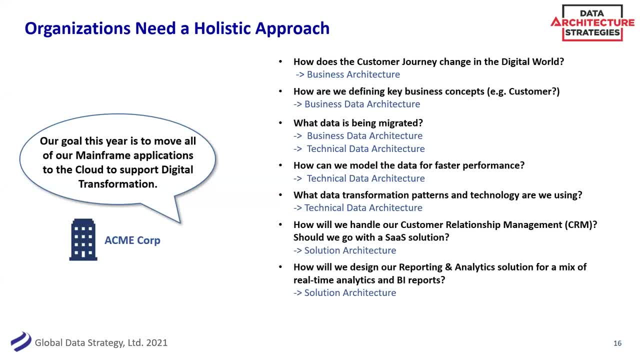 I mentioned it before in maybe a disparaging way: CRMs are awesome, So how do we manage that? Should we go with a SaaS solution? How might that integrate with our analytics? How might you know web analytics tie with our on-prem analytics? 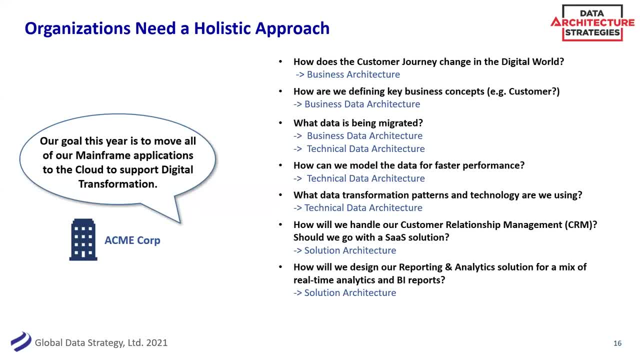 But again, you, you're doing that architecture with a solution lens and maybe I'm designing my solution for analytics and reporting, And then I'm going to do that, answer that same question with more of the data lens for this, And then again huge decision in terms of price. 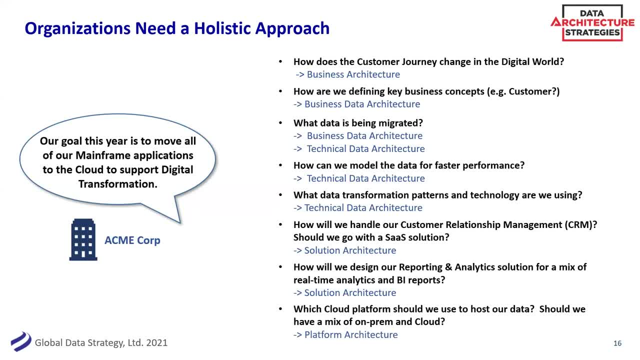 in terms of performance, in terms of vendor lock-in and et cetera, et cetera. But you know which, maybe? which cloud platform should we use? Should we have a mix of on-prem and cloud? Should we go with a multi-cloud solution? 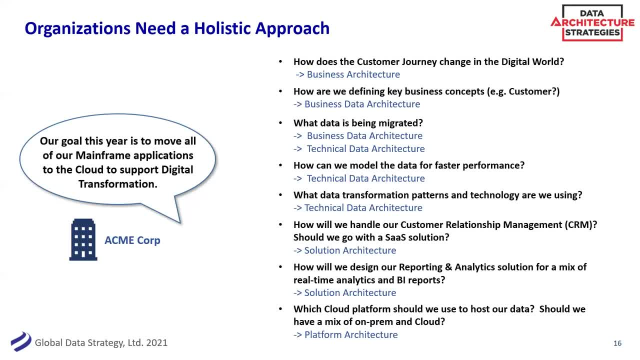 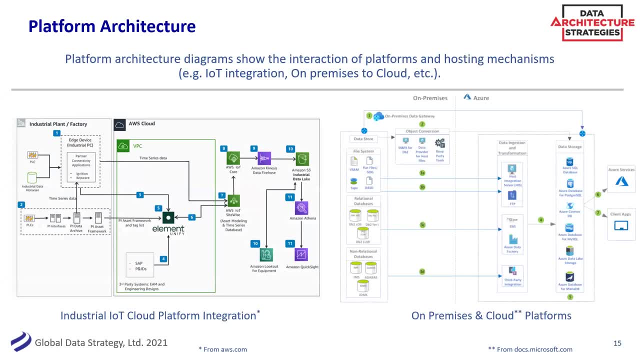 Et cetera, et cetera, et cetera, And that's some of those you know diagrams we saw in the previous. A big decision, as I mentioned, there's a lot of patterns out there, a lot of things to think about as you go through. 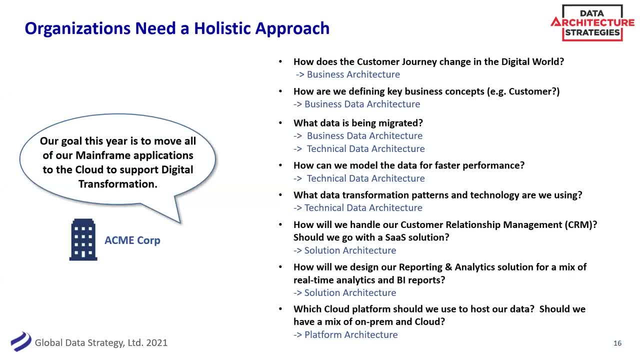 So don't skip any of these steps right. Don't only think about the customer journey and then forget you know and go and put it on a mainframe if that's not the right decision. And again, don't jump right to the cloud. 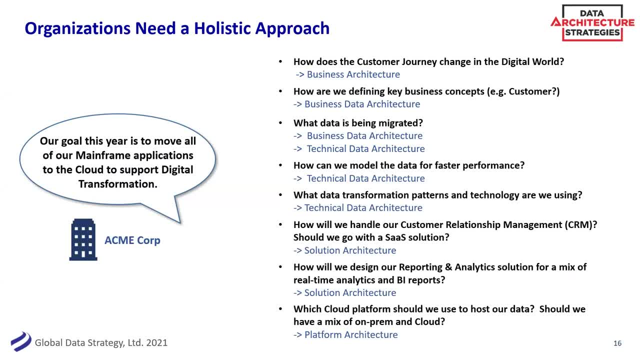 and think of all the other steps. Don't just move the database to the cloud and not look at how that database is modeled. There's so many different ways and different technologies that can support. Not everything is a relational database anymore. So again, there's a lot of different patterns. 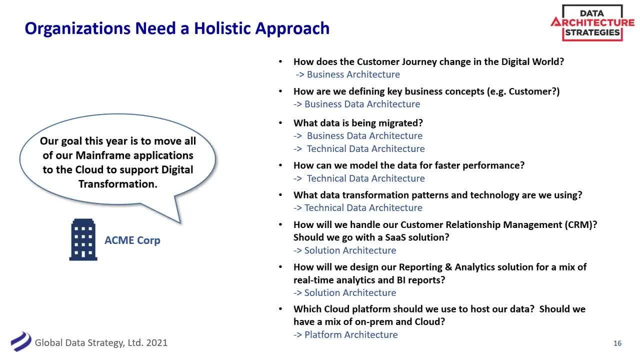 And think of it this way: There's pros, none of these design. well, there's some crazy design patterns, But it's not that these, any of these design patterns, aren't intrinsically good or bad, it's. does it meet the use case? 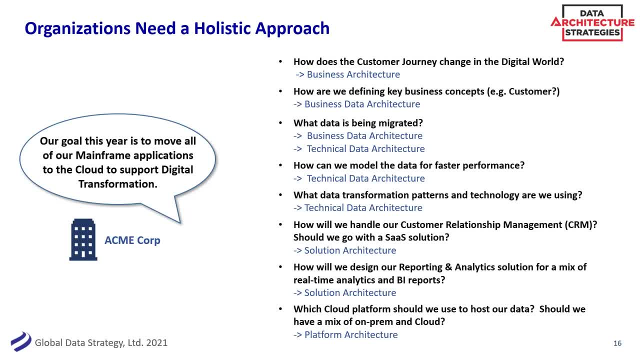 And that's why I like to think of these as design patterns at each level. At each level, it could be different Even how you define a customer. there's different patterns, There's different patterns for that, There's party models, et cetera, et cetera. 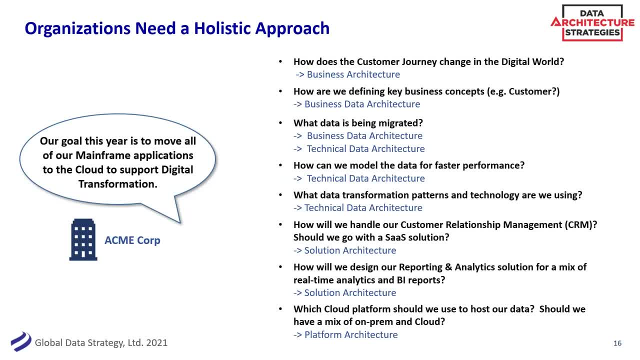 No one is right or wrong. It really just has to match what you're trying to do with the organization, which should be obvious, but it can't be said enough because I just see it skipped too many times. Okay, up for air. 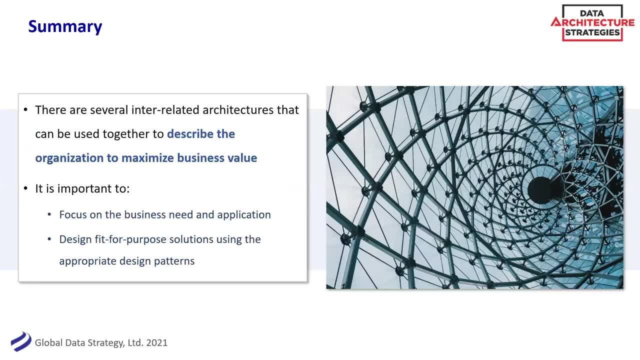 So, in summary, there are several architectures that are used together And hopefully I cleared things up and didn't make it more confusing in terms of when we talk about an architecture, what do we mean- And you might disagree with me, and I'm absolutely okay with that. 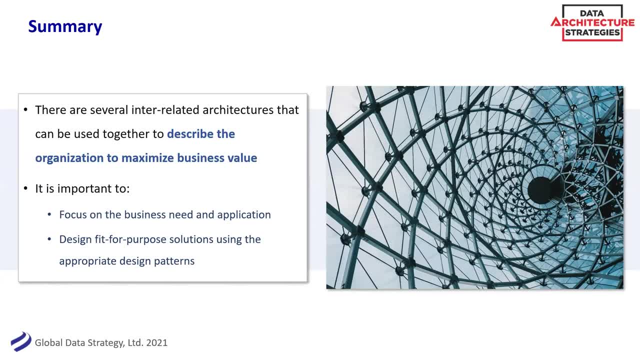 as long as we just set our terminology in the beginning. If we're going to have a meeting and we're talking about an architecture, this is the one I'm talking about and this is how I show it: good, We're good to go and now we can have a discussion. 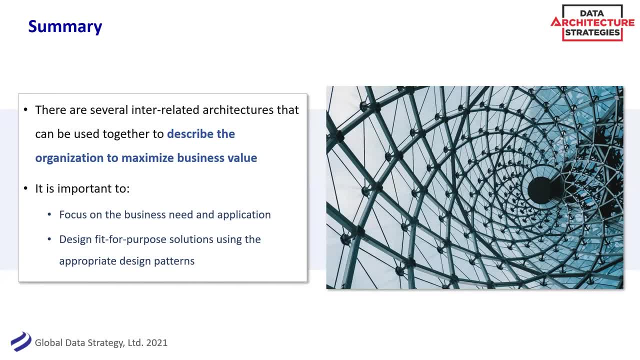 about how we can maximize business value, So don't get in that architecture. you know, I show a data flow diagram in a different way. good, Does it still get to where we want to get to? Yes, because there's a lot of different flavors out there. 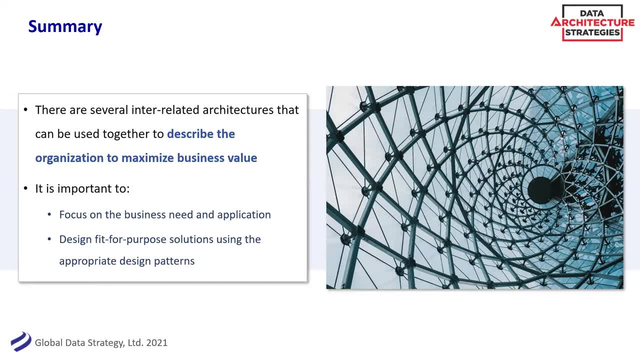 because really we're trying to focus on that business need and then design a fit for purpose. We're trying to find a solution with the right design pattern that makes sense to you, and there's a bunch of them out there, and that's what makes our job so fun and hard. 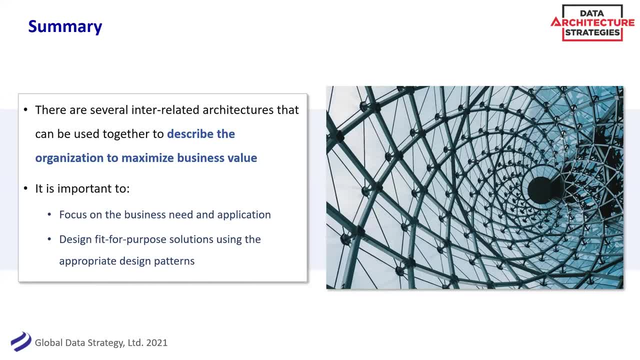 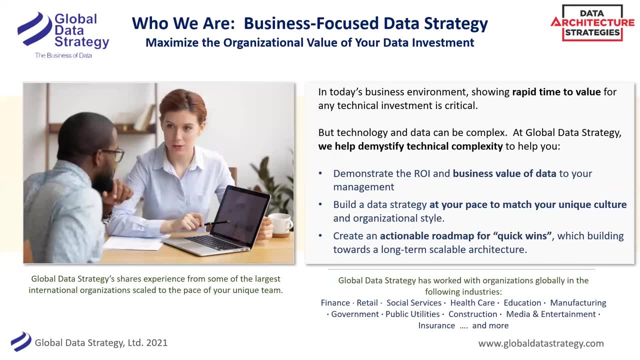 because these are big decisions and, again, that's why I like to design them before you build them, because there's a lot of thought process. So we will open it up for questions in a moment. Quick sales pitch: we do this for a living. 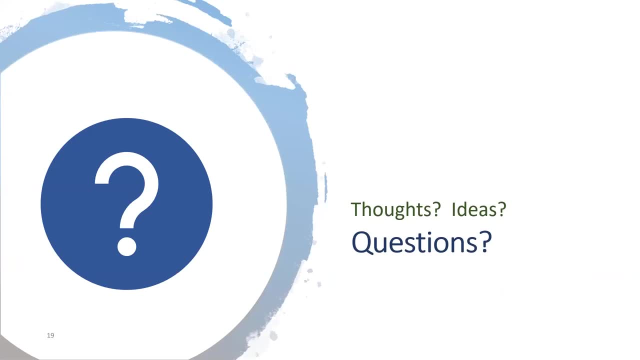 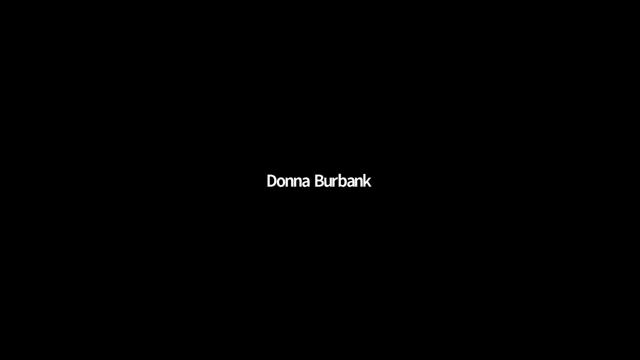 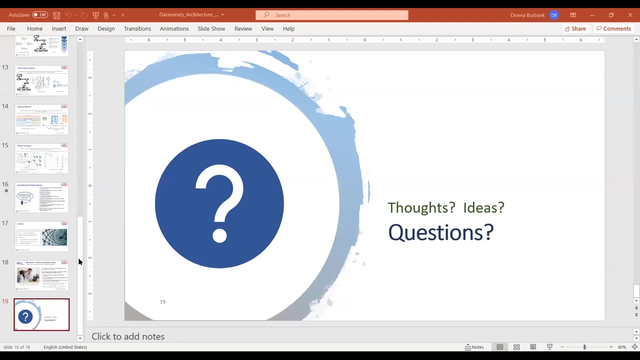 If you need help, you know where to go. And then, as I will, just one more quick oops. I think I stopped sharing my screen, but the idea is we will open it up for questions. We also have the series, and next month will be. 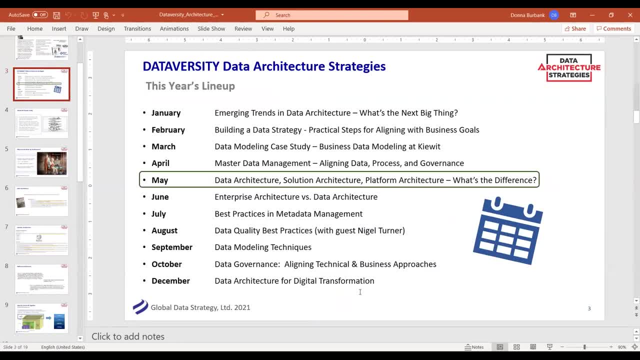 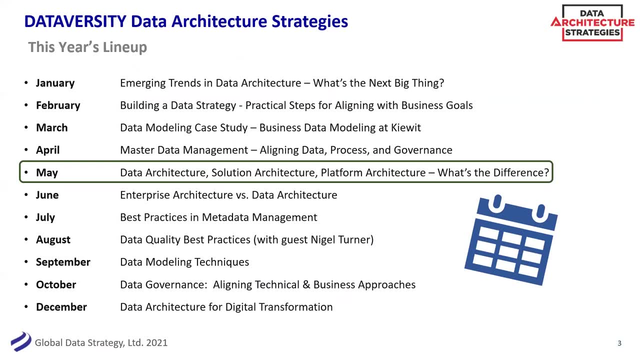 on enterprise architecture. So if you can join us for that, please do So. I'm going to open it up to Sharon for Q&A. Donna, thank you so much for another fantastic presentation. Lots of great questions coming in. Just answer the most commonly asked questions. 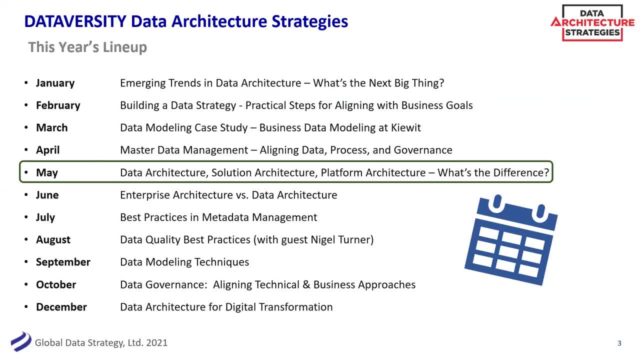 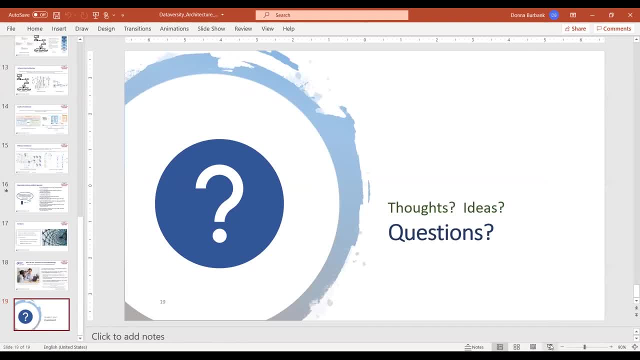 Just a reminder, I will send a follow-up email for this webinar by end of Tuesday. Monday is a US holiday, so it's going to be by end of day Tuesday this time with links to the slides, links to the recording and anything else requested. 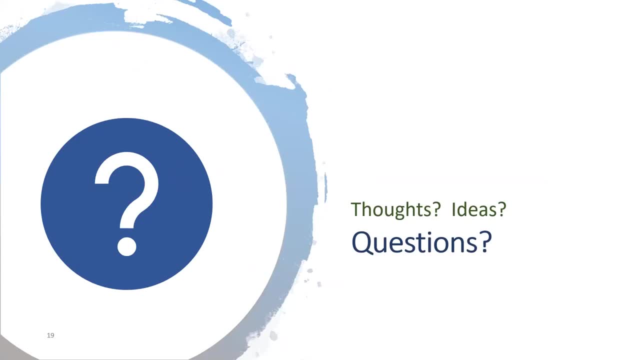 And if you have questions for Donna, feel free to submit them in the Q&A section. And if you see a question that's there already that you wanted to ask, that you were going to type out, I have just hit that little thumbs up arrow so you can just say: hey, you asked the same question. 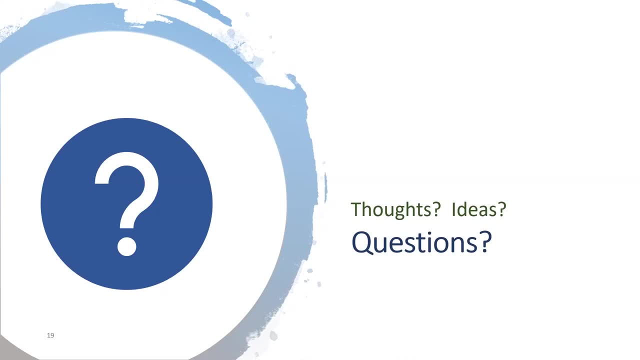 I wanted to know- And it's a very handy little feature there. So diving in here, Donna, these businesses and technical data architecture artifacts haven't changed. They haven't changed very much for a while As we start doing more on the cloud and in quote unquote, modern. 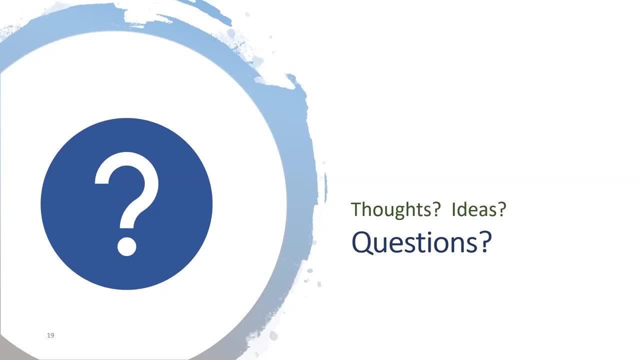 architectures. there's a push to use repositories like MongoDB, where data is stored and unstructured or semi-structured. As a result, many non-data-focused people seem to think we no longer need to model data. How do we justify the need to model in this new world? 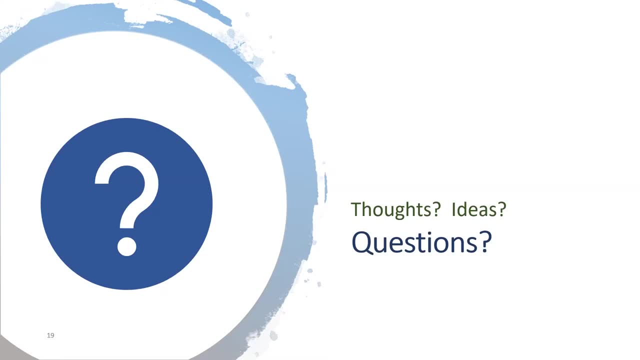 Yeah, no, there's always a data model, whether you have explicitly modeled it or not. right? I like to start with a concept. So I like to start with a conceptual data model or that business layer, because that really fleshes out some of those core business rules. 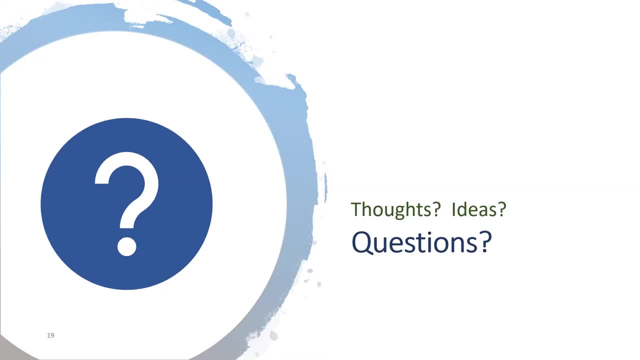 And I have had many a convert from the business of why do we need to model? why are you even discussing customer and you give them an example and they argue with you for another hour about that definition of customer. So I think it's just showing it some of those core. 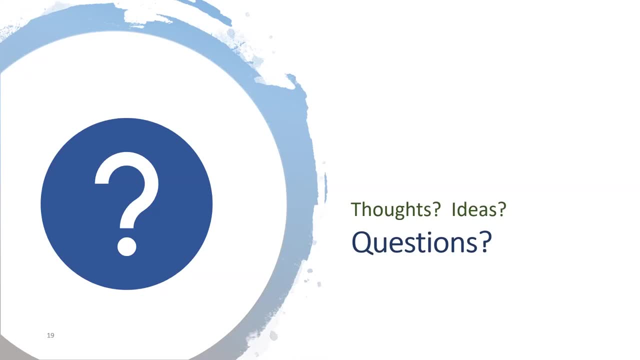 the business should be modeled And then from that, those are your business rules around data, or even a taxonomy, And then from there, then you have to be able to model and model And, yes, you might store it in a document, database or relational. 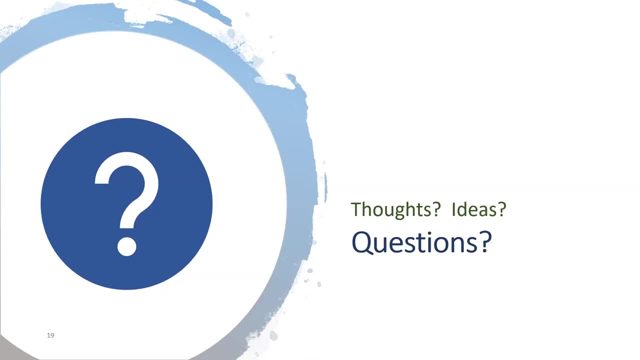 We did show a relational. I think at the logical level that view still shows, because there's still rules: Can a customer have more than one account with the bank, Yes or no? And then, whether I model that some reason, some of those look more relational. 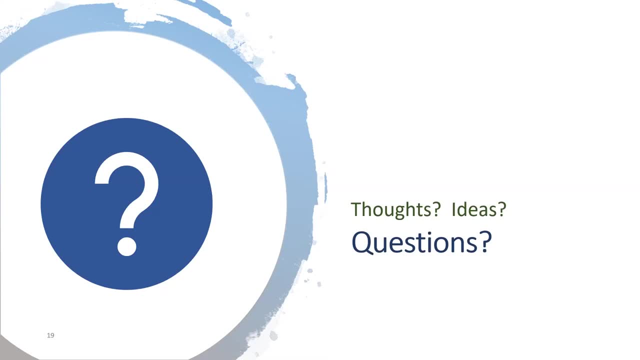 is because they tend to capture those business rules. Maybe I'm doing a key value bearer because I'm trying to have a really performant website. That's just one of the use cases, And some of those technologies don't necessarily need to be as closely modeled. 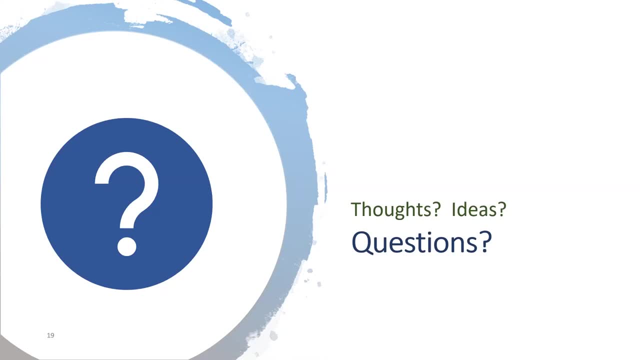 So these were sort of the business models, But I would push back the fact that no model is needed. I had some really bad customer experiences. I mean, I joke about these things of what's the customer? I just the amount of time we're doing a lot of hiring, the number of times. 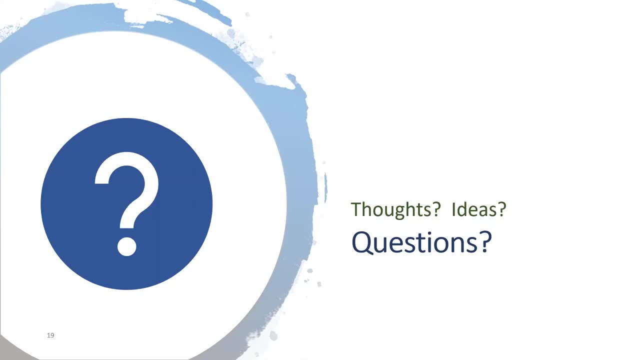 I have signed up for a trying to post to a job board and they advertise it back to me that I just posted it and they're trying to have me apply for my own job to. they have a salesperson Contact me after I've already posted the job. 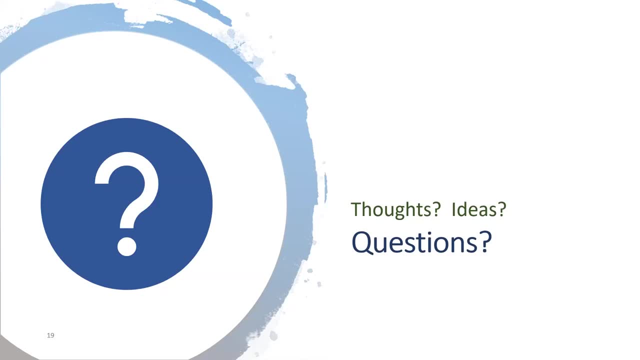 Classic: what's the customer right? And these are all new, They're obligated and they were fast, They were high, performant, all of that, but they missed the core business role. So that's why I think you always need to model. 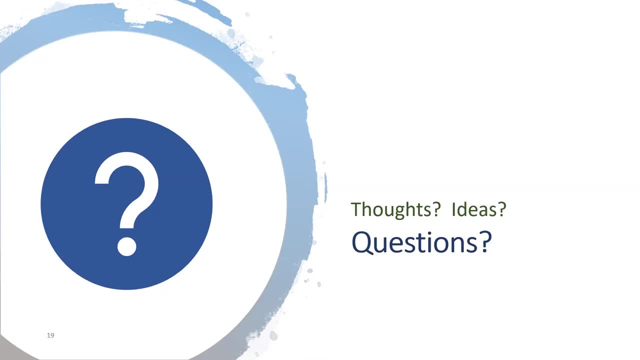 And then you just might have a different display of the model, but there's always a model. So that's my thought. I love it. So do you consider semantic modeling part of data architecture, and where does that fit in? Yes, absolutely. 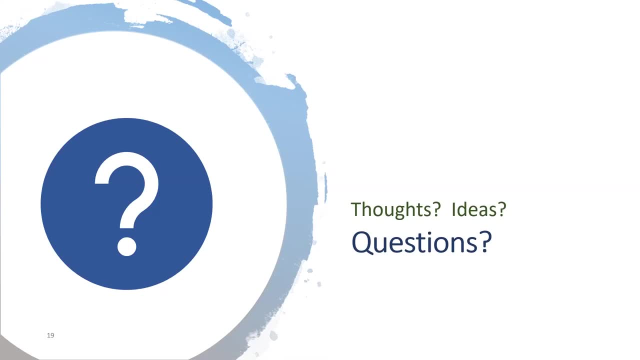 So I would put In that the kind of that business data modeling- I think semantic models are perfect And that kind of see those kind of with a taxonomy, with a glossary, with a conceptual data model on that same kind of category. 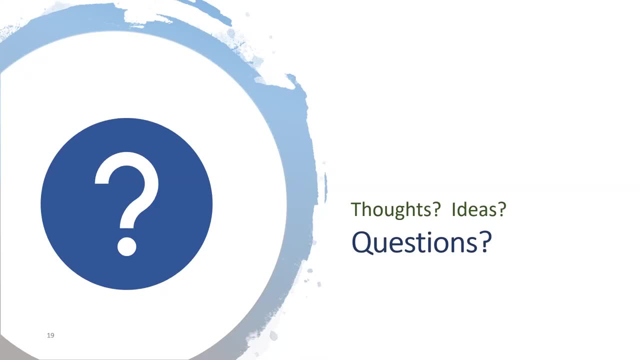 And then if I'm not working with a relational database again, do I still a lot? Do I still use the logical and physical data models? You talked about this a little already, but I think a logical definitely, And it really depends what you're doing. 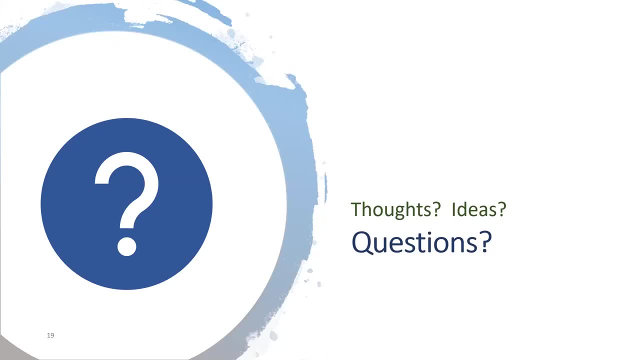 You can be doing XML hierarchical database, a graph database. I think sometimes those are nicely modeled, So I think everything has an inherent model. So maybe not for everything, It really depends on the use case, But I would start with the assumption that you do. 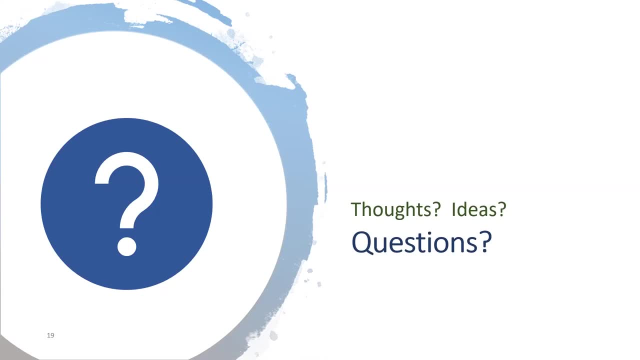 But then definitely start with that logical guess where you get the business rules and then just make sure that the model you're using or the technology you're using is aligning with you know. if nothing else, you know just the data types or the you know. 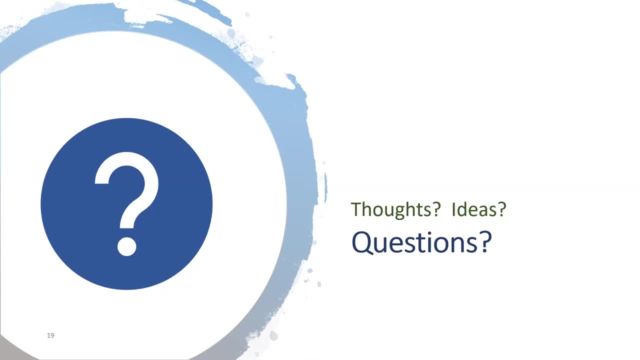 the field definitions of you know, could we just be API or you're passing the customer name back, Do we? do we mean the same thing by the name? You know, everything has a model And I do think, starting with some of those cores and just making sure anything aligns with that, 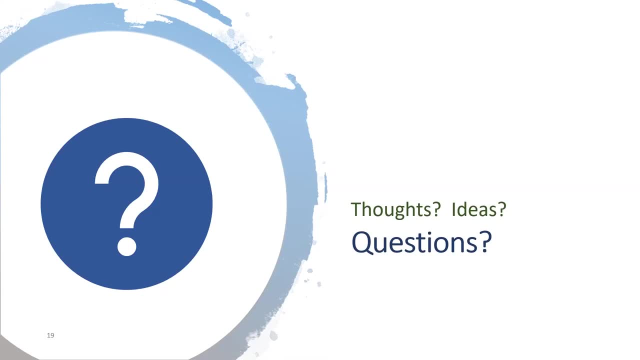 But yeah, you probably don't need a fully attributed data model for everything at the physical level And kind of a part B to that. Donna, you know what about graph databases? How do you? Is there a way to do that? 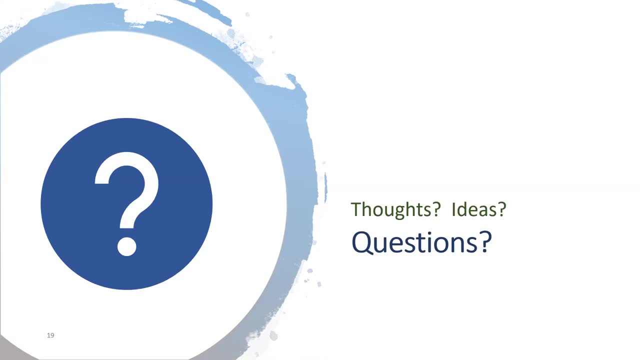 Is data modeling still needed specifically for? Yeah, no, definitely. And that's one of the beauty of graphs, that kind of ties back to that, you know, semantic model question. So one of the beauties of graphs is you can kind of have those different model layers and kind of how those semantic questions put together. 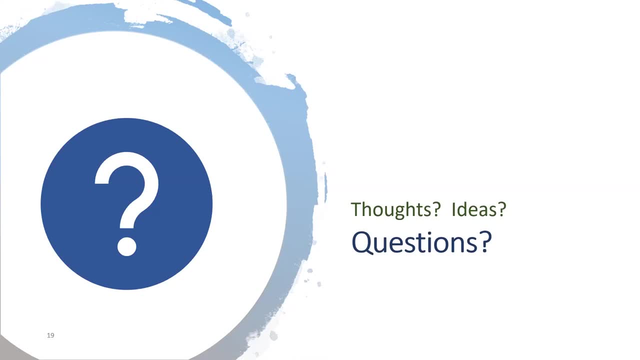 So, absolutely, graphs and data modeling go really well together. It's just slightly different style than the ones I showed, But absolutely that that's one of the powers of graph is that you can kind of have those, those more of a semantic model on top of them. 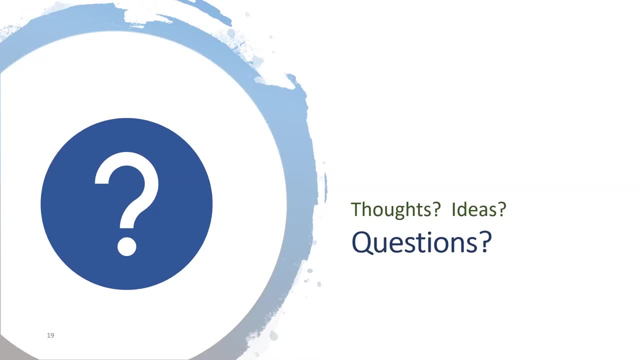 So, yes, Can you address the question of moving data physically versus virtualization or some combo thereof, How much is really needed in real time and what are key issues to weigh and key misconceptions? Yeah, and then we think we did was. I don't lose track of time with it this year. 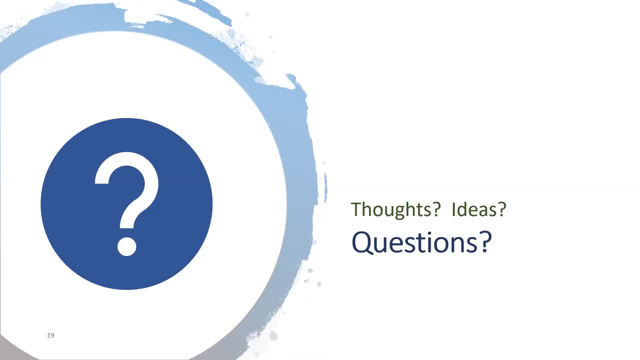 Last year we did have a one of the recorded webinars just on data virtualization. I think that's a classic case of Start with a business name. Why are we doing this? I know it's hot. I know a lot of the technologies have nice user interfaces and some I have one customer that wanted to use it just because they like the user interface and they really didn't have a use case for data virtualization. 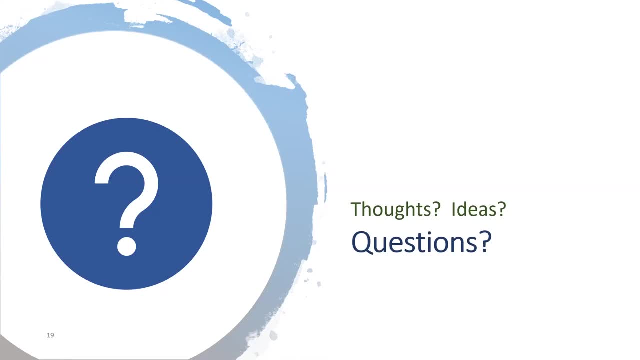 Absolutely Start with these. Having some of these more technical platforms, solution and data models can help you with that decision of whether you need to virtualize. Some of the benefits is that you think the question question or suppose of the question mentioned that you don't have. 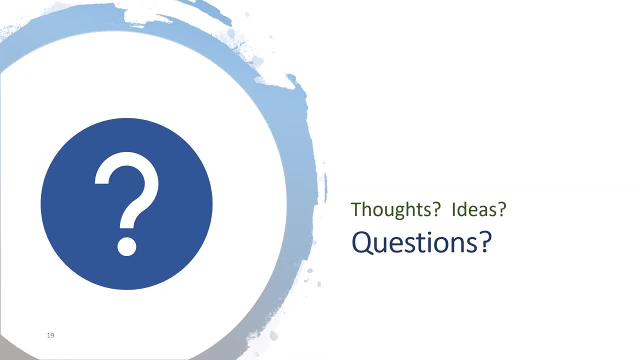 You don't only have to move things, for example, into a central data warehouse to report on it. You can have more of a federated model. You can leave things in place And then just have that virtual layer. so that can be very powerful. You can have a kind of a common reporting layer across multiple technologies. that can be really powerful. 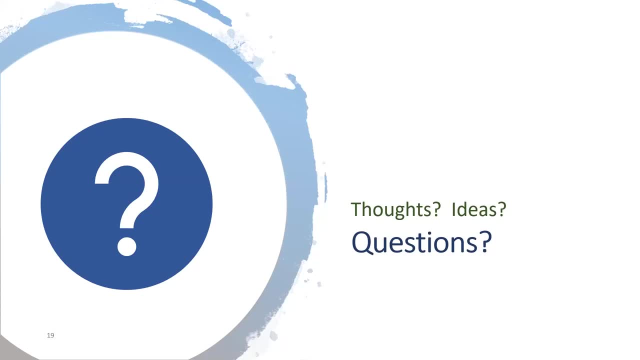 So you know, especially, you can use it for everything in production. I do have some people using it kind of almost in that exploration: before I move things, Let's kind of virtually integrate things and see, you know, do we absolutely have to have it in a single data warehouse? 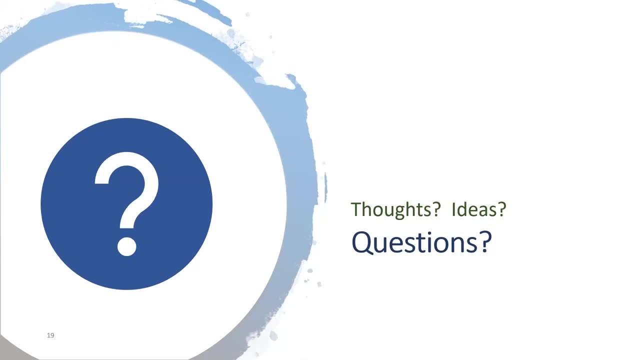 I think the caution of that is some people or some organizations use days of virtualization as kind of, you know, duct tape over the structural problem. You have to- almost more so I think- model out what data is where, how it's integrated, what it means, what the security levels are. 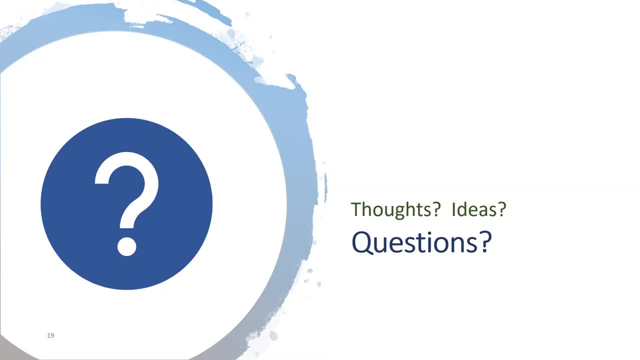 So I would argue, in some ways you need to have even a better architecture to make virtualization work, Because you need to understand the systems, But the benefits, the ones I mentioned. if you absolutely know the pattern, one org we used did it really well. 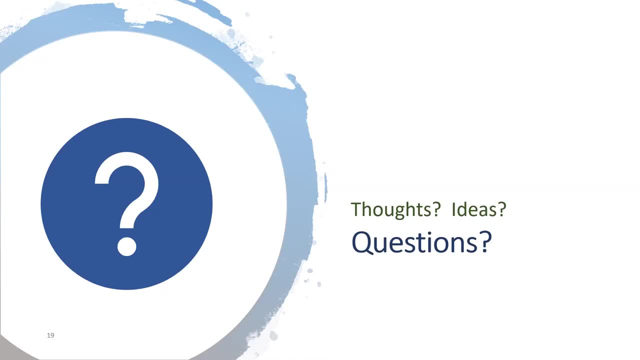 It was a university like what do you call it? consortia, where they were able to share data in terms of they understood the structures, But there was no way they were going to move the data between the different universities, So they did have a virtualization layer. 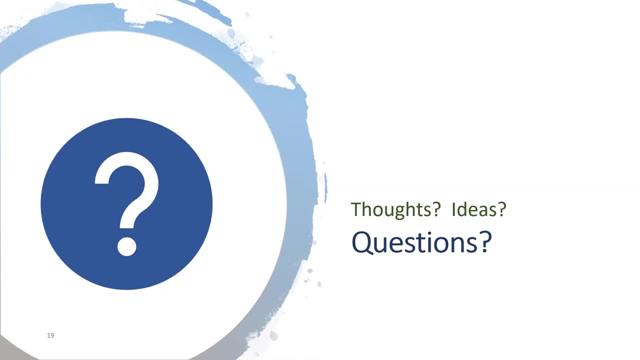 And that was a really good example of, yes, it was well modeled and understood And, yes, it was virtualized. You know, some people don't model it so much and use the virtualization as a test case. But what I would say, don't do is just virtualize so you don't have to do the hard work. 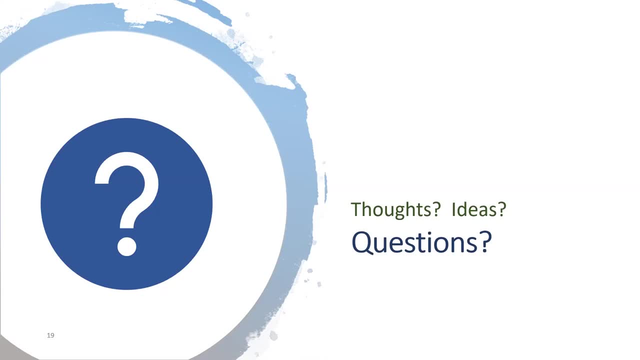 So hopefully that answered the question Absolutely. Thank you. So in which architecture will you define data pipeline patterns? I would say some of the data pipeline patterns are getting more into that bottom kind of that platform architecture. I mean, there's a bit of a data flow diagram on top of that. 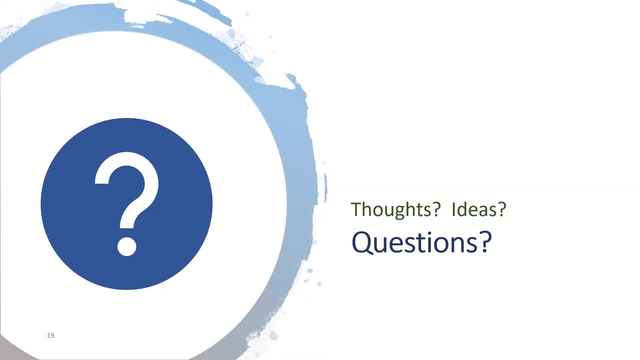 You do kind of have that logical architecture, But I'm thinking that's more of your kind, of your platform of how are we moving it, what do those pipelines look like, what's the timing of it? And, Donna, can you give some more examples of taxonomy? 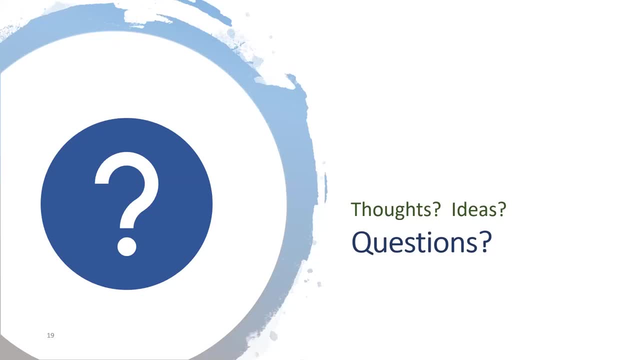 I have seen a taxonomy in I sometimes different categories that the different one organization was doing a lot of market research and they had their own taxonomy of these are: These are consumer packaged goods and these are health care products or kind of the different ways of looking at it. 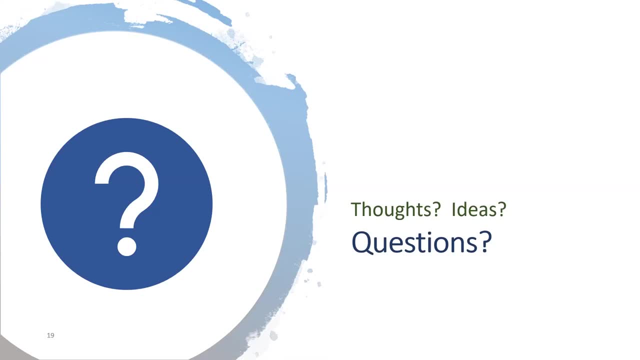 Some organizations use taxonomies kind of to organize their products. These are lifestyle products and these are sportswear products and things like that. Part numbers And things like that can kind of have their own And it's almost like a hierarchy of where they're all part numbers. 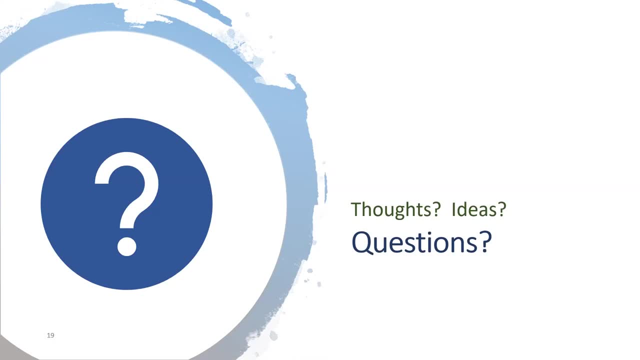 Right, But we kind of have a part number taxonomy that really kind of organize them might be another way to look at it. So those are some common ones that I've seen in terms of a taxonomy- I mean the classic one I had in biology. 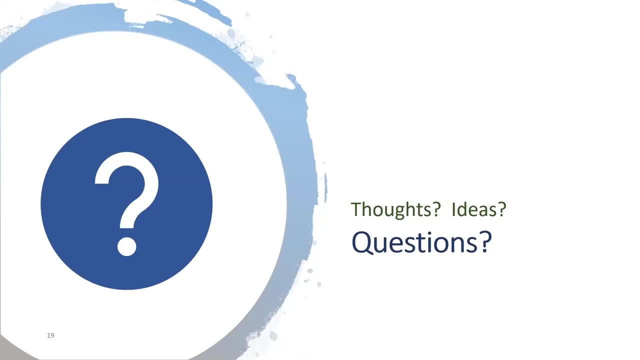 Right, You kind of had a taxonomy of the different species and things like that, But it is sort of like a category. They're all categories But you kind of have a taxonomy within them that add that structure in terms of the content. That makes sense. 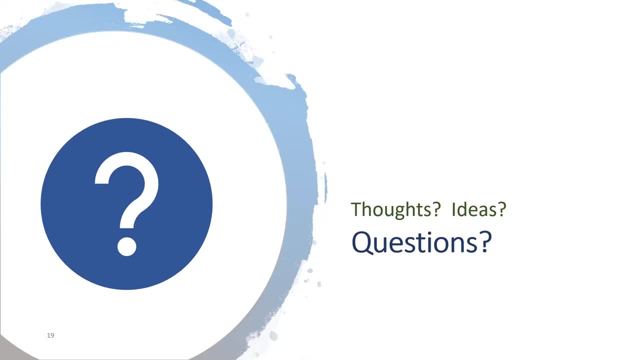 Probably explain that really badly, but hopefully that explains Well. if the questioner has additional insight that they would like, feel free to submit it in the Q&A. Well, I'll get to that. So, Donna, my current case: designing the new enterprise IT strategy with the first time ever, integrating data architecture into the well-established disciplines as application and technology architecture. 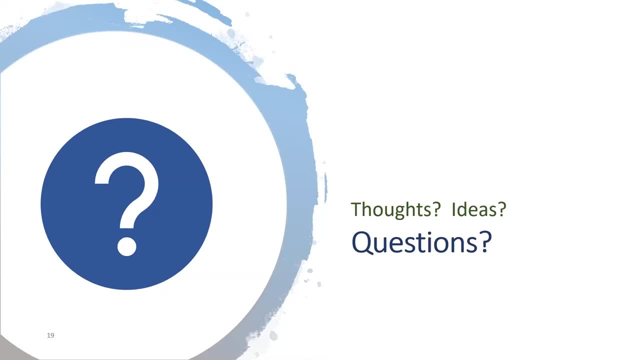 The old stuff is straightforward, as is to be, as is to be to gap, but how to address and integrate data architecture first time is such an established process. So, if I think I'm understanding that correctly, everything else in the organization is well modeled and well established, but the data maybe wasn't. 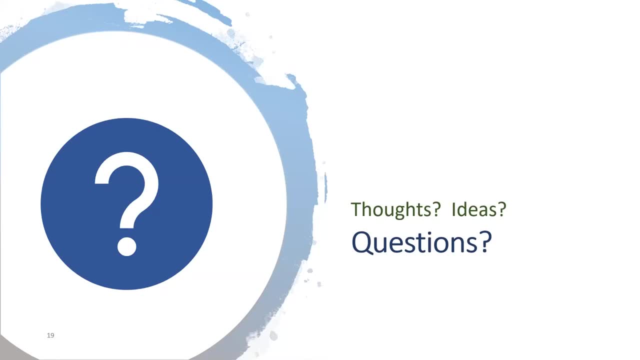 I think that's how I'm reading it. I would. I would hopefully the other areas- I guess I'm just thinking aloud here- If the other areas are well documented already, I might take those diagrams and kind of add a data layer. 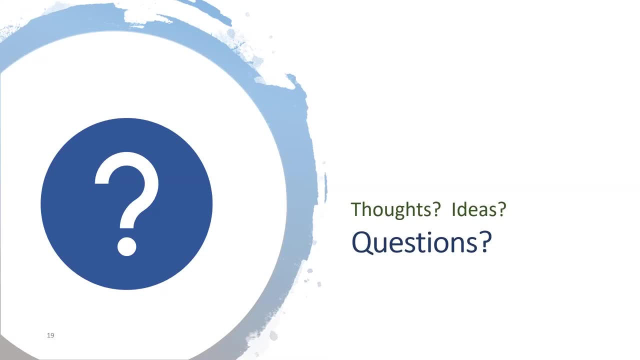 Again, this is probably not an official diagram of those ones I mentioned, but added data later on top of those. I think a big starting again with kind of that high level of what data we need to focus and then having some kind of use cases. 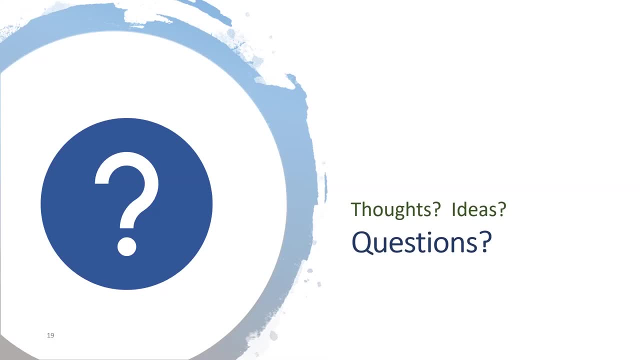 So say, it's customer data. Now, how would customer data go through this architecture that you have? Maybe that's a good question, Maybe it's more like a data flow, but it would show the integration of. you know, maybe these are the applications you've already all integrated. 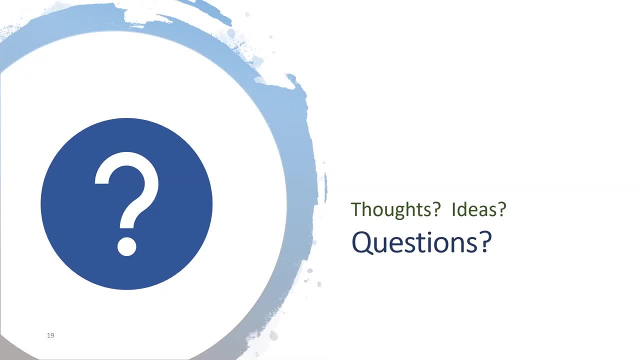 That's great, But now how would a customer address go through from the CRM to the you know shipping or to whatever else they have? Maybe that's to kind of tell that data story of how data flow, how it's structured and how it flows and then maybe how that would affect the platform decisions. 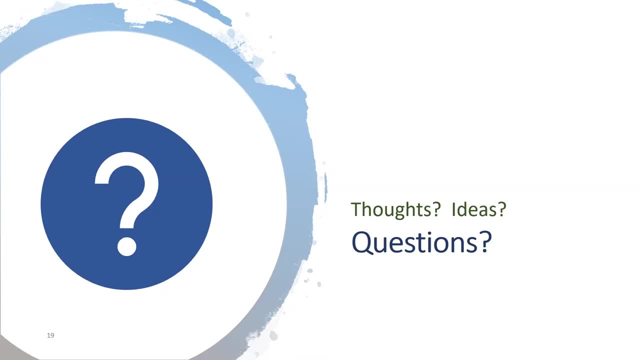 So therefore we have to do X as a data architecture to support the architecture that exists. That is my off-the-cuff way of how I might approach it, but without more details can't get more specific. but hopefully that helped. Makes sense. 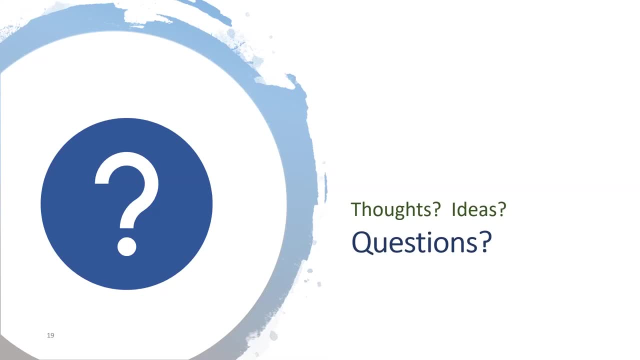 All right, I think we have time for a couple more questions, at least one more. So any suggestion of good? or excuse me, let me just kind of check through here. Layered data modeling to link individual data models in different architectural domains. 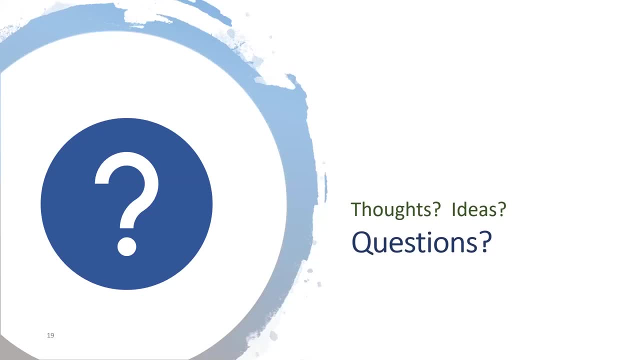 I'm sorry, Could you say that again? Yeah, So is there layered data modeling? is it to link individual data models in different architectural domains? A lot of the enterprise architecture at a high level, a lot of the enterprise architecture tools kind of have that layering. 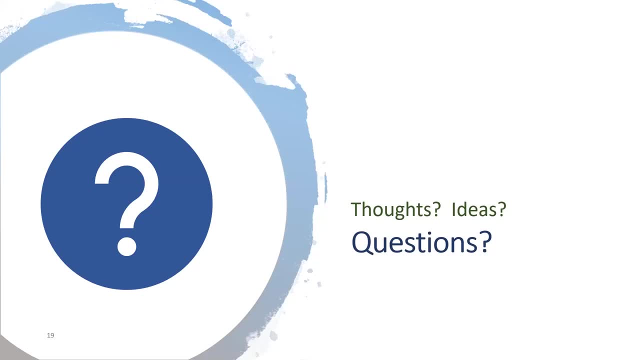 They tend to be. you know, here's my data model, here's my process model, and then they can sometimes share some of those artifacts across. Those can also be very expensive And it takes a bit of rigor to do that. I'm also a fan of even just things like a Visio, or maybe it kind of ties back to my previous question. 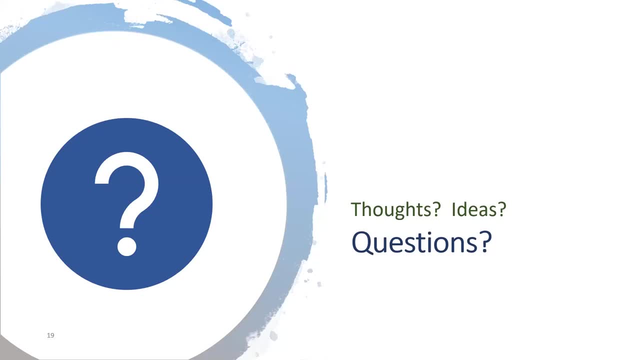 I often get a little more flexible with the design if it tells the story. So, for example, I'll do a process model and then just not too far off from BPMN, but, like you just put, here's where the data lives, All right. 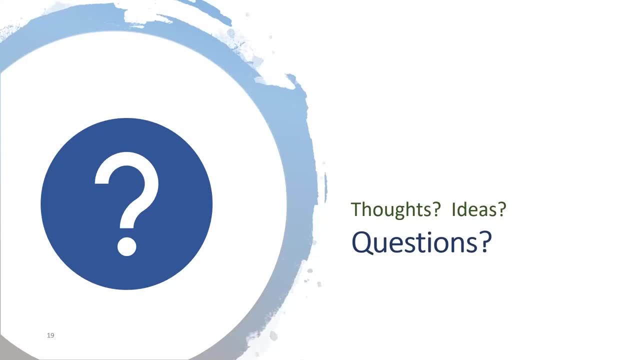 Or you kind of adding a data layer literally on top of the diagram with a picture or a graphic, And then the data modeling tools are going more of the enterprise architecture route, so that they can take their data model artifacts and then kind of show them on the diagram. 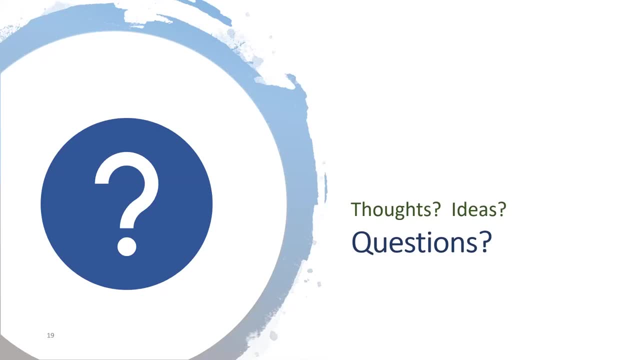 I mean that makes a lot of sense. But I think it's more of that enterprise architecture that seems to do it. And you know, almost on the other end, sometimes good old Visio can kind of you can mix and match different modeling paradigms and kind of show it that way. 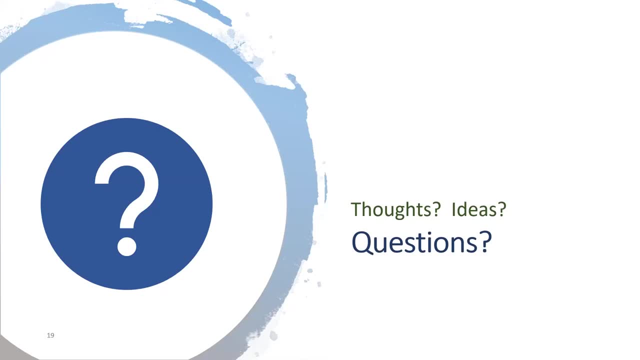 Those are probably two extremes. Anything else, Well, I think we you left just enough. Okay, Enough time for one more question here, An elevator pitch. I understand the value and the components as a data architect, but how have you had success explaining things to the executive leadership? 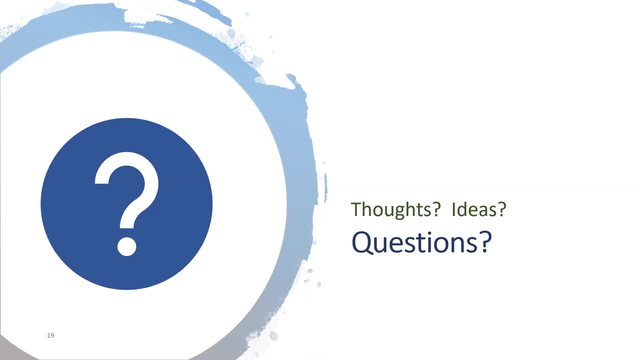 Um, I generally so for each of these, and I, when I went into the data layers, I kind of talked a lot about the conceptual, logical, physical. I think that can also hold true. Yeah, I think so. I mean, and I think that's a pretty good question. 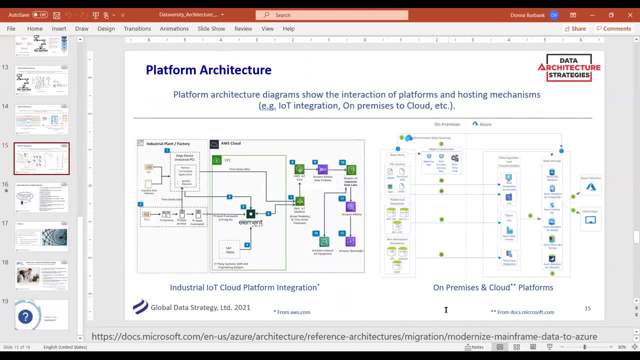 So I would say that a lot of this is it's kind of. you know, I'm a big fan of the technical, the technical part, but I think there's a lot of the technical stuff that can happen in the data center as well. 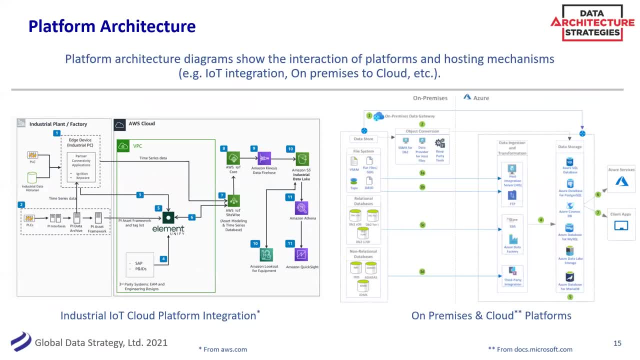 I think there's a lot of, you know, for any of the layers. As you know, I'm a big fan of storytelling, So part of it is how you tell this story. but I have so dying Actually. for firstly, I think a lot of the tools vendors these types of even platform diagrams just look prettier.